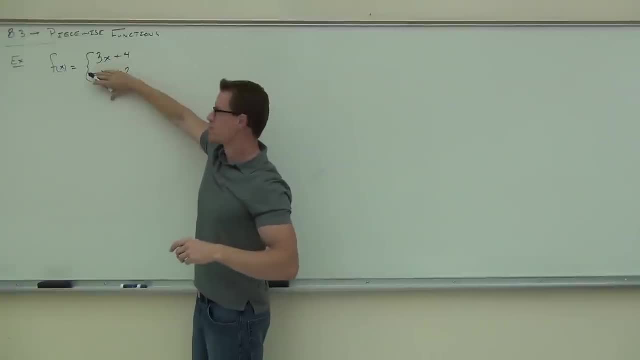 you draw your line, You all with me on this. This is a very much review for us. If I ignored this one, could you graph that? Say, yes, What's your y-intercept, What's your slope? You'd go down one along one after going up two on the y-axis. 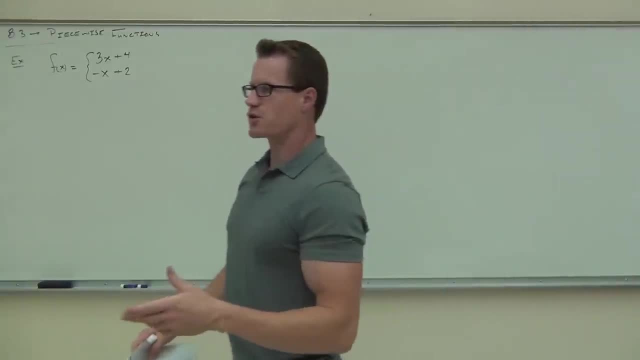 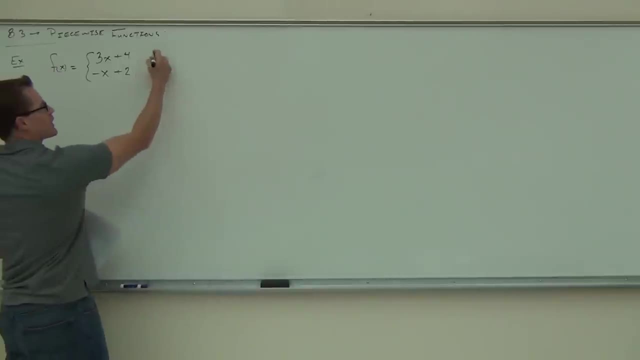 So we could graph each of those things. now, When you're talking about a piecewise function, we put those two ideas together, but we do it with some directions. So what I mean by after each function, you're going to have a comma and it's going to tell you when you 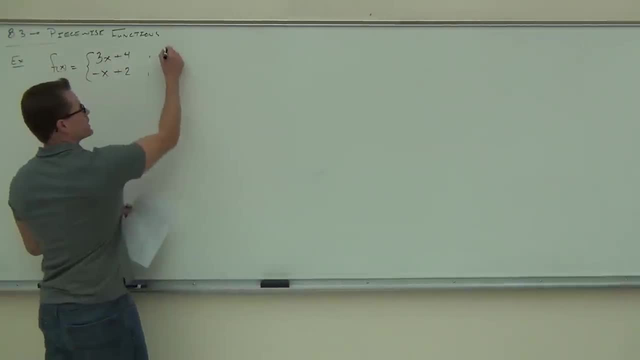 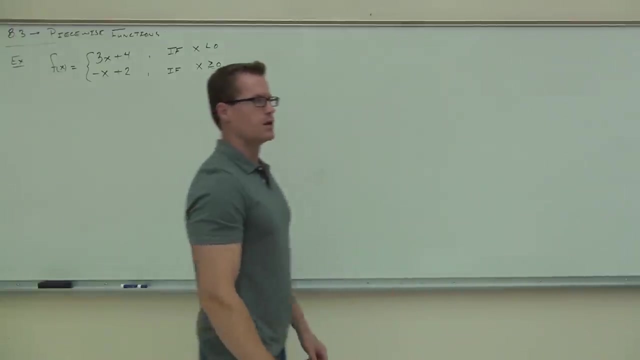 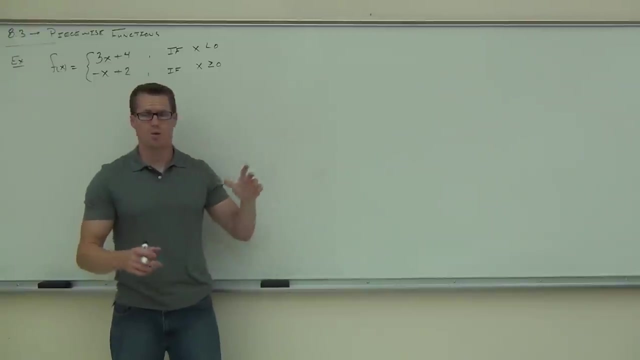 use this little piece of your function. So in our case it'll say: if x is less than zero, if x is greater than or equal to zero, You're always going to have the situation where you have less than and greater than something. It doesn't necessarily have to be zero, it could be three, or negative two, it could be. 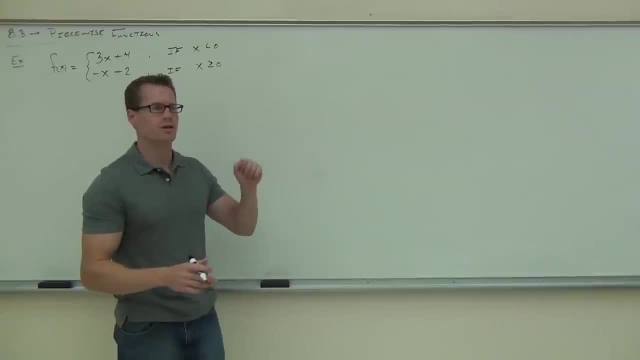 whatever's up there. In our case it happens to be zero. Also, one more thing to notice: Do you see how one of these has the equals and one of them doesn't? That has to be the case. They can't both have equals, otherwise you wouldn't have a function because you have. 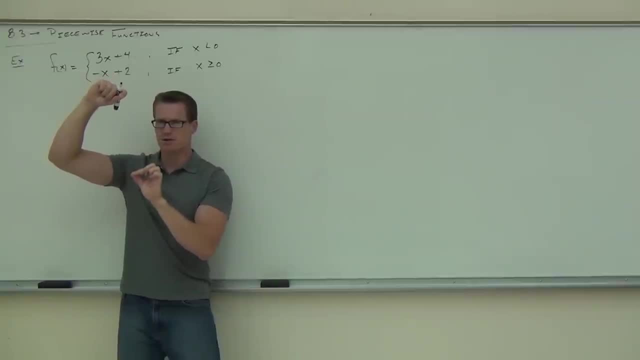 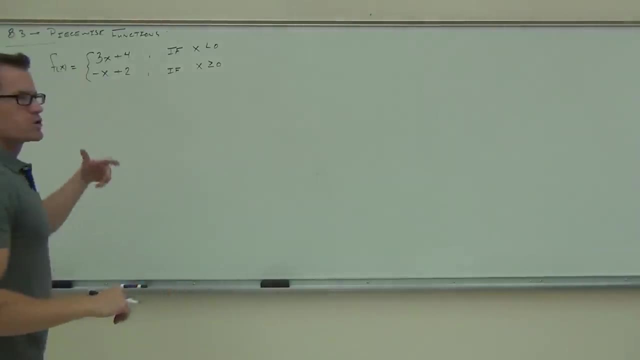 two points for one spot. Does that make sense to you? So you've got to have a less than or a greater than, strictly in some case. So how do we accomplish plugging points in then, if we have two functions? Well, this tells you what to do. 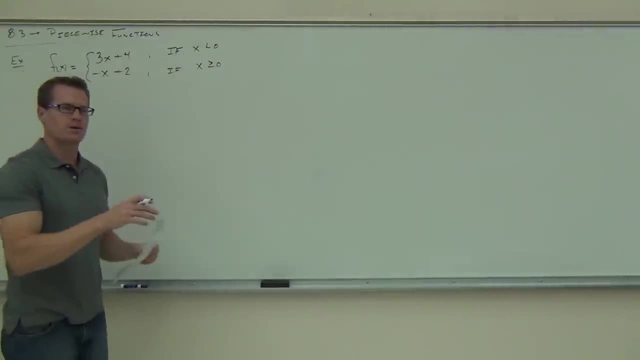 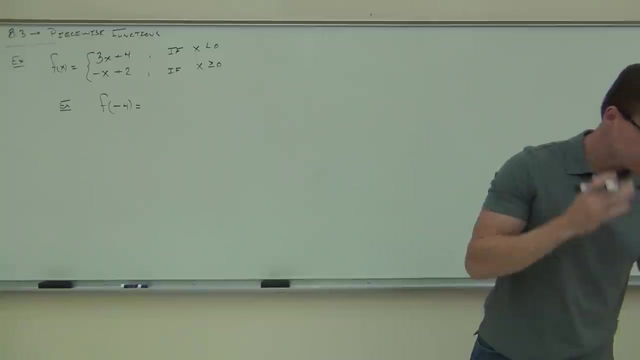 Let me give you an example about how we go about finding out how to evaluate these things. So, for instance, let's say I asked you to find f of negative four. So if I'm trying to find f of negative four, of course f says we're looking for the function. 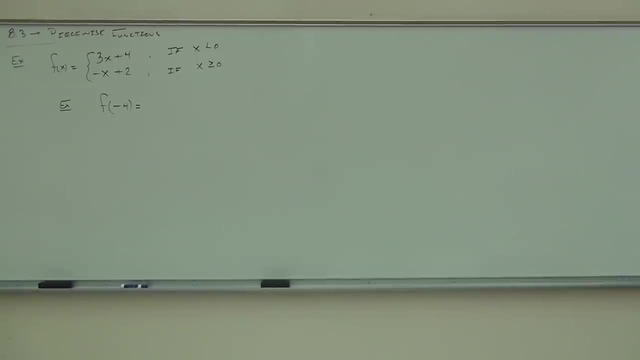 f. What's negative. four say to do. What's negative. four say to do. Well, which one do I plug it into? That's the question. So when we look up here, it says f of x. we want f of negative four. 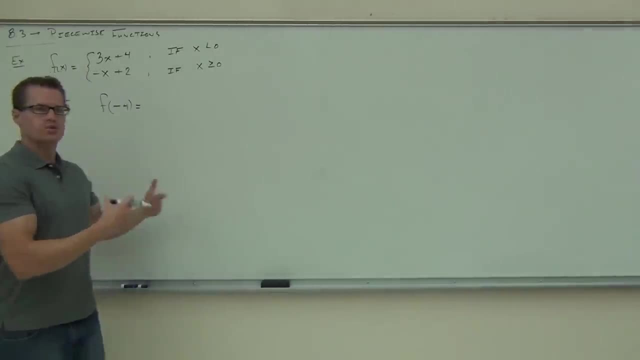 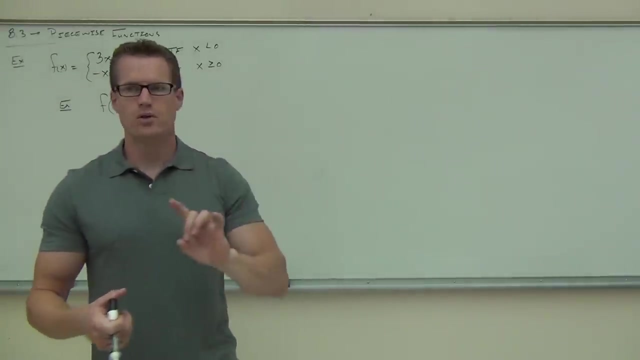 F of negative four means plug negative four into my function. but which one do I use? Do I use this one or this one, or do I use both of them? What do you think If I use both of them? listen carefully: If I use both of them, you're going to get two points for one input. 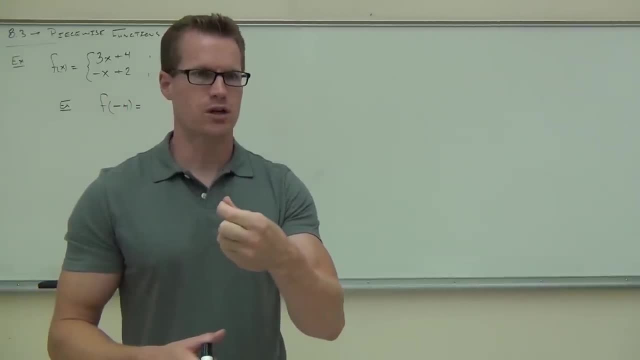 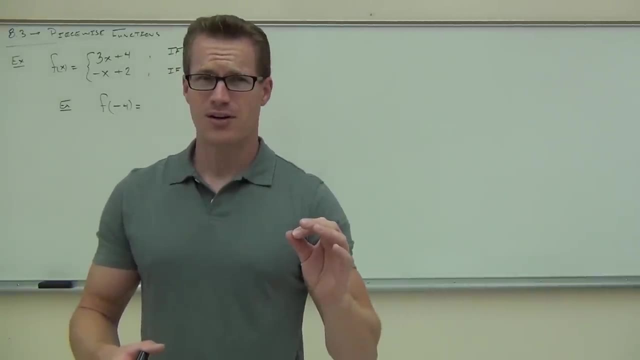 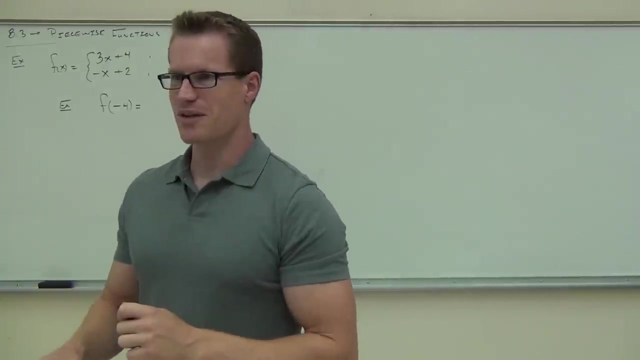 Does that make sense? You cannot have that. It won't be a function. So let me make this very clear to you: You never, ever, ever, ever, ever, ever plug one point into both expressions. Are you clear on that? 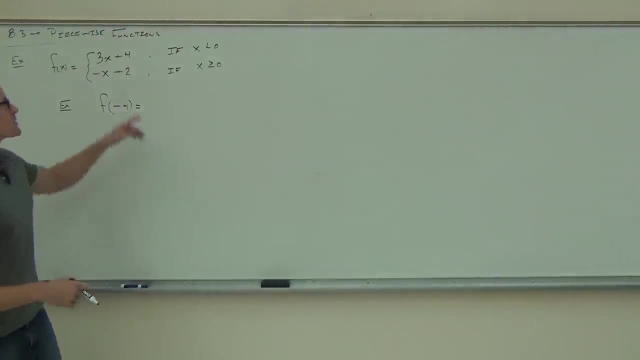 Ever. It's either one or the other. Now this should tell you what to do. This says we're going to use the top one if x is less than zero. It says we're going to use the bottom one if x is more than zero. 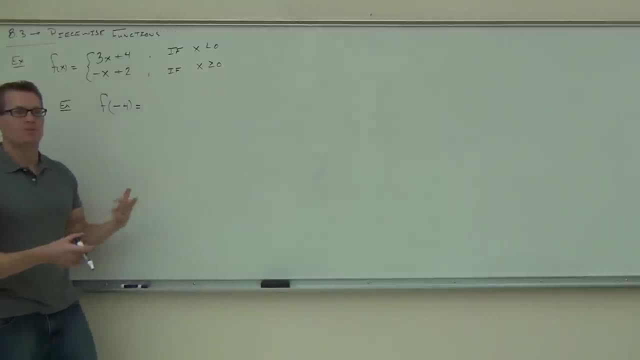 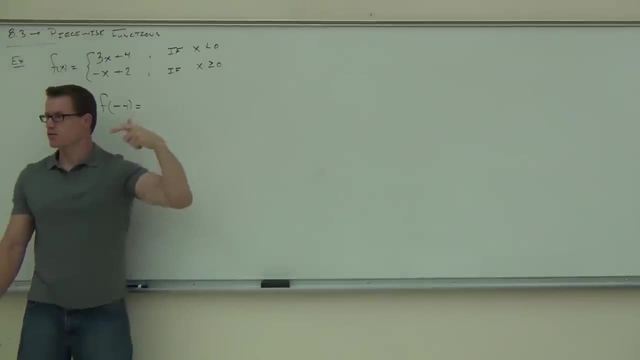 Less than zero, Then how are we going to use the bottom one if it's not greater than zero? Does that make sense to you? So you just find out where this fits. It's either going to be the top one or the bottom one. 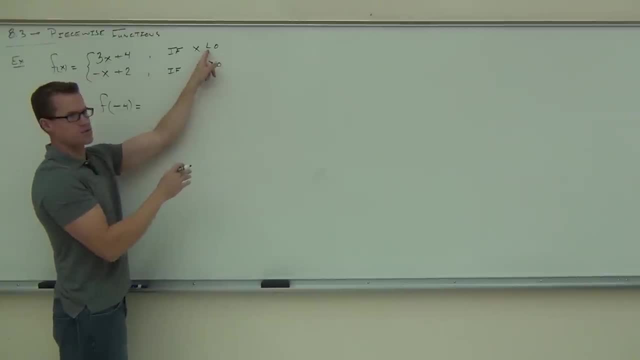 It's never going to be both. That's why you don't have an equals here. even if I told you about zero right, It'll only fit in one of these things. Does that make sense? So, whatever we have here, you're going to plug into either the top one or the bottom. 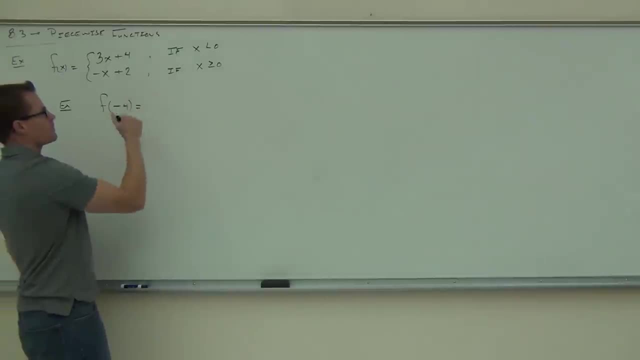 one. We look at our x value, It says negative four. We're going to use the top. So we just say, okay, three times negative four plus four Again. why don't we use the bottom expression? So this only works if x is bigger than zero. 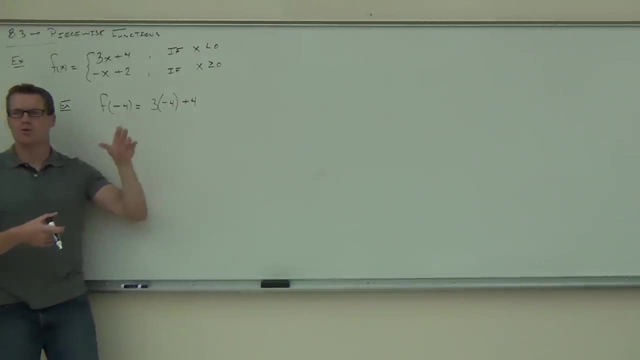 This works if x is less than zero, Since, in our case, we're plugging in negative four, that happens to be less than zero. That's the one we're going to use, And then we evaluate, like we normally would: How much are we going to get out of this thing? 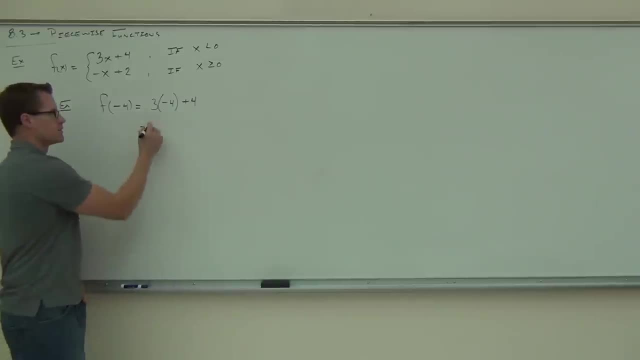 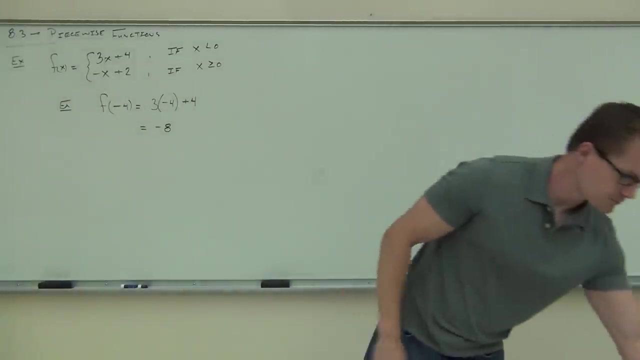 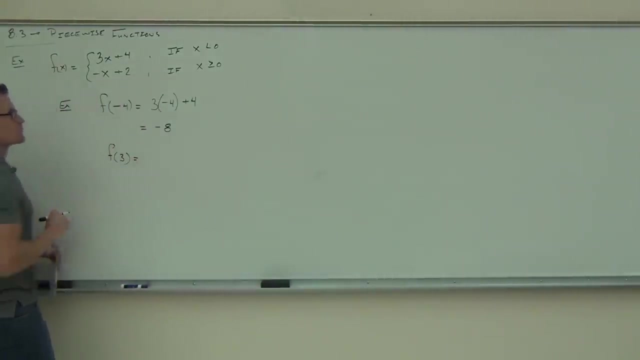 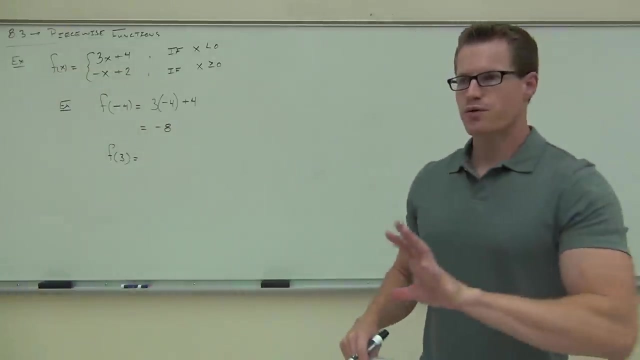 Eight. Negative eight. Negative eight. okay, So we get negative eight out of that. How about f of three? Let's talk about that one real quick F of three. In this case, it says: you go into your function, f. 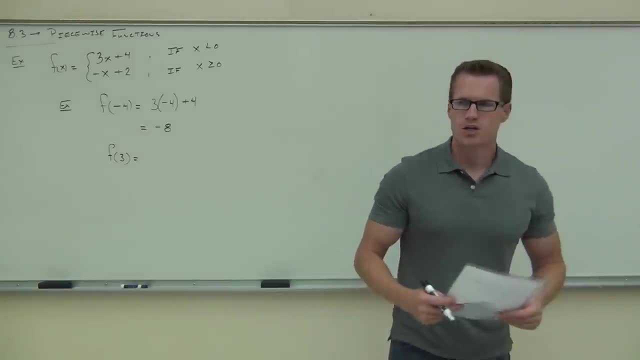 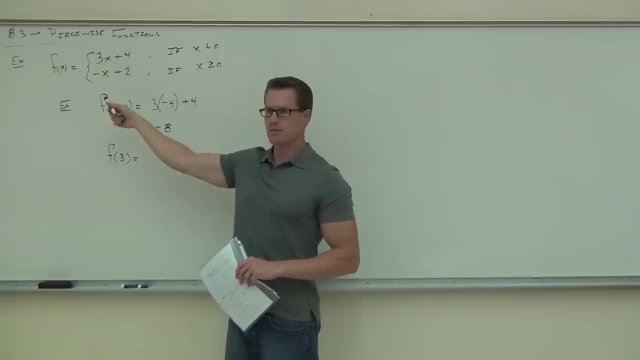 You're going to plug in the number three. So in our case, x is three. Should we be using the top, the bottom or both of these? Y? Y Because it's bigger than zero, Okay, great. So this says, if x is less than zero, we use the top one. 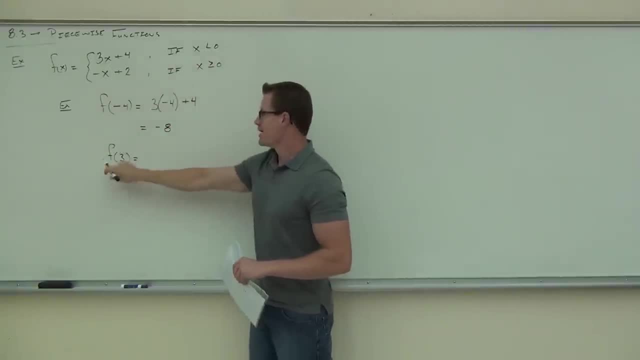 Three is not less than zero. right, Three is positive. Three is greater than zero. Yeah, that's what we want, That's the one that says to use. So we're going to be using the bottom one, and only the bottom one. 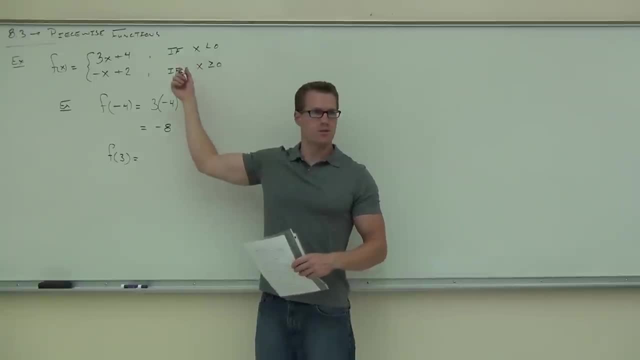 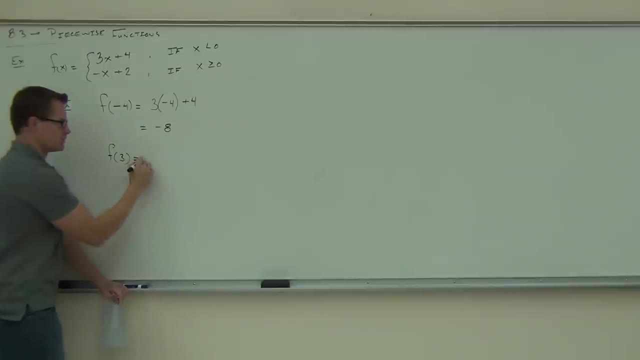 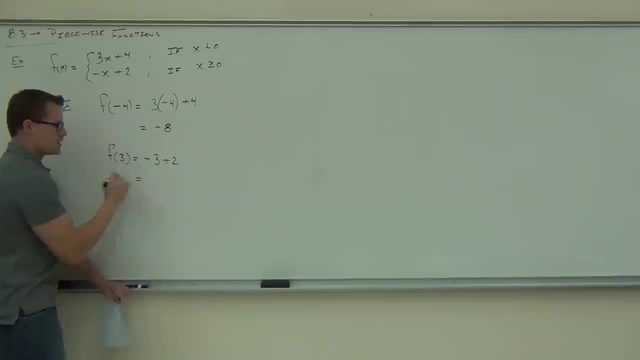 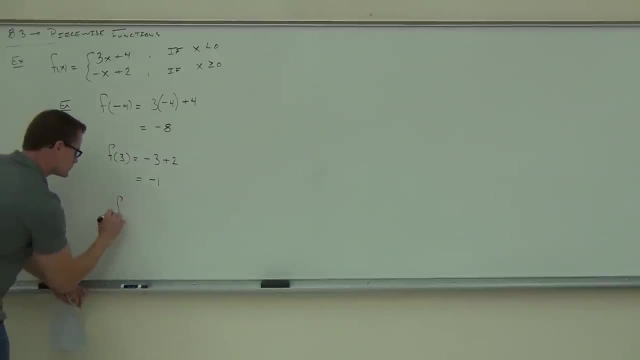 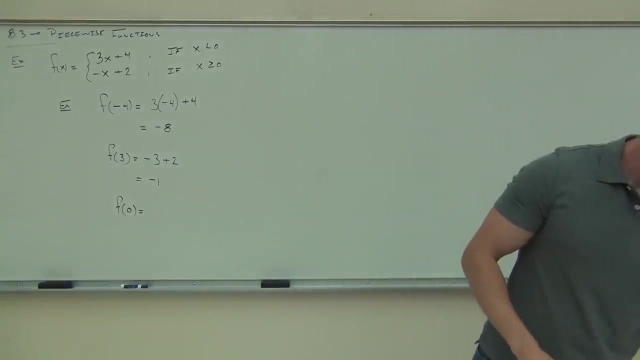 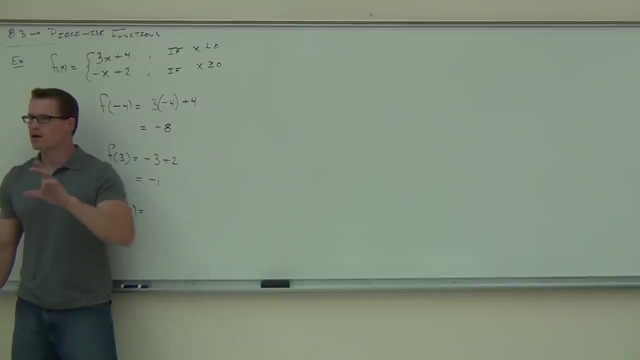 We've got negative one. Is it okay to plug in zero? Yeah, Is it going to be plugged into both of these functions, do you think? No, Not bottom one. Okay, so we know the inequalities have that greater than greater than equal to less. 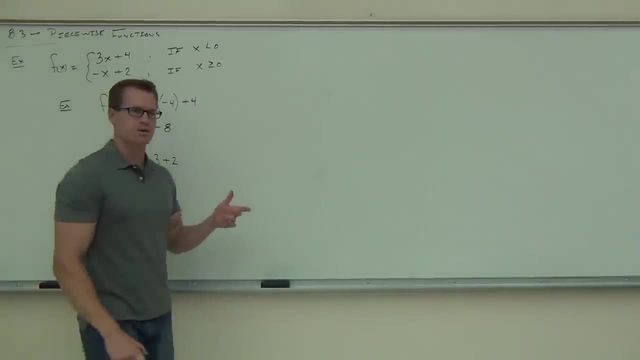 than less than equal to Equal to zero. that's the one we're going to want to plug this into, because we have the actual value of zero. So here, since it's not equal to zero, we can't use the top one. 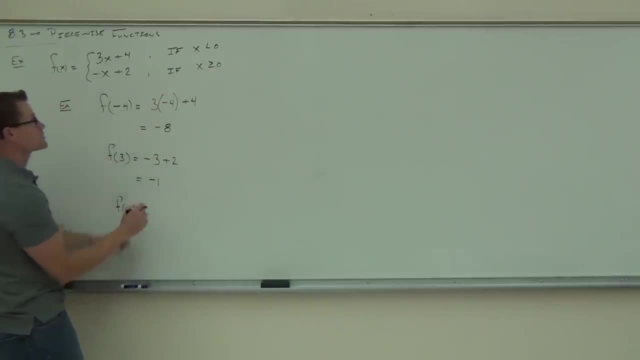 Here it is equal to zero. We are going to use that. So we're going to use negative zero plus two, Negative zero plus two. of course that negative zero does not do anything for us. We get just two. Of course you're going to feel okay plugging these numbers into our functions. 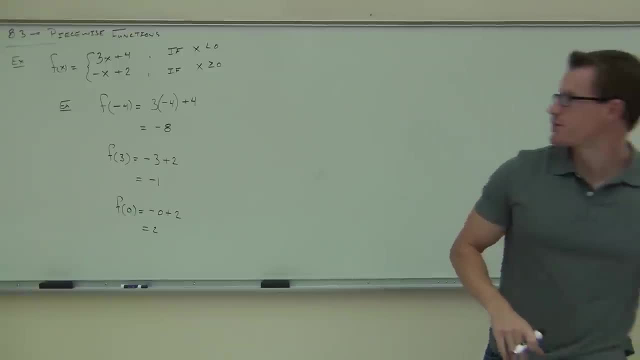 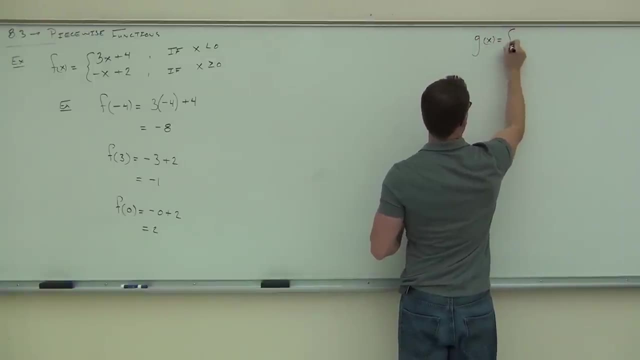 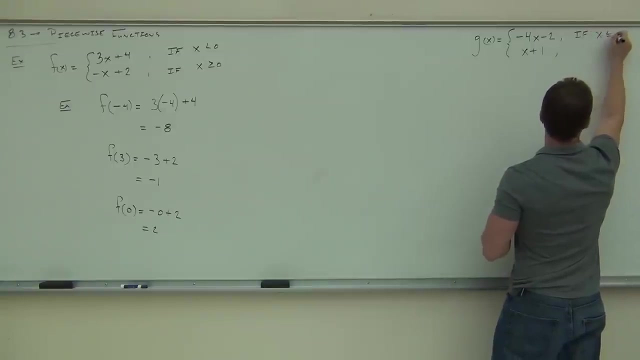 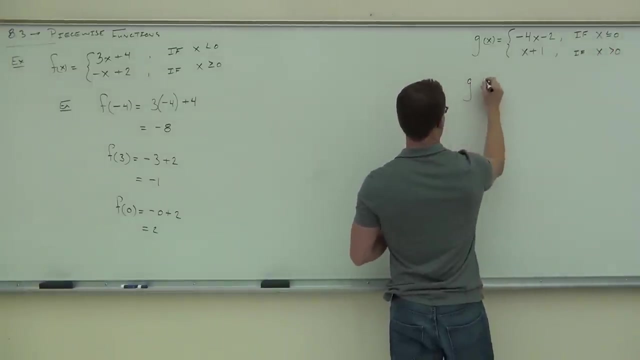 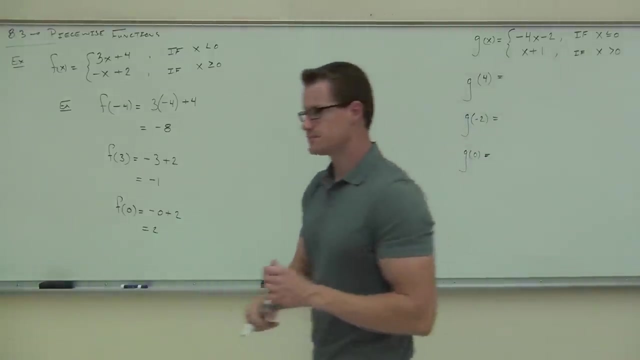 Good, Why don't you try one on your own, and then I'll show you how to graph these. Okay, there you go. Take each of those numbers, Plug them into the appropriate function and see what you get. Okay, so we're going to plug them into the appropriate function and see what you get. 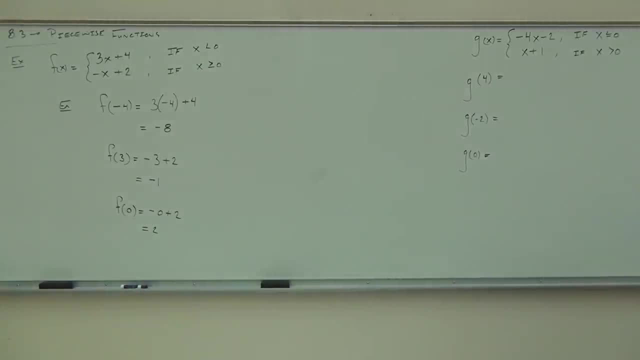 Okay, Okay, All right, There we go. Let's see where these guys fit. No, I told you we never, ever, ever plug one number into both functions, because otherwise you'd have something that really isn't truly a function. What has to happen on g of x is you plug in one number, you get out one number. 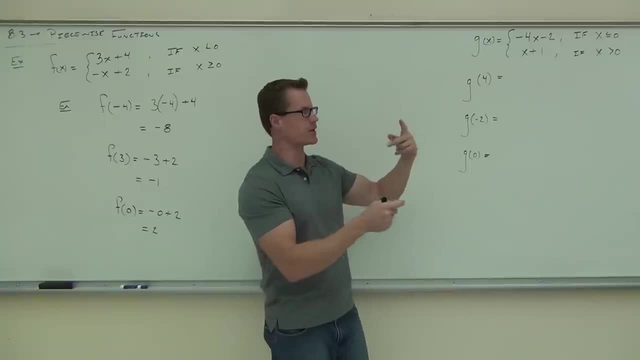 You can't plug in one number and get out two numbers. That means you don't have a function out of this thing. So we needed these directions to make sure we're doing this correctly, make sure we're getting out one point, one value for every value we plug in. 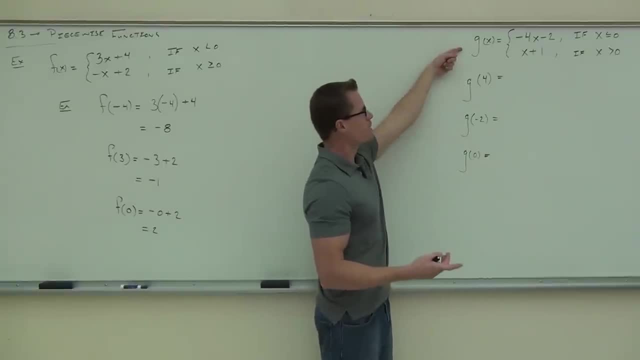 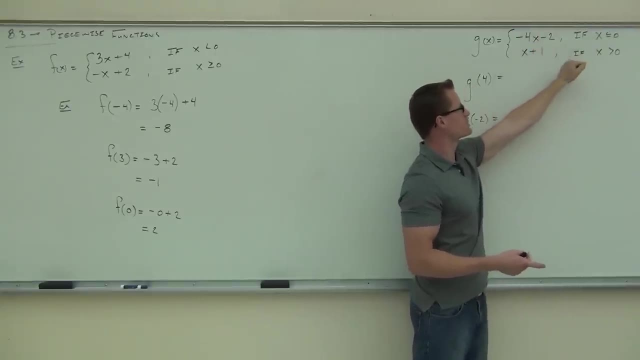 So when we look at g of four, it says: you're going to look at g, that's g. you're going to use your directions to plug four into the correct spot. So we use our top function or our top expression. if x is less than or equal to zero, we use 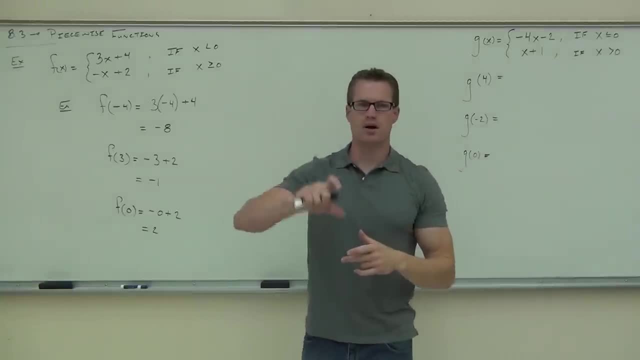 the bottom one if x is more than zero. In this case, we're going to use the top one or the bottom one. Bottom one, Definitely the bottom one. We had four. four is greater than zero, so we're using the bottom expression. 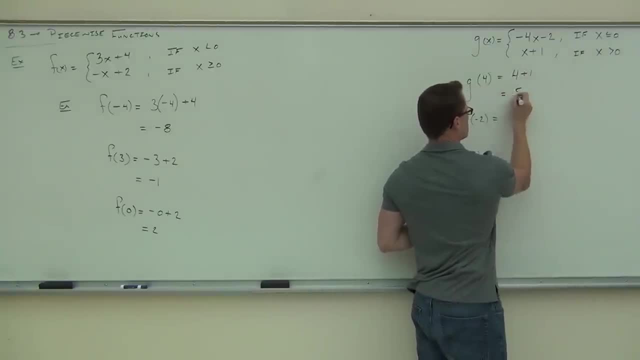 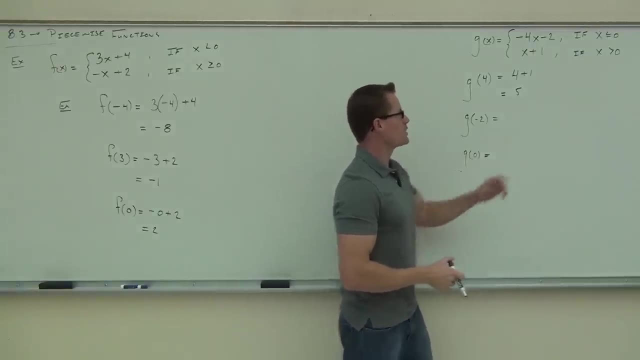 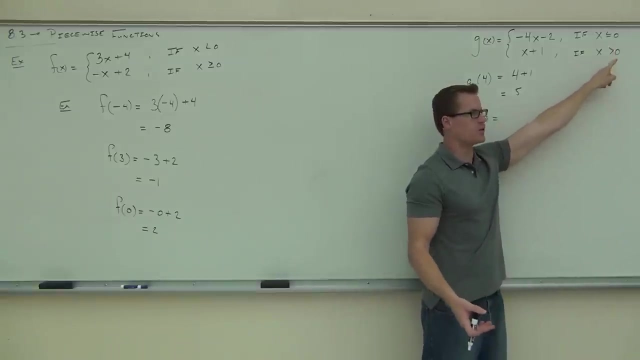 And we get five out of that, raise your hand. if you got five, Good for you. Okay, next one: negative two. Are we still going to be using the bottom expression for negative two? No, No, that wouldn't make sense, because negative two is not greater than zero. 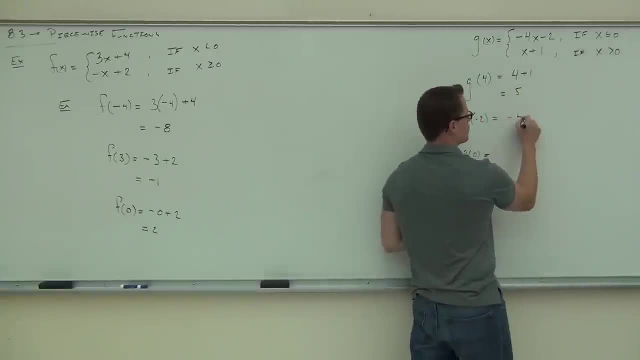 Negative two is less than or equal to zero, so we use our top expression negative four times negative two minus two. and what do we get out of that, folks? Six? Sure, because we have a positive eight minus two. that's going to give us six. 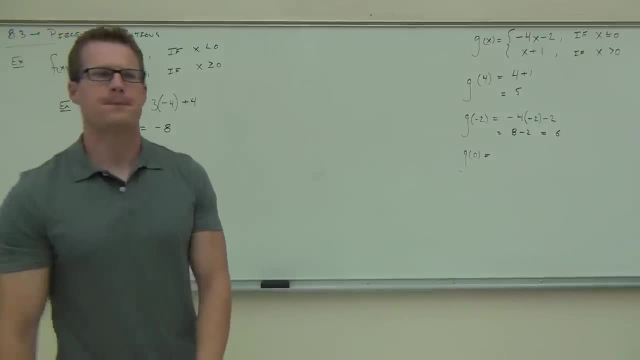 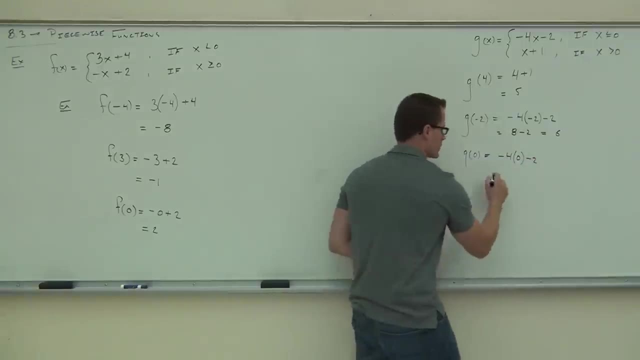 And lastly, zero. where does zero fit? Top one, bottom one, Top one, Yeah, definitely, because that's where our equal's at. So negative four times zero minus two, So we get negative two out of that. Are you guys with me on this one? 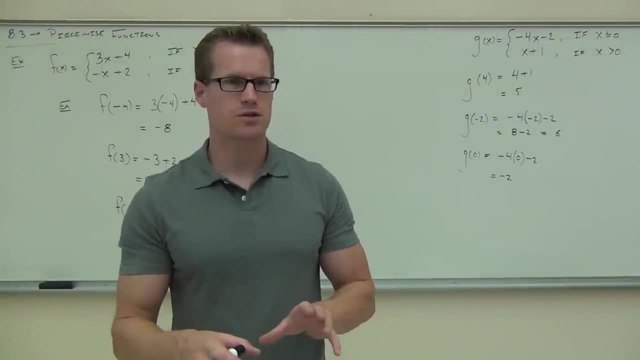 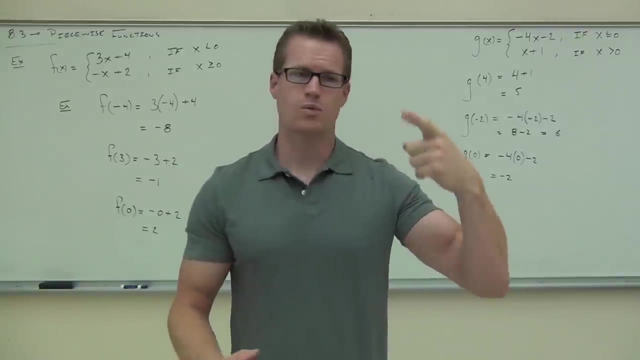 Do you understand how to plug the numbers into our piecewise functions? Just look where it fits. according to our directions off to the right-hand side. We use how many? Both or just one One, Just one. It's got to fit somewhere. 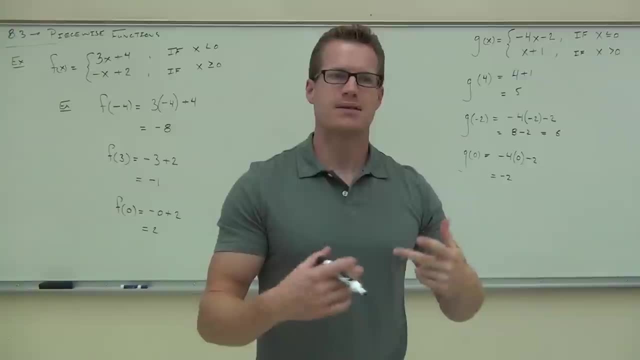 It will fit somewhere. It doesn't ever fit in both of them. okay, That's going to tell me I'm going to give you a problem like this on the test. It's going to be very easy if you know what you're doing, right. 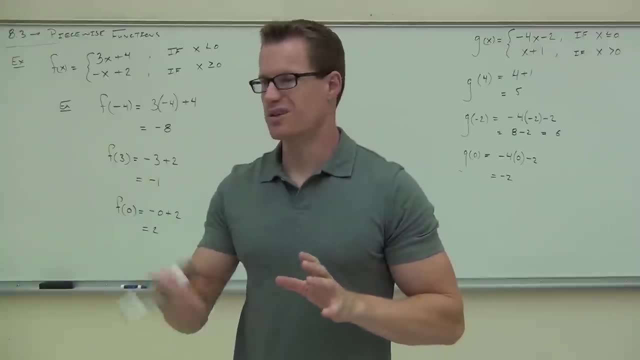 You just plug numbers in. If you plug into both of them- I know you don't know what you're doing- I'll just give you zero. If you plug it into one of them, then I know you know which. at least you know the idea. 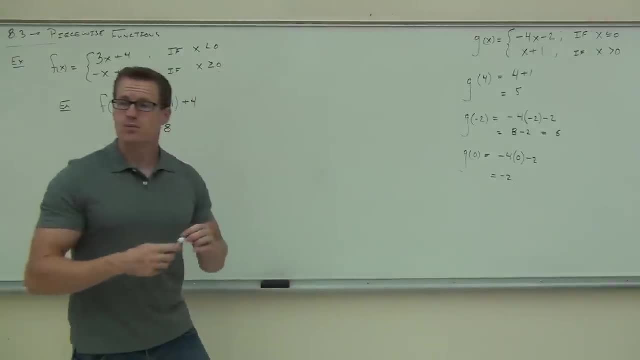 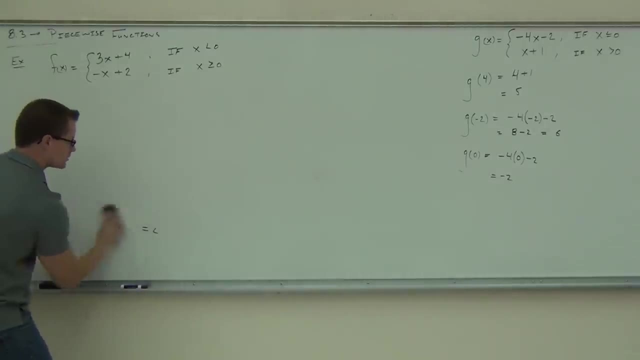 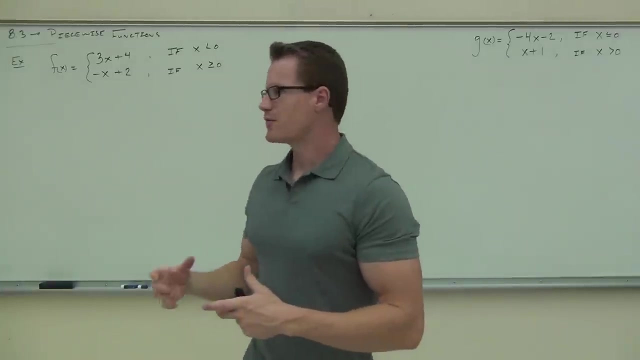 behind this. okay, So that's, that's your idea. Now, the second thing we're going to do is figure out how to graph these. Now. we'll just stick with the same ones. Now, I'd really like you to get away from graphing linear functions like like these are, with: 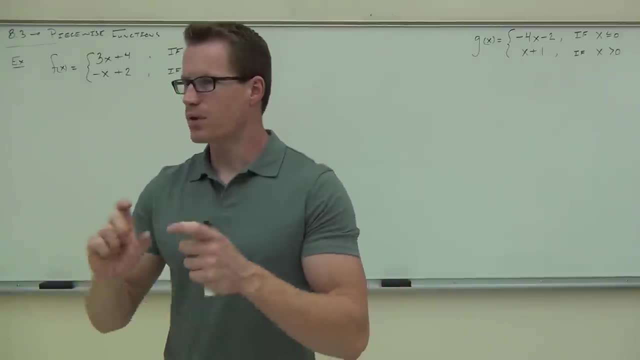 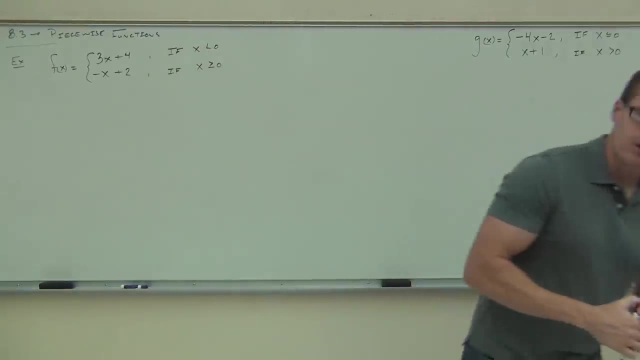 tables. It just takes. it takes too long, It takes a long time And plugging in negatives. sometimes people mess that up. So we really do need to be graphing with our y intercept and then using our slope, But how do we graph it in a piecewise function? 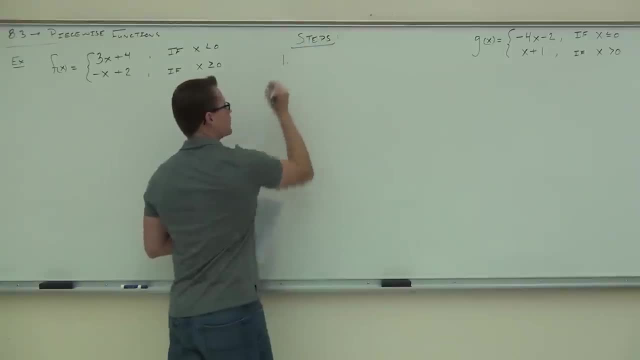 Well, here's our steps. The first thing I want you to do is do a little ignoring of one of these things. So, when we look at this piecewise function, I want to completely ignore This bottom part. okay, I'm actually going to completely ignore the directions for now. 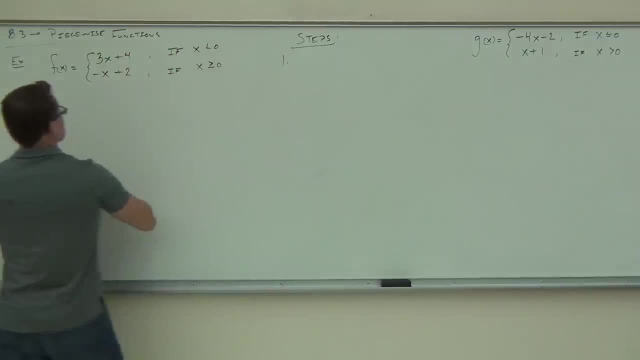 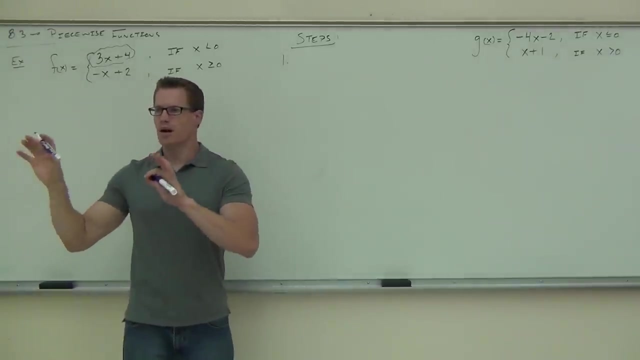 All I'm looking at right now is this: three x plus four. What we're going to do right now is graph just three x plus four, as if it were like y equals three x plus four. So our first step is we're going to ignore the rest of this, the problem, and graph the 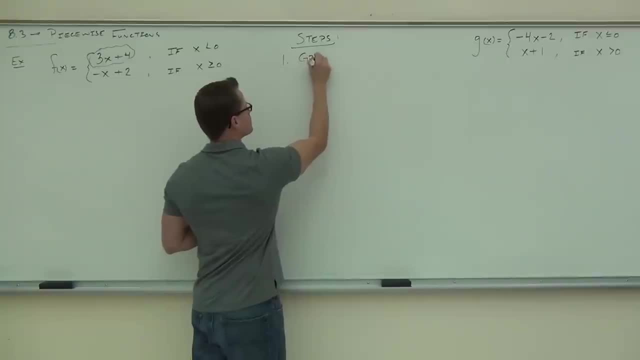 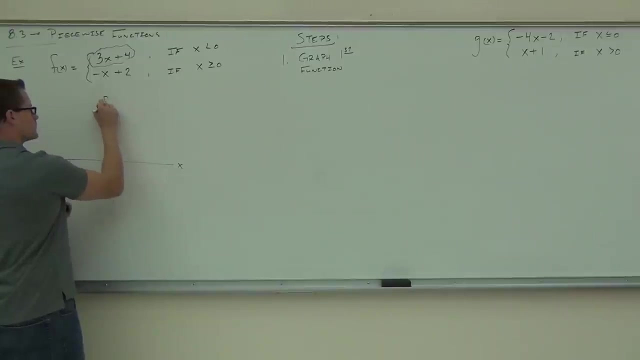 first function. Okay, So, So, So, So, Let's write that down. Okay, Let's see if we know where to do this. So, graphing the first function, three, x plus four, you can see that we're pretty easily. 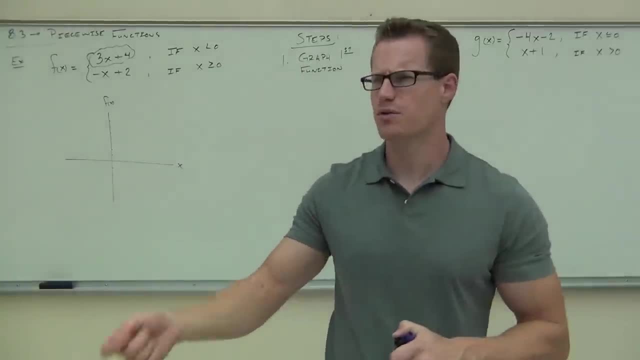 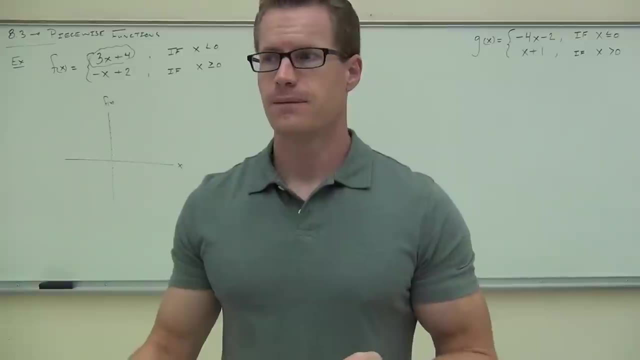 going to get it done. Okay, Again, let's go over this one more time. What's our y-intercept for 3x plus 4? What's that tell you to do? Okay, And we're going to put a point right there. 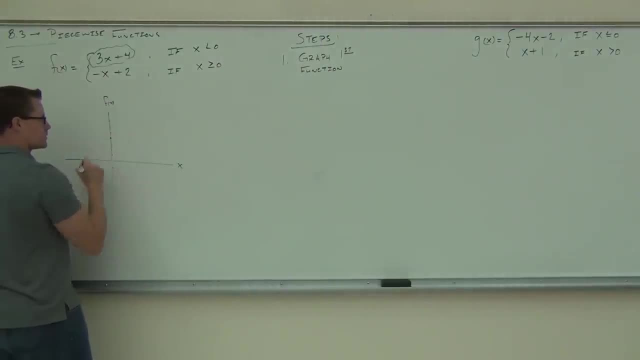 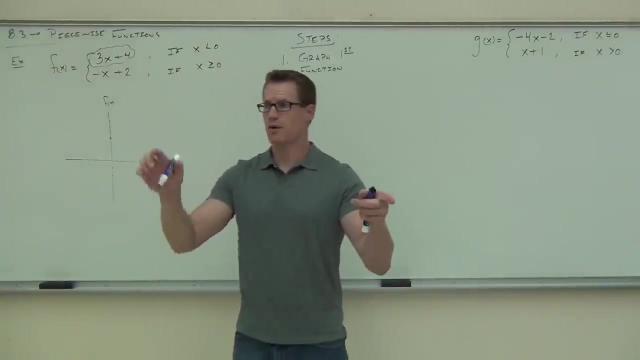 So 1,, 2,, 3,, 4 for the point right here. Now how do we find the next point? What do we do? Slope, Good, So someone on the right-hand side of the room? what's my slope? 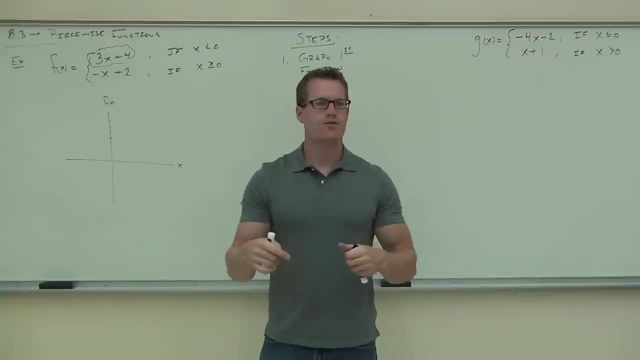 Good 3 over what? 1.. Okay, So from which point do I go? Do I go from the point I just plotted or from the origin, From the point you just plotted? Yeah, that's right. From that point. 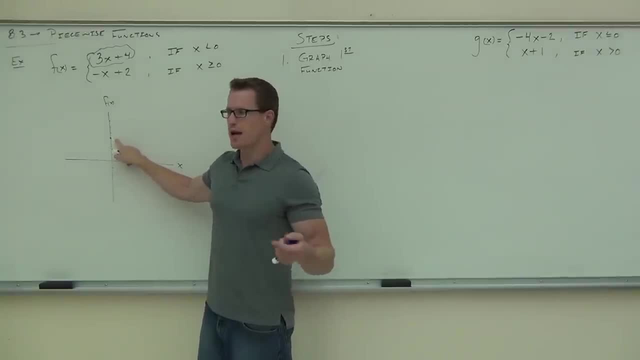 Why would we plot that point if we're not going to use it right? That wouldn't make any sense. So we have this point right here. From this point, our slope is 3 over 1.. We're going to go either up or down. 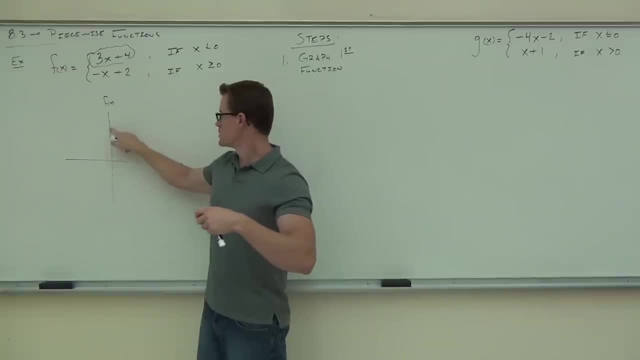 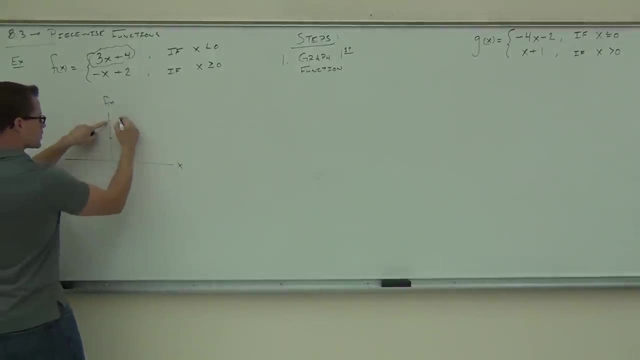 Which one Up Up, how many Up? 1,, 2,, 3.. And then over which way? To the right, To the right, That's right. So we go up 3 and over 1.. We'll put a point right there. 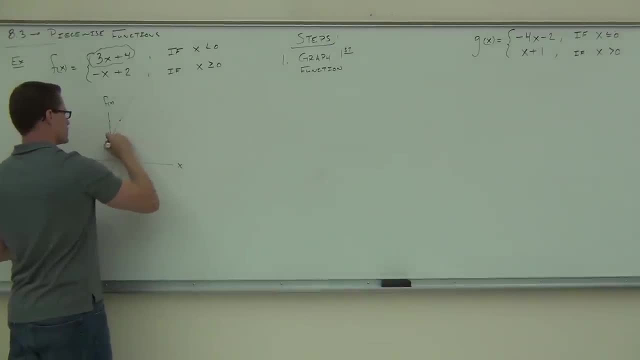 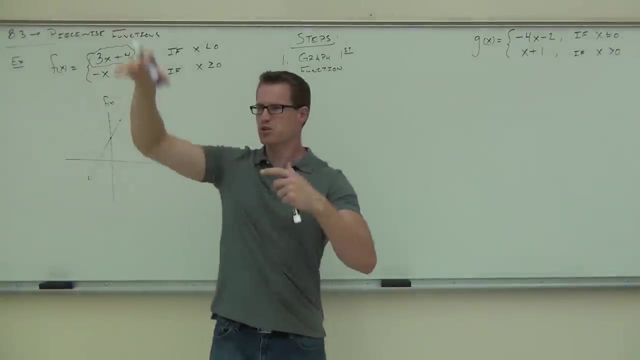 And we're going to graph this line. Would you please raise your hand, if you're okay, graphing that line for me? Good, We should be. We should all be at that point, at least at this point, right now. Now, Now's where those directions come in. 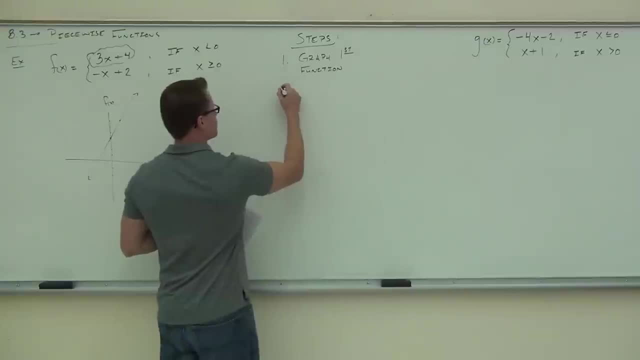 What we're going to do in the second step. we're going to do a little erasing. We're going to do this- It's going to sound Kind of weird- We're going to erase the part of the graph that doesn't actually exist. 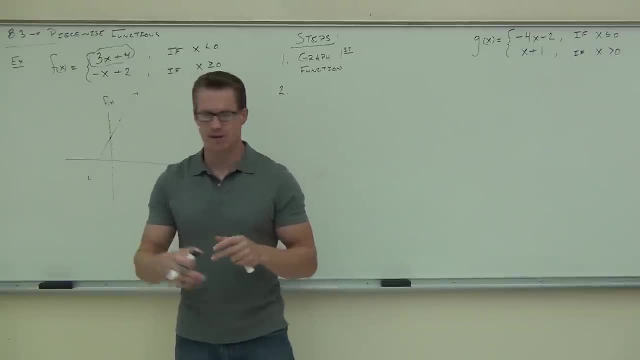 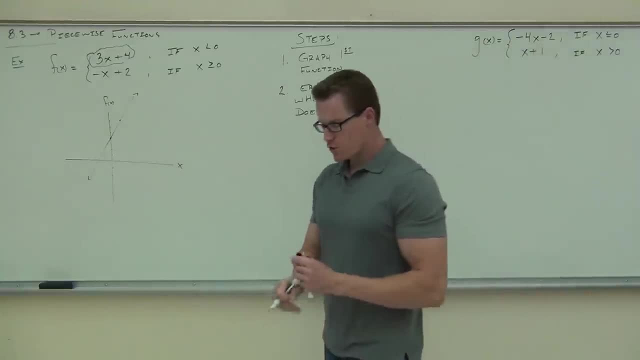 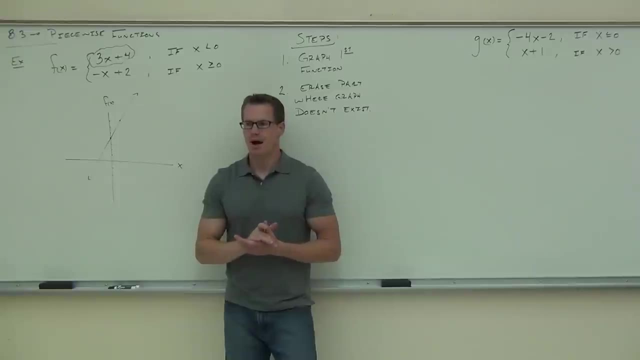 We're going to erase the part of the graph that doesn't actually exist. You see, here's the thing. If you remember anything about functions themselves, when we went over this, the very beginning of this chapter, I talked a little bit about what's called the vertical line test. 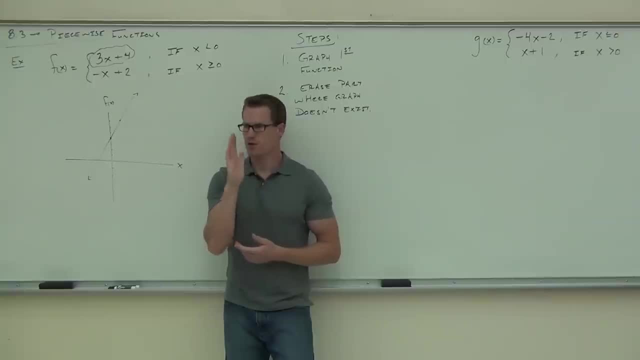 You ever heard of the vertical line test? What it says is that every vertical line must intersect a graph at only one spot. If it intersects at two spots, it's not a function. Have you ever done this? If I were to graph both these functions, I'll give you a report here real quick. 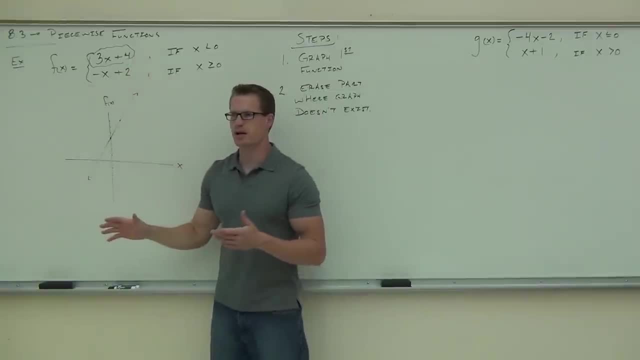 If I were to graph this one and this one, do you notice? they're going to be crossing right. They're not going to be a function as a whole. What I need to have is only one graph per little section. So that means I can't ever have a crossing of lines. 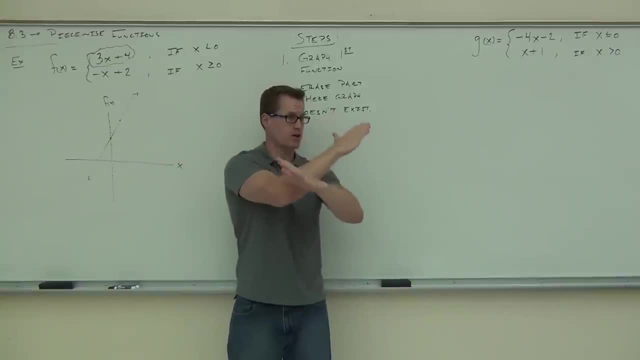 Nod your head if you're with me on that. I can't ever have two lines on top of each other. Are you with me? You can't ever get that, So we're going to erase half of this graph. You just have to pick the right half. 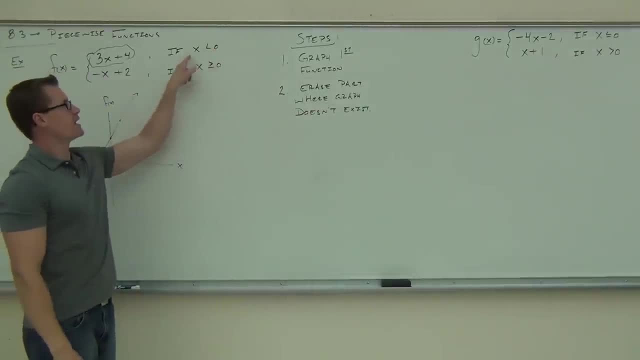 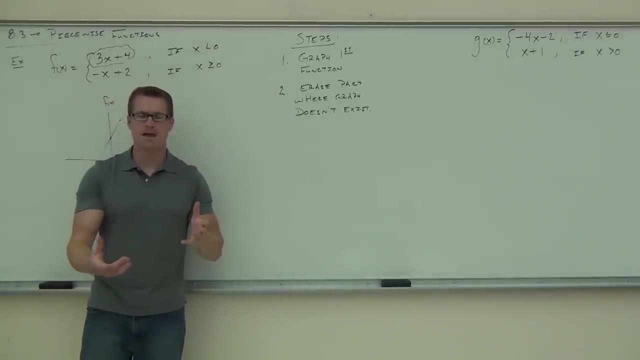 Here's how you do it. You're going to go to the point on the x-axis that's listed over here. It doesn't necessarily have to be. it's only zero in our case. Okie dokie. I just said okie dokie. 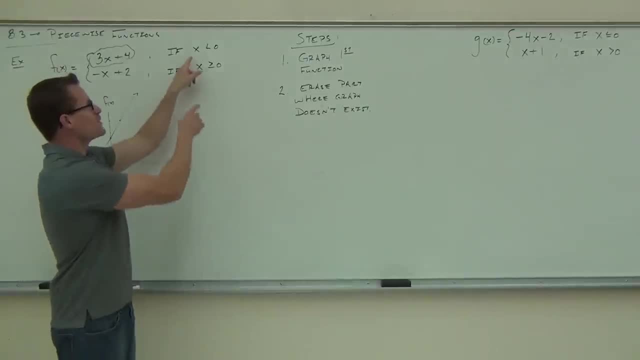 Wow, Old school. So we go to the point that says it says x is less than or x is greater than so. that clearly means we're on the x-axis. Let's go to this point. Tell me when I'm at that point. 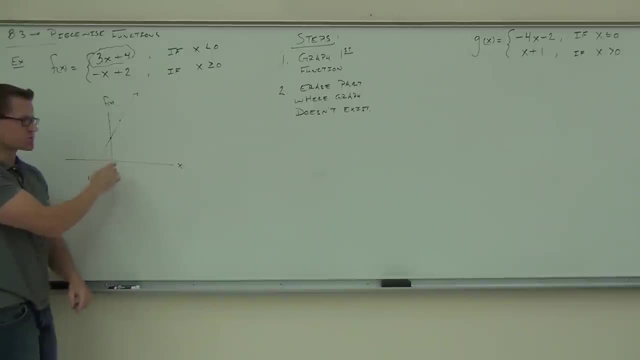 I stopped automatically because I'm right there. But you're at x equals zero. You with me on this? Now you're either going to erase the right side or the left side. The directions tell you what to do, So we're looking now at our directions. 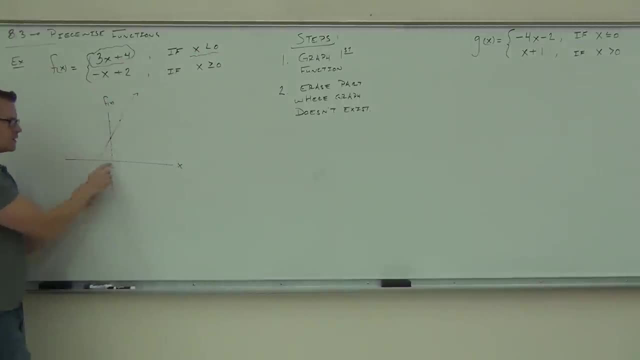 Where's my finger? according to the x? What's the value? again Zero. So I'm at the right spot. Tell me what's this number? One, Just according to the x right. One, two, three: What's this number over here? 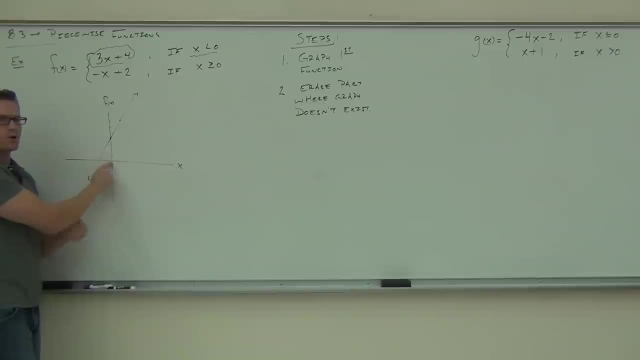 Negative one, Negative two, negative three. What we're going to do? we're going to find all the x's that satisfy this X is less than zero. Tell me something, ladies and gentlemen: Is this number less than zero? No, 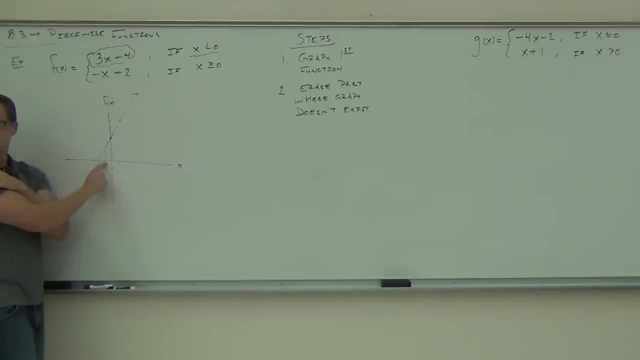 Ok. Is this number less than zero? No, Is this number less than zero? Yes, Yes, These are. can you agree that? these are all the numbers that are good for our top function? These are all the numbers that are bad for our top function. 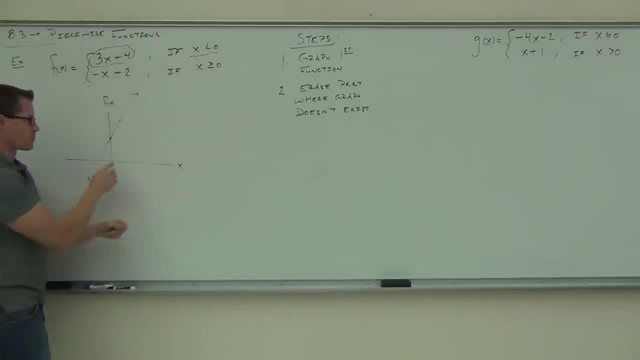 True, Yeah, Ok, So what we do? we go to our value zero Or whatever value's there. We're looking for the x's that are less than zero. This is less than zero. less than zero, That's true. 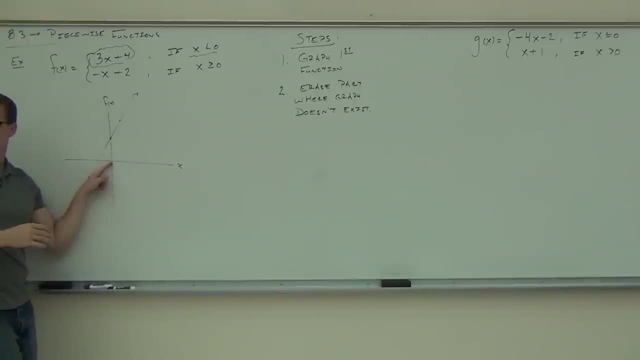 These ones are not less than zero. Are you all with me? Here's the key point: You're erasing, you're going to erase the ones that don't work for your function. So, if we want these ones, we're going to keep this half of the graph. 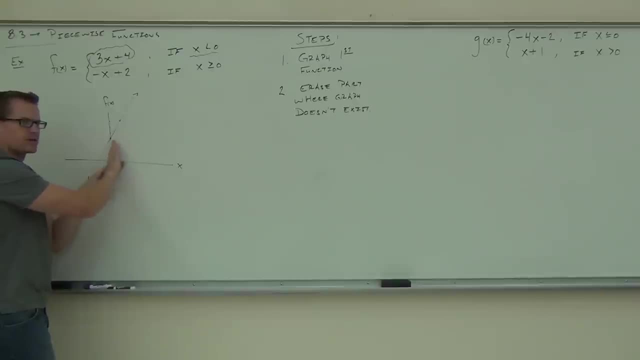 If we don't want these ones, we're going to erase everything that's to this side of the graph. Are you with me on this? We're going to erase it all. So everything from zero to the right is gone. Agreed. 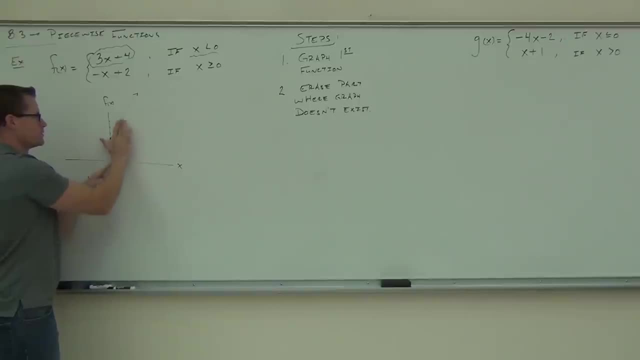 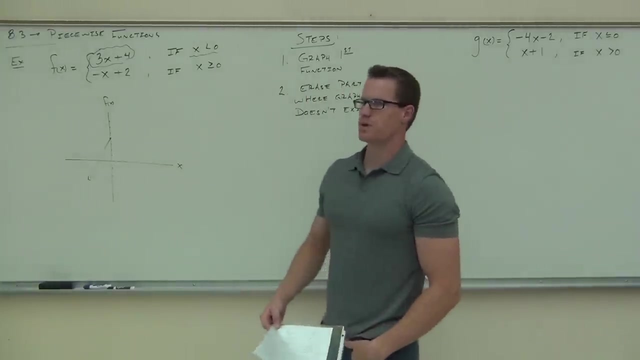 Yes or no? Yes, Everything from zero to the right. That half is gone. That's confusing for a lot of people. Every time that I teach, this is real confusing for people. So again, how you tell what to do, it really is all by your directions. 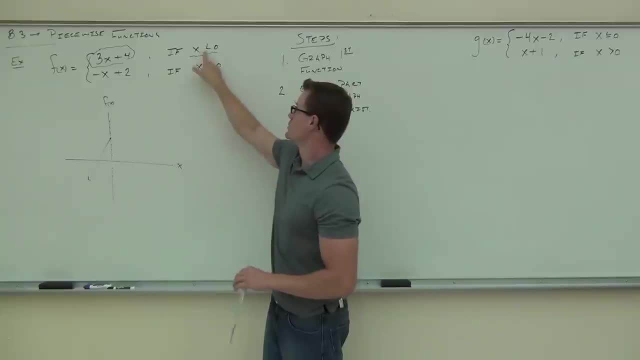 Treat it like a number line. ok, Treat it like a number line. You go to: x equals zero. That's here You look for the values that satisfy. x is less than zero, So x less than zero. Y'all nodded your head when I said which numbers are less than zero. 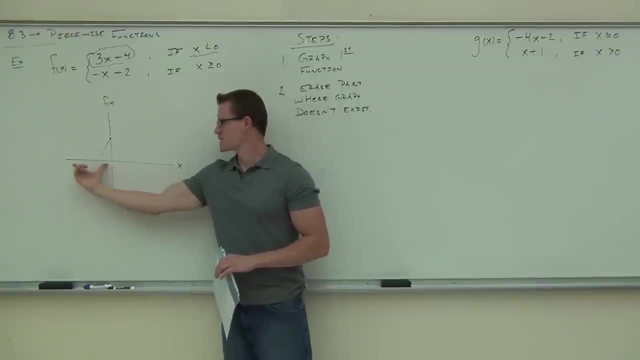 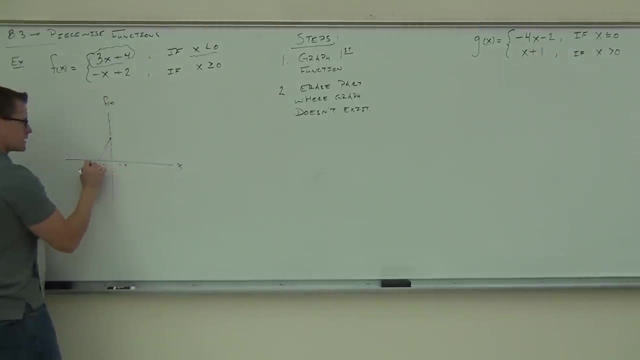 Are these numbers less than zero? Clearly not. Are these numbers less than zero? Definitely, This is a number line right. This is 1,, 2,, 3.. This is negative 1, negative 2, negative 3, and so on and so forth. 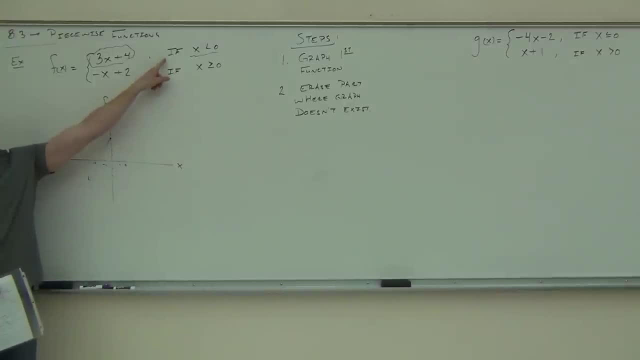 So are these numbers going to satisfy the top one? Let me ask you a question. folks, Look up at the board here with me. I asked you to plug in 4, didn't I in the previous example? Could you plug in positive 4 up here? 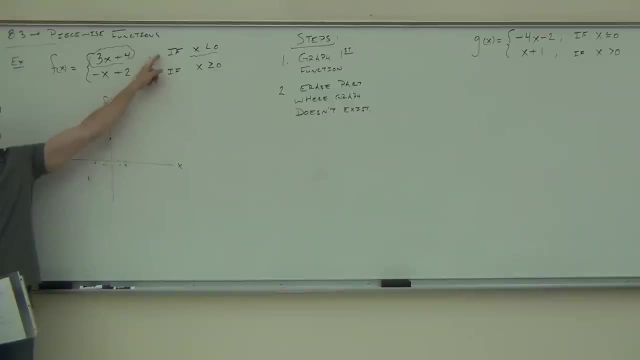 Where would you plug in positive 4, here or here top or bottom Bottom? Then why should we have half of a graph if we can't even plug those numbers in? Does that make sense? We shouldn't have that. If you plugged in positive 4, it would not go here. 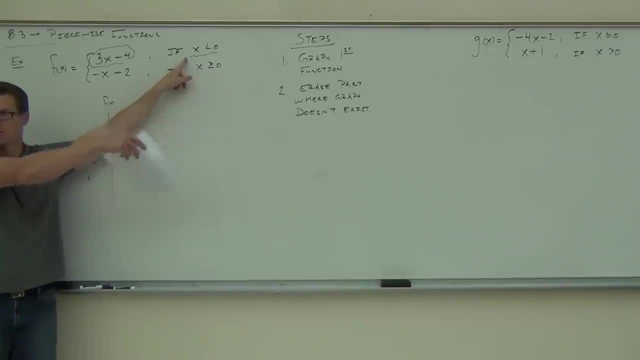 Are you with me on this? Because you all got that one right, right? If you all plugged in numbers over there correctly, we wouldn't even have a number 4 here, So we'd have to erase that part. yeah, Since the top one we're doing is, x is less than zero, couldn't it not? 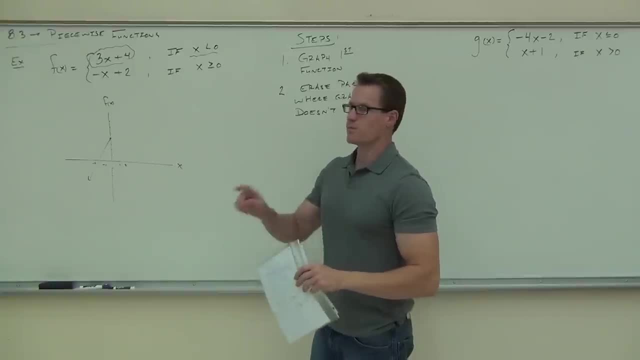 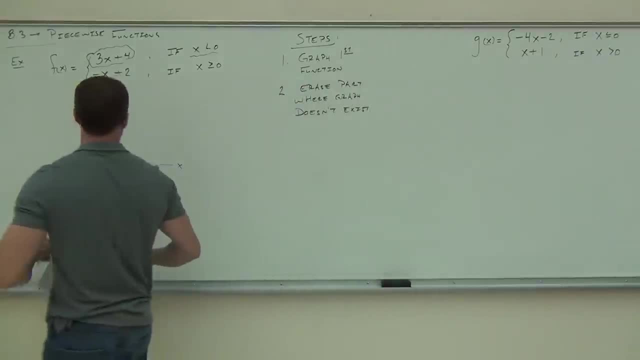 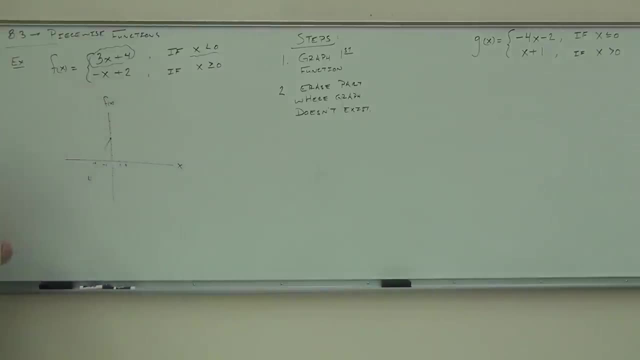 But just one. Okay, All right, So are we a little more clear on why we have this half of the graph and not that half of the graph version? If you're clearer, getting more clear on that, Good, Okay, We cannot plug in positive x's. 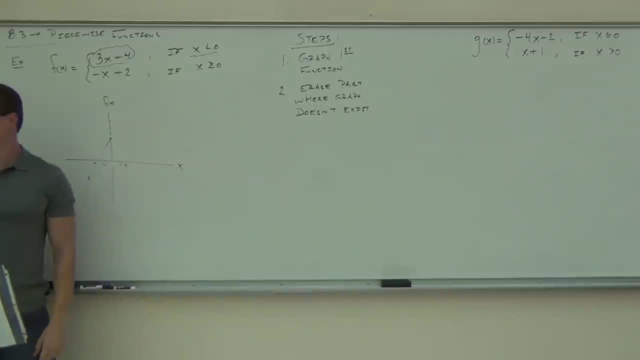 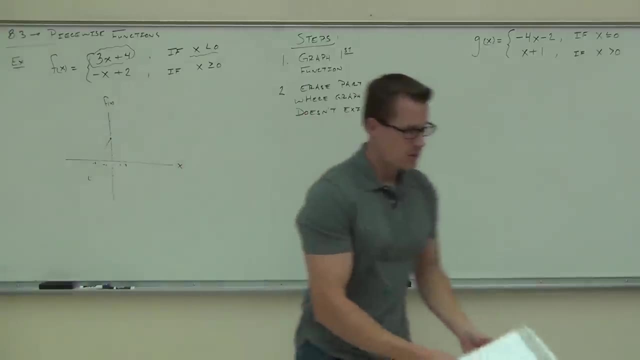 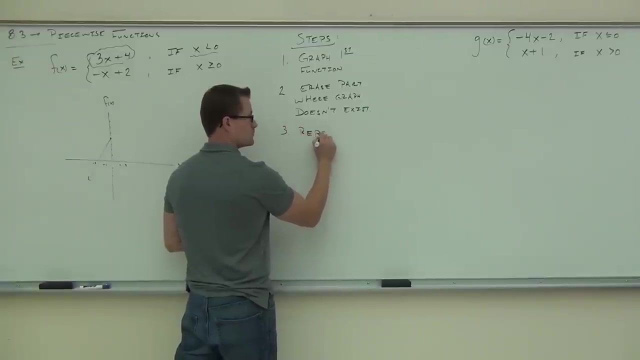 That's why we don't have positive x's on that graph. Yes, sir, Okay Now, after you do the top one, the bottom one's a little bit easier. You're going to repeat this for the second function And you're thinking: well, how is that easier? 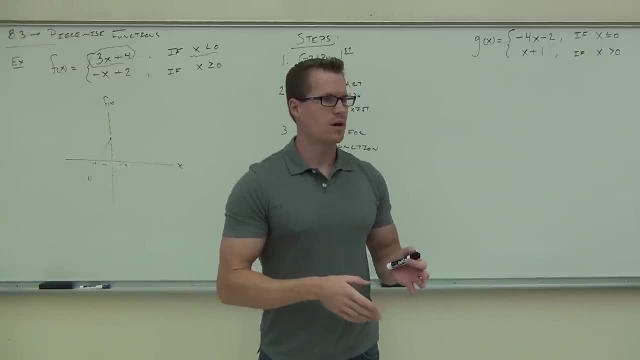 We have to do the same exact thing. Well, no, not really. You don't have to think as much. Here's why you don't have to think, And no one likes thinking right, We like it to be easy, We don't want to think about stuff. 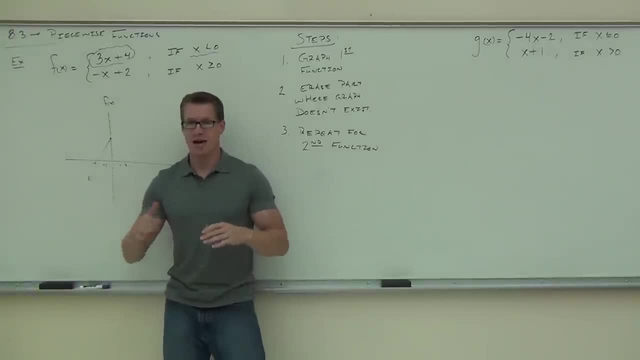 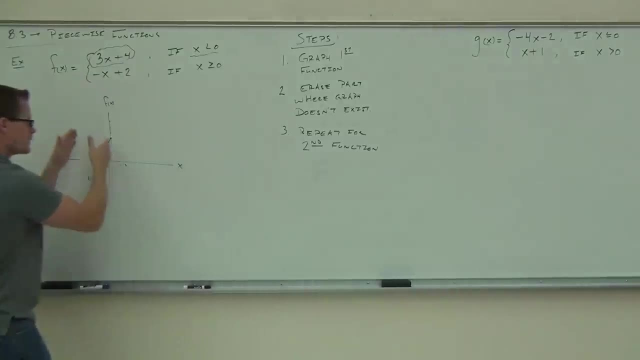 Here's why you don't have to think as much. Do you remember how I told you? you can never have two lines on top of each other? You can't ever have two lines in one segment. right? You've already figured out that this is where this graph is supposed to be true? 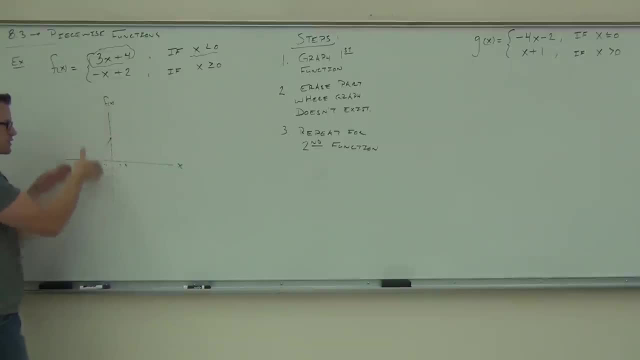 So tell me something: If this graph is here, where's the second graph going to be Here? It should be here, OK, So we already have a graph in this segment. If we have a graph here, we can't put another one in that segment. 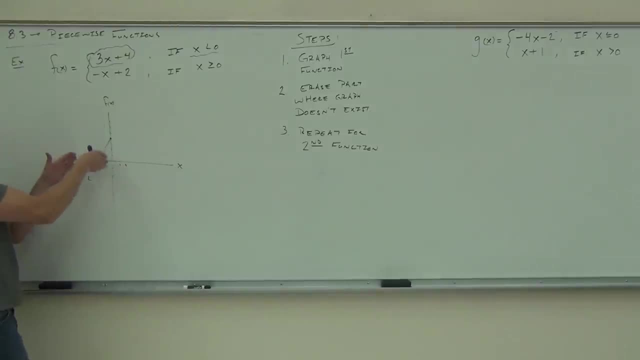 It's got to go in the next segment. So if we have one here already, we know the next one's going to be here. It has to be that way. They can't both be in the same little section, So let's go ahead and repeat that for the second function. 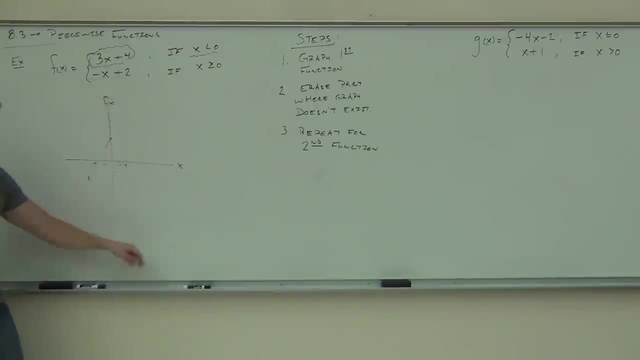 Tell me something. What's my y-intercept here? 2. So we're going to go up to 2 and put a point. What's my slope, ladies and gentlemen? 1. What's that tell you to do? Go down. 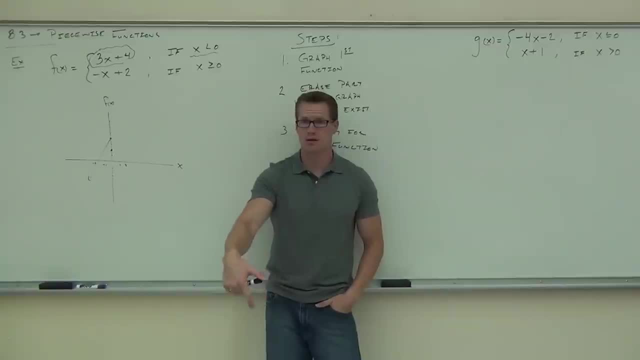 Down, Down, because it's negative, sure. And then to the left or right, Right, Right, Yeah. So from our point, we'll go down 1 over 1.. Here's what you can do with this one. You can draw the whole line. 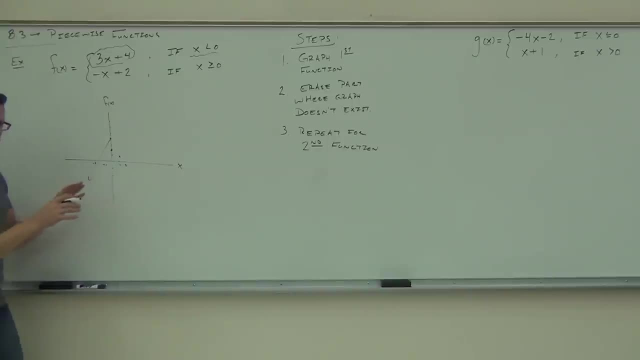 And I'm going to do it this one time, just to kind of show you that this is going to work. If I draw the whole line, we're ignoring the purple line. I want you to go to this line, This point. So we're going to go to x equals 0 again. 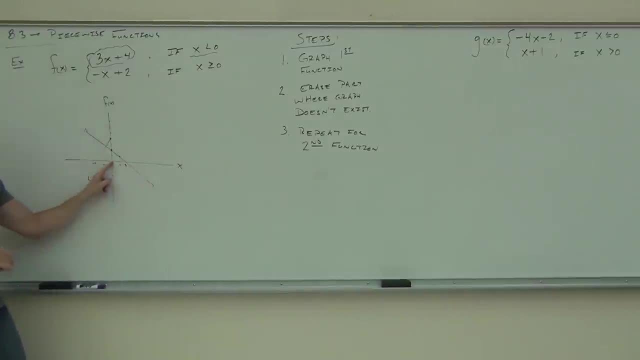 And we're going to look for the points of x that are greater than 0.. We'll go through the same process. Is this number greater than 0?? No, Is this number greater than 0?? Yes, Great. So these are the ones that are going to work for us. 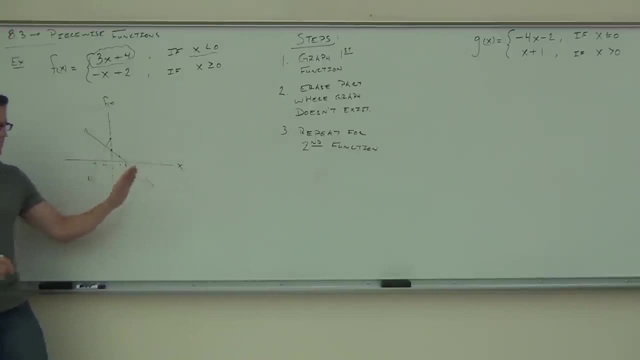 Are you with me These points? they're not going to work for us. We have to erase this half of the line. Now, before I erase it all, I want you to look at something. Do you see what I mean by the two lines overlapping? 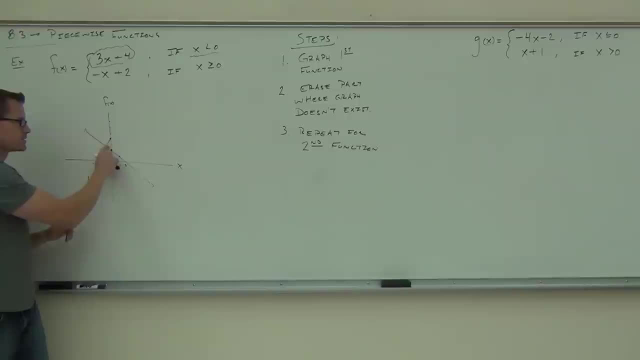 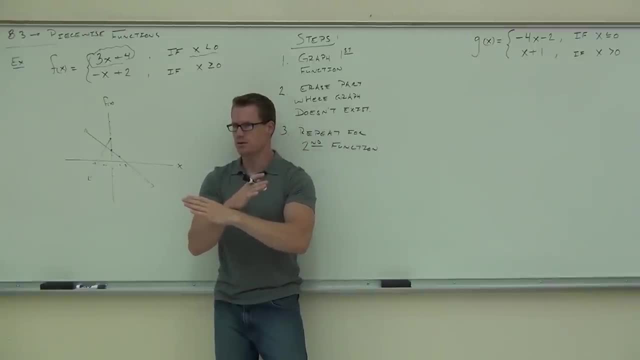 like this. you know you've done something wrong. You with me on that. You know something's going, Something's a little fishy. We can't have that. So you're never, ever going to get two lines in the same vertical segment. 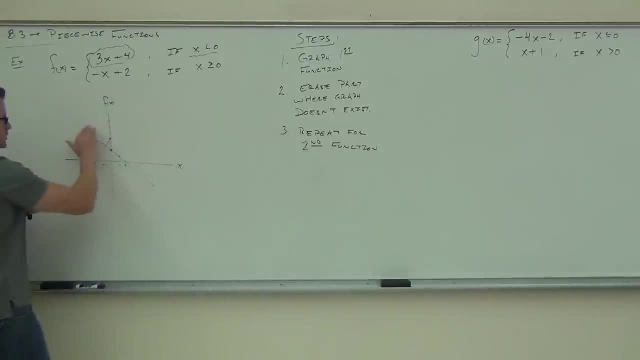 That cannot happen. So when we look at this, really if you were to start this over, if you were to start this over really could just say: okay, well, here's my y-intercept, I go down one over one Can. 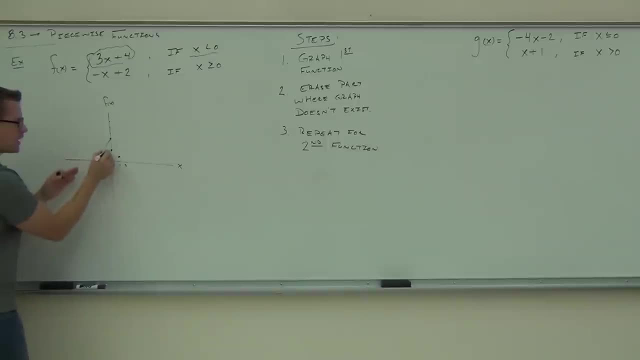 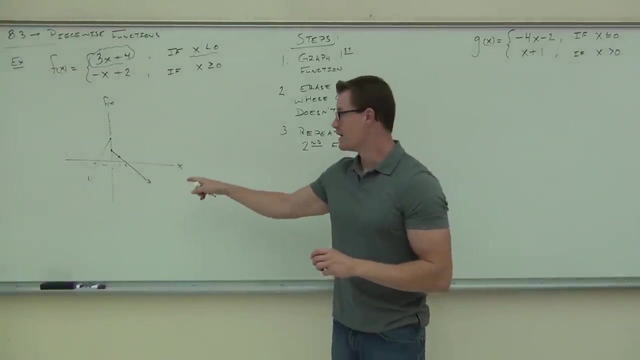 I possibly graph this way. No, No, I'm going to get a crossover over there. I'm just going to graph this way. That's your piecewise function. Now there's one other little part that I need to tell you about, but for right now, how many people are okay getting that far? 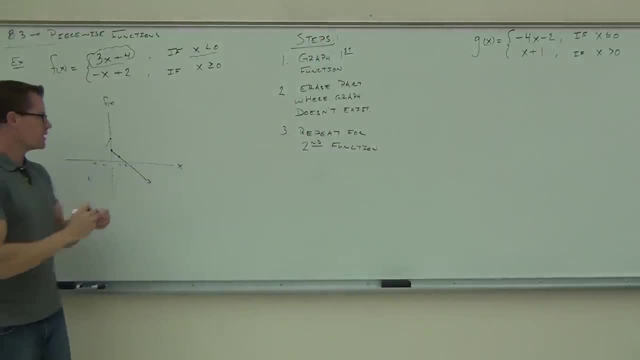 Good, Now, Jose brought up a good point, Don't? we have two points right here, And we know that can't happen, right? Well, which one do you keep? And that's answered by your directions again, The equals one that says you have a point there, How we represent the points. 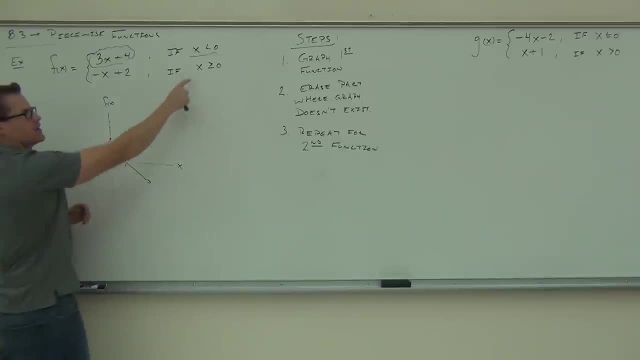 not actually there is by an open circle. So when you look at this, it says x equals zero, x equals zero. on the second graph We're going to keep this point solid. That's going to be a solid point. x is less than zero. It means I can get all the way up to zero. but 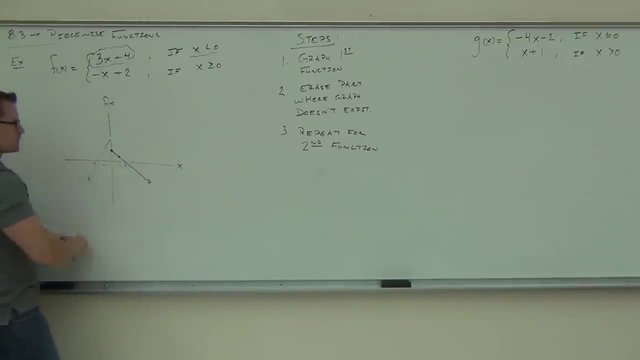 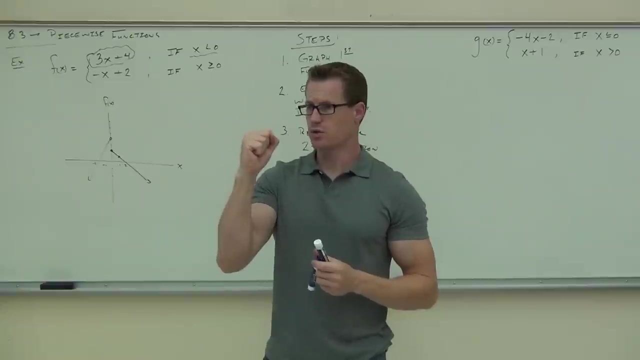 I can't actually plug it in. I'm going to make sure I'm doing this right. I'm going to make sure I'm doing this right. I'm going to make sure I'm doing this right. So, wherever it's equals, equals means a closed circle. Wherever it's not, equals that. 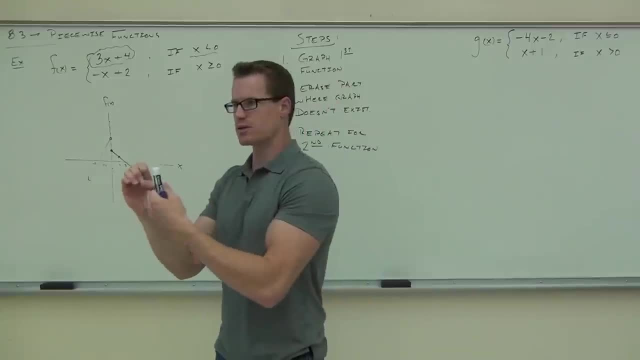 means an open circle. Open circle means you can't actually plug in zero. Where we plug in zero when we actually did a problem, well, that was down here, It just equals zero. We didn't actually plug in zero to the top function. How many people feel okay with this graphing? 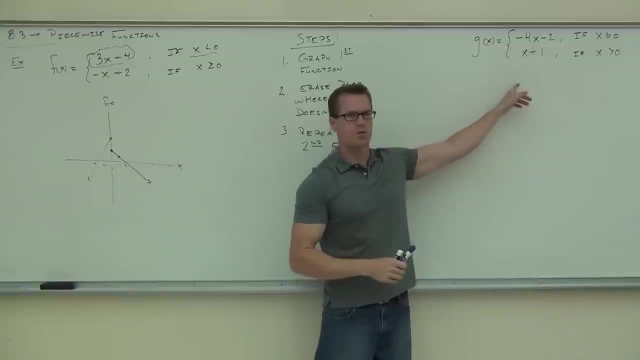 What I'd like to do. I want you to try that one on your own. Go through the same process. graph that We'll take a couple minutes to do this. I'll be walking around. If you need help, just raise your hand. I'll give you a hand. 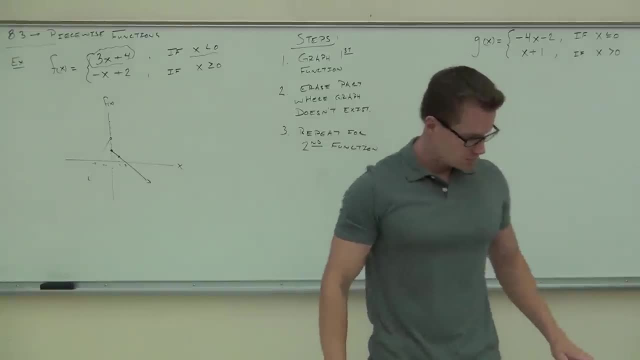 What do we have on this? one Equals is closed When it says like less than or equal to That. equal to that means closed. If it's just open, if it's just greater than or just less than, that means you have the open. 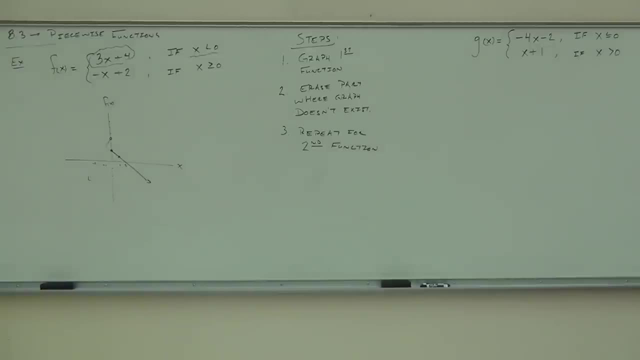 more, less than or equal to. Thank you, Okay. we're going to graph the first one. I want to make sure that you have this part down, right, okay? So when we're looking, 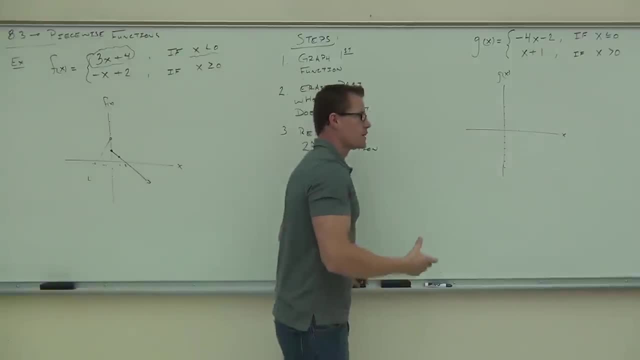 to graph these things. we really don't need a table. What we need is to understand the slope intercept form and use that to graph our line. When we do this, we're going to ignore the second function completely. We're just going to 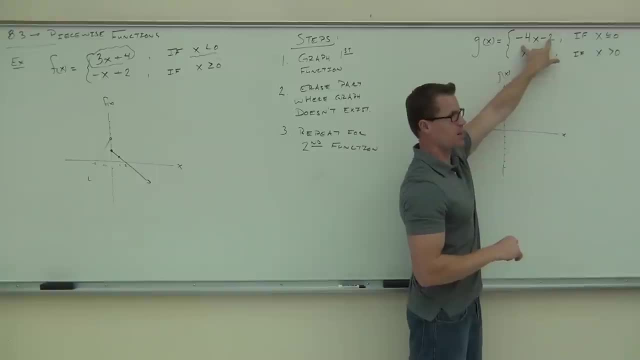 look at the top function right here. Now we're looking at the negative 4x minus 2.. What's your line intercept for the negative 4x minus 2? Negative 2. That means I'm going to go down 2. 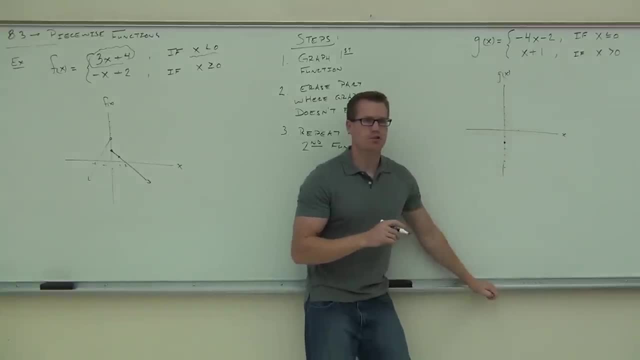 and I'm going to put a point: Did you all get that far at least? Yeah, Good, What's your slope there? Negative, 4.. So that says I do what? Down 1.. And then Down 1.. Okay, so 1,, 2,, 3,, 4,. 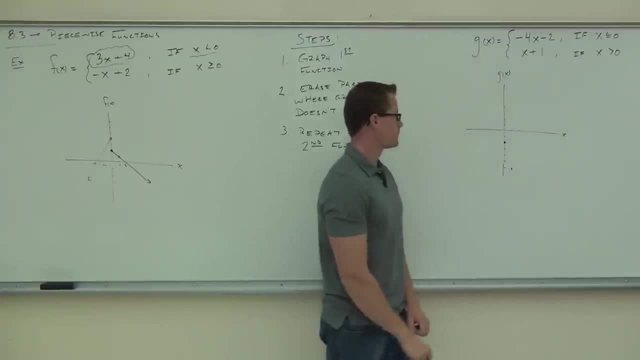 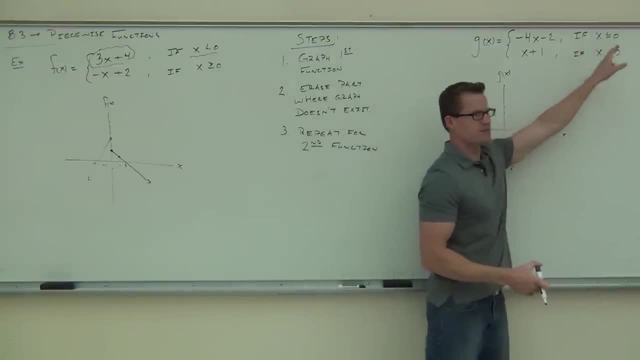 I know my negative. I know x is supposed to be less than 0.. My negatives are what I'm looking for in this case, but my point's off to the right. That's okay. Remember, you're going to be erasing. 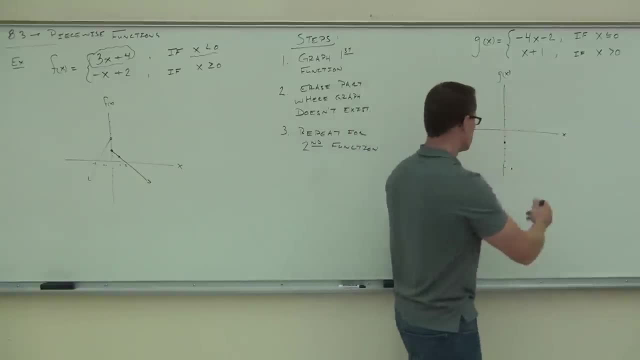 half your line, right, So use that to draw your line. So there's my whole function. How many of you feel okay getting that part of it? Good, All right, so we have our whole line here. Now we're going to erase. 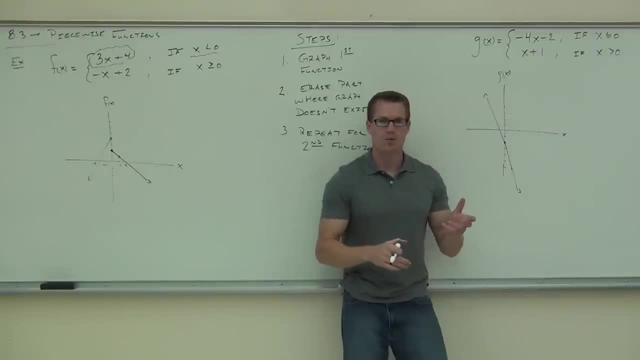 half of it. Which half do we want? Now, remember, we can only have one vertical segment that works for our graph on each side of our number that's given. In our case, it's 0 again. So either this one's going to be okay. 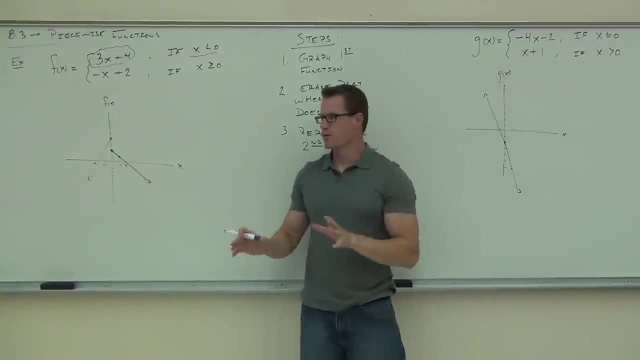 or this one's going to be okay, but not both, Only one or the other. Which one is okay? Which one is less than 0 as far as the x goes? Is this less than 0?? Yes, This one. So this is the side. 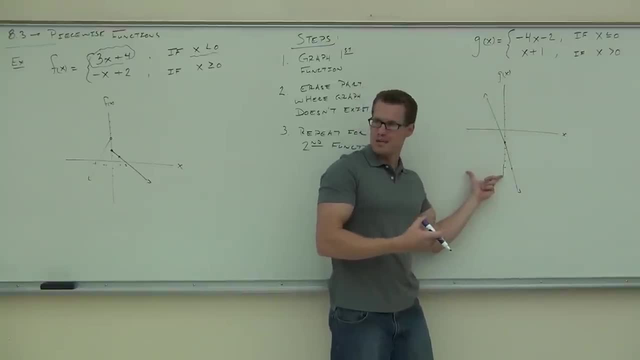 that we're going to erase or keep. What do you think Keep? We're going to keep that side. How about this side? Is this the side we're going to keep? No, No, because it says we want x is less than 0.. 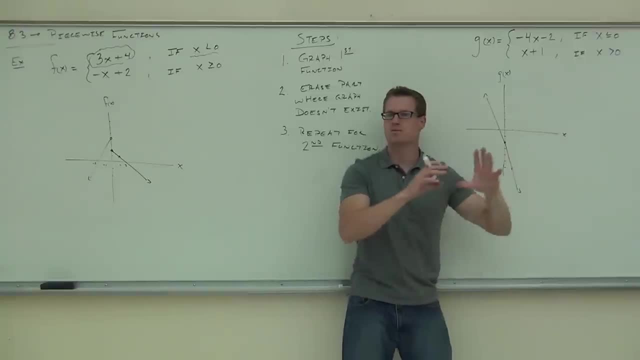 This x is greater than 0.. We don't want this side. This side's going to be erased. So again, we go to our 0.. We follow our directions. We want x's less than or equal to 0.. This is less than 0. 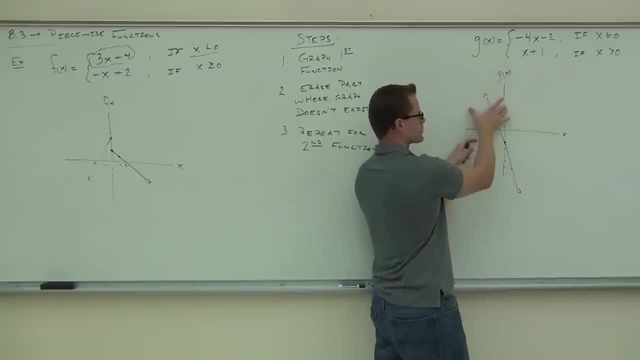 This is less than 0.. This is That means I'm keeping this vertical segment. This is not less than 0.. This is less than 0.. This is not less than 0. I'm erasing this vertical segment. So nothing on this side. 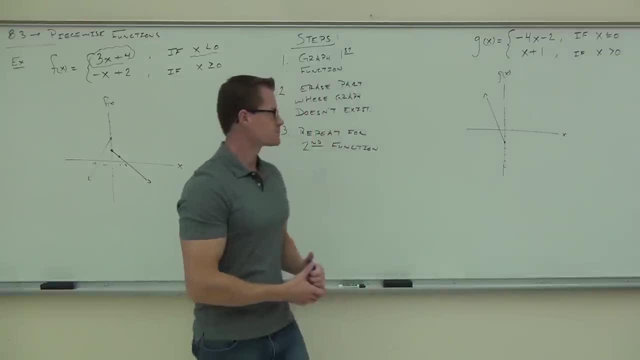 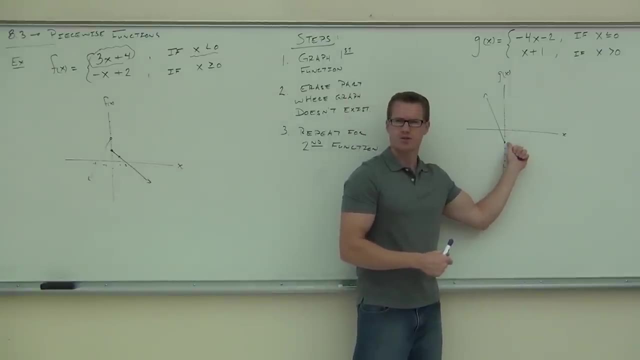 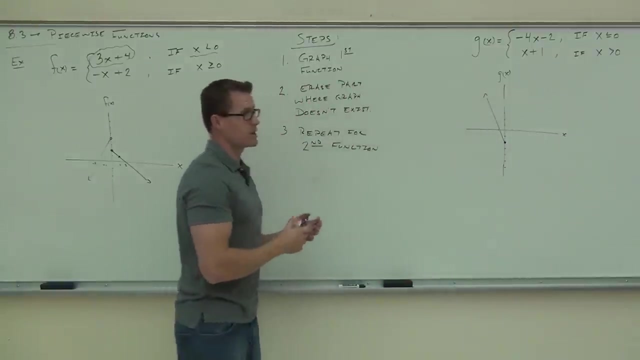 of the graph should be there right now. Another question: Should I have a point here or an open circle there? What tells you you're supposed to have a point? Good, So I should have that solid point there. Hey, that's half our graph. 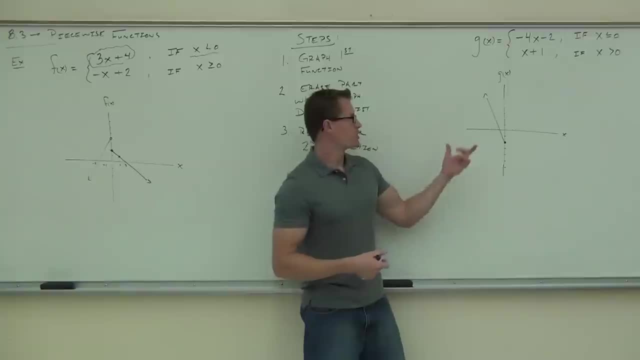 Tell me something. Where should the next half of our graph go? Should it go on the left-hand side or the right-hand side? That's why it's so crucial to get down the first function correctly. You have to have this part, right? 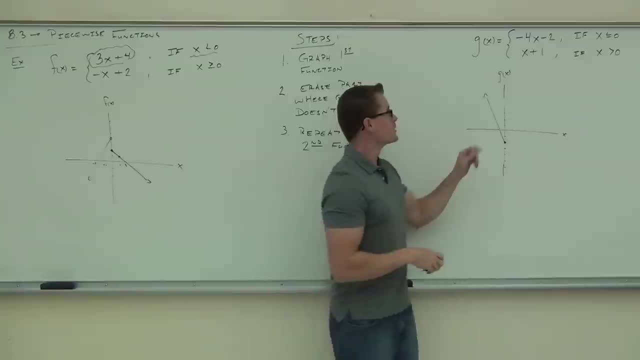 Otherwise you're going to have your graph flip-flopped. It's not going to look right. So the next one is x plus 1.. We're going to go plus 1 on the y-axis. That's our y-intercept. 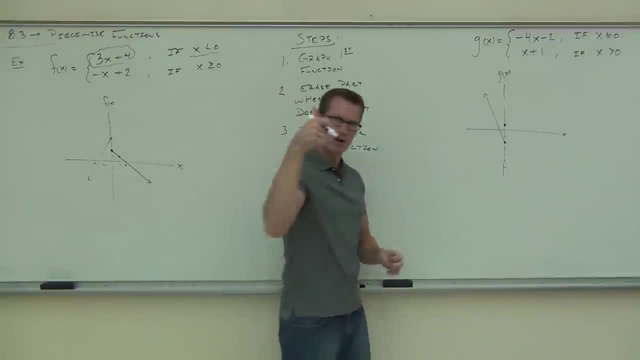 We go up 1 over 1 because our slope is positive 1.. It says up 1, right 1.. Now I don't have to graph the whole line anymore. Do you see why I don't have to graph the whole line anymore? 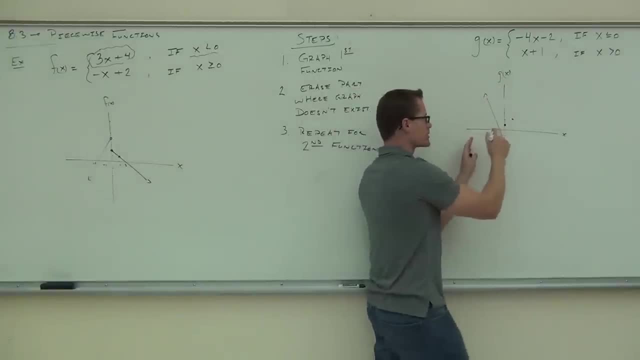 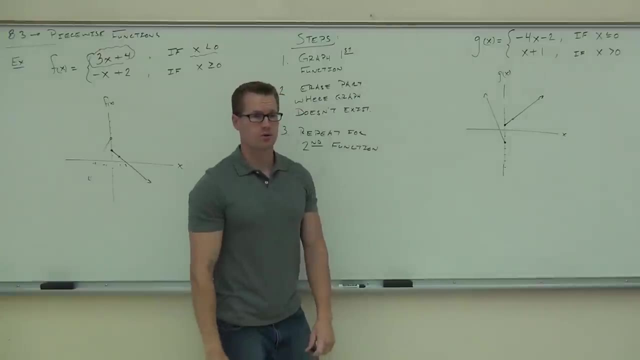 I already know that this side has a function, already has part of that piecewise function. I'm just going to be going that way. Why is it an open circle? Because it doesn't have that equal to 1 here. Good, So I'm going to change. 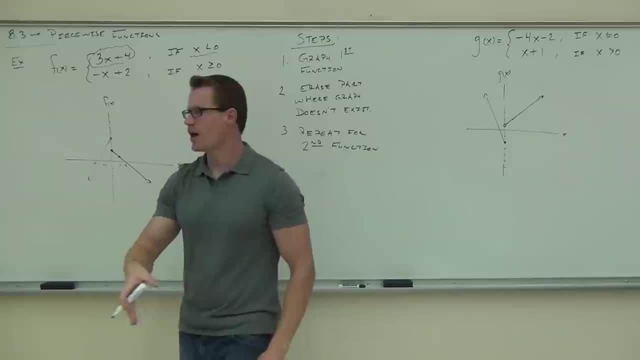 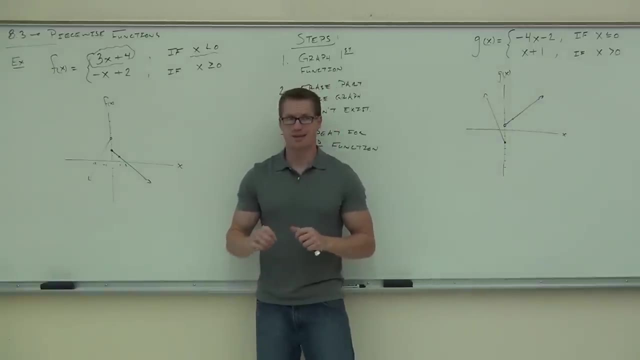 that to an open Can't ever have two points in the same vertical line. So we're done right there at that point. Do you feel okay with this graphing? It might take a while. This is brand new for you. I mean, this is like whoa. 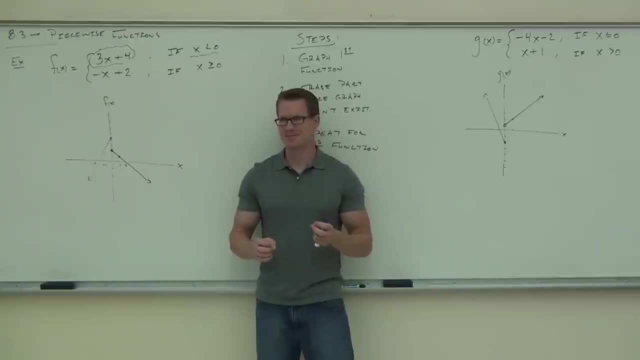 For some of you, you're like, oh, hmm, you don't want to go down there. I know that you might not want to do this. right now It's graphing two lines in one and then erasing half of our graphs, right? 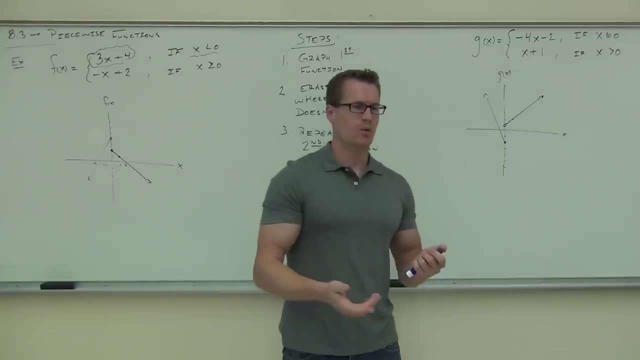 It seems kind of weird, But graphing piecewise actually happens a lot. When you get to calculus- hopefully you will get to calculus- you're going to be graphing and looking at a lot of piecewise functions, So you kind of have to know how. 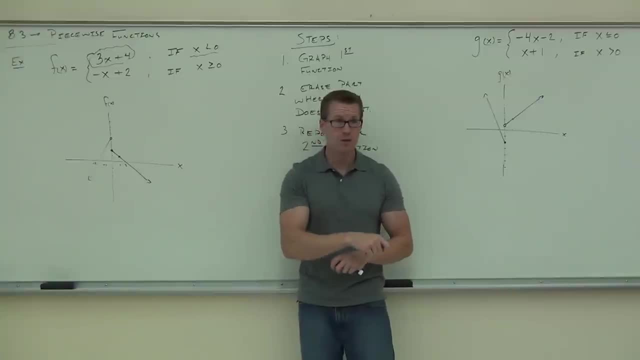 to manipulate them now. So take some time, Go back and watch this video again if you really are just kind of struggling. still, You want to see how to do it again. I think it took 35 minutes to explain these two examples here. 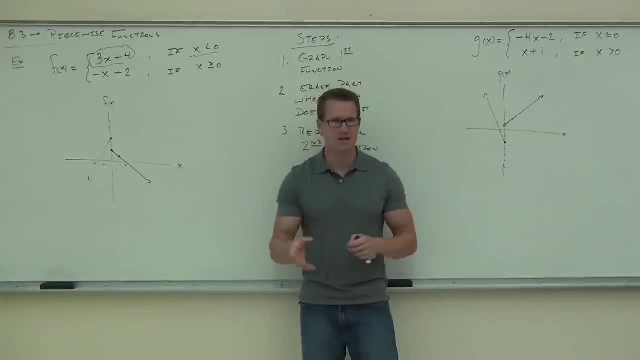 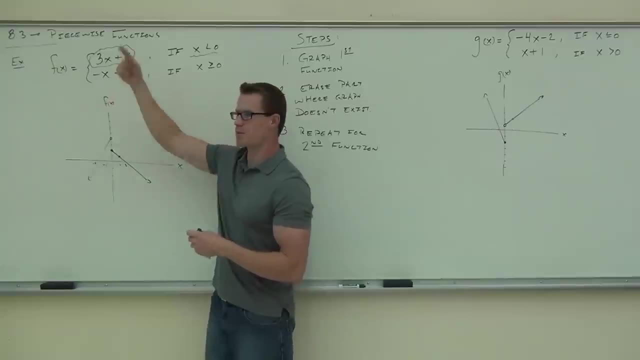 So go back and look at those until you really have an idea about how to graph these lines. The graphing part shouldn't be a problem. Everybody in here should be able to go up four- I'm sorry, to a one instead of four. 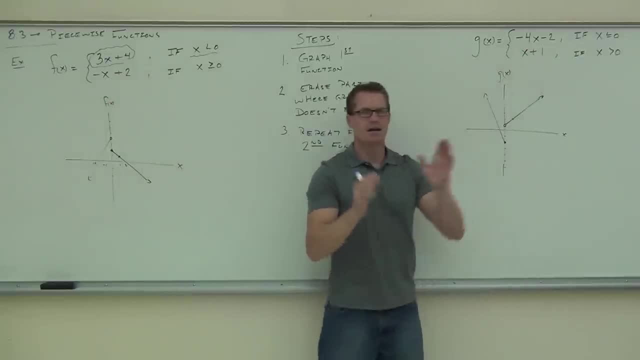 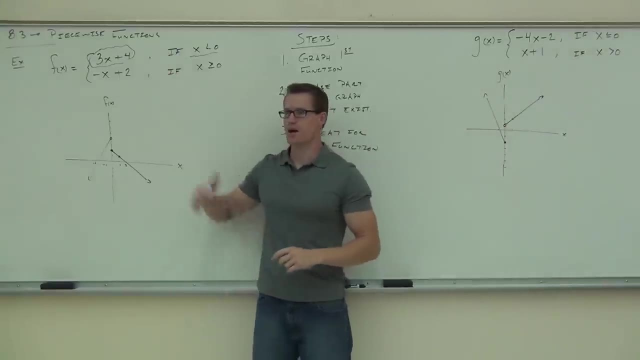 up three over one. Everyone can do that. Everyone can graph these individually. It's identifying which half of the graph to erase And how you do that is by looking right here at your directions for your graph. Can we move on or are we okay? 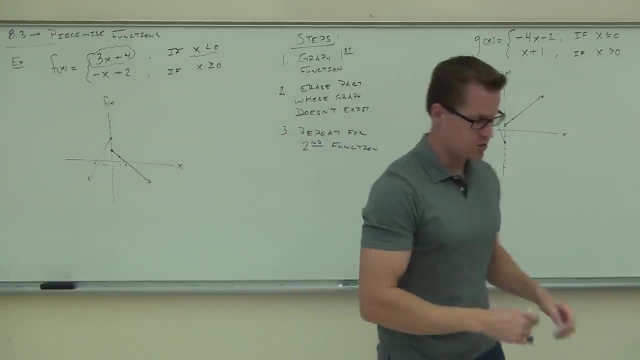 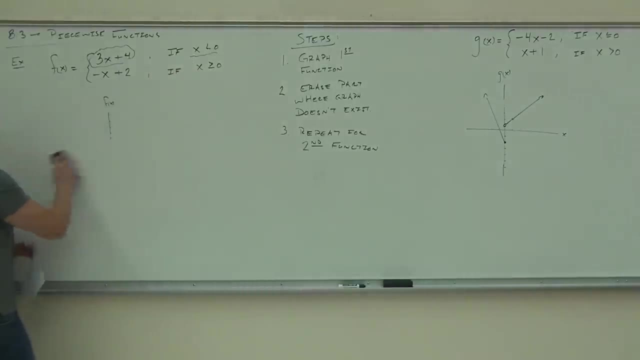 with that, All right. Now the next part that we're going to talk about in Section 8.3 is how to manipulate the graphs once we know what they are. If you remember from 8.2, we took a lot of time. 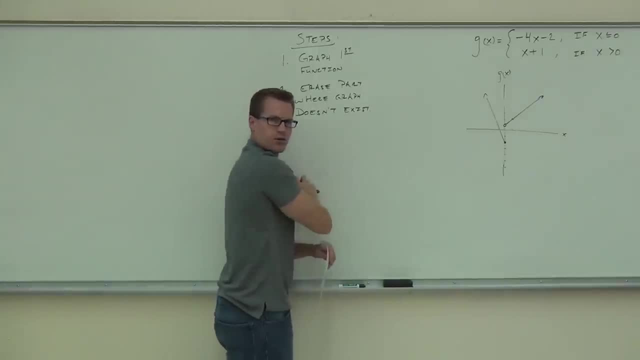 and we graphed some non-linear functions. You remember those non-linear functions. We had basically four shapes. We have basically four basic shapes for graphing The first graph that we had, and this is back from a long time ago, like math A-days. 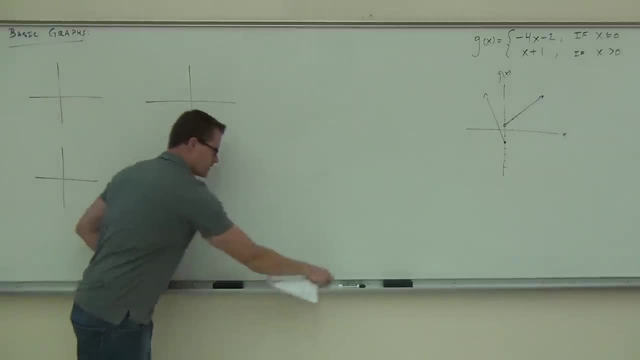 The first graph you see when you're graphing, things are your typical straight lines. This would be the graph f of x equals 3.2.. This would be the graph f equals x or y equals x Once you plug in for x. 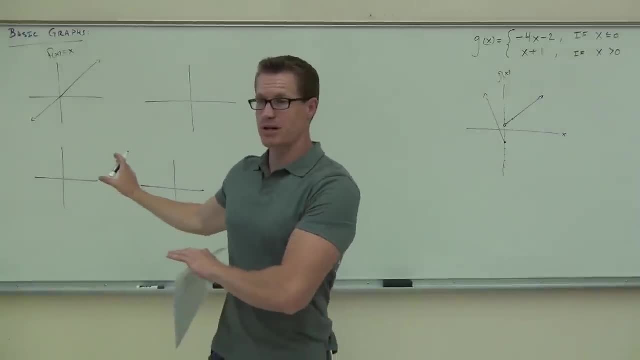 you get out for y. That's why we have that diagonal line right there. This is no big surprise. We've had lines pretty much our whole lives, right, So we've had these for a long time. The other ones we learned yesterday. 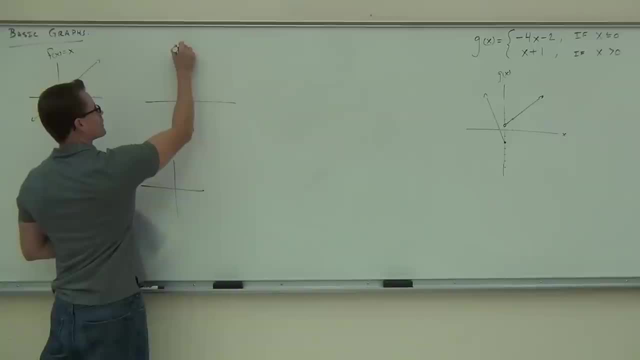 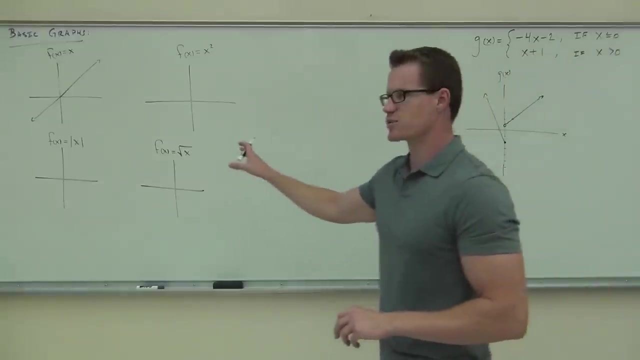 or not. yesterday, two days ago, was f of x equals x squared: the absolute value of x and the absolute value of x And the square root of x. If you were here a couple days ago, you know these make some weird. 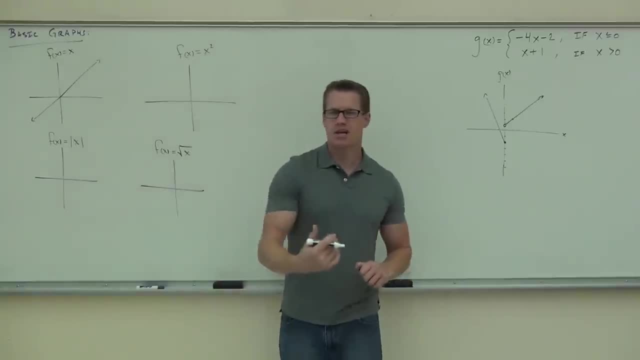 looking graphs, some of these things. Do you remember the shape of f, of x equals x squared. Do you remember what shape we got out of that Parabola? Yeah, show me with your hands how that looks. U Is it the v one? 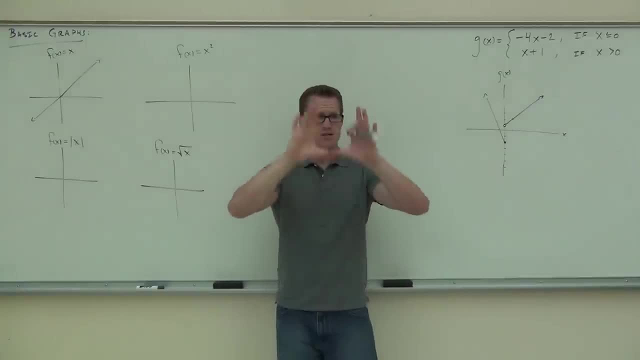 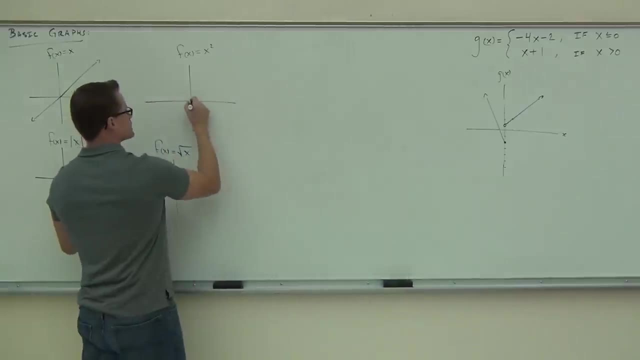 Or the u one U. Yeah, that's exactly right. Was it upward facing or downward facing? It depended on what sign was in front of it. right, But the negative made it go down. This one was upward facing. How about this absolute value of x? 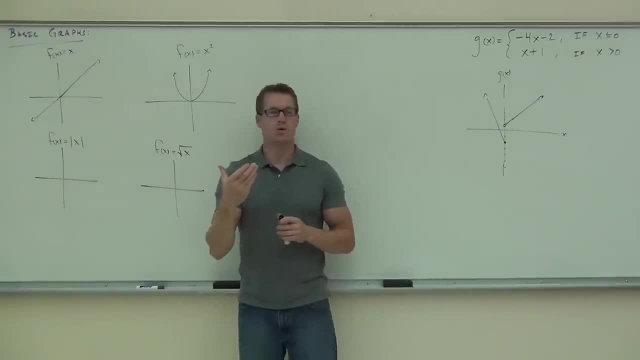 Absolute value of x. was that also a u? No, it was a v. Oh, okay, So that was the one that was just like that started at the origin went up as a v. The way I remember that absolute value equals a v. 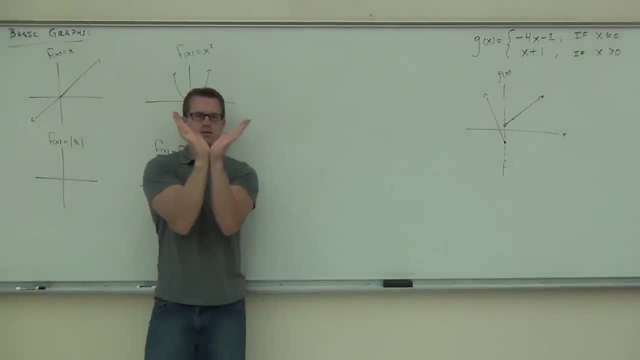 the v has two straight lines that come together. right, This has two straight lines, So take those lines and put them together. it makes a v. Does that make sense to you? That's how I remember it. Okay, very good. 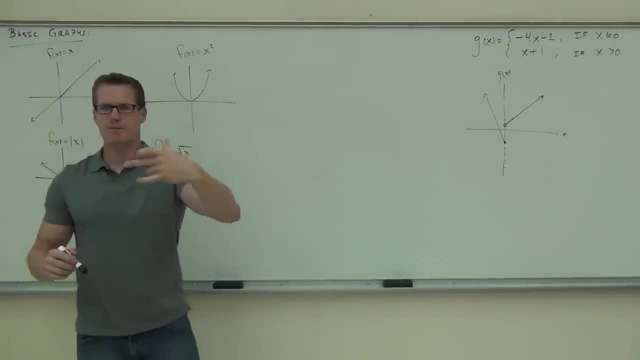 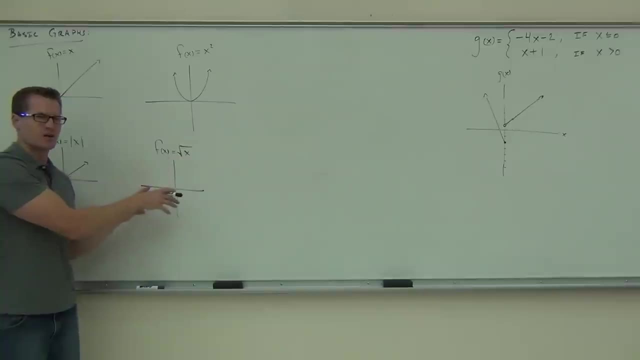 And this is the one. we shifted vertically. We added one onto the end of it and it made it move up one. Do you remember that? Awesome, That's why we went over that, so this would be kind of easier. And then this last one: this wasn't the u, this wasn't the v. 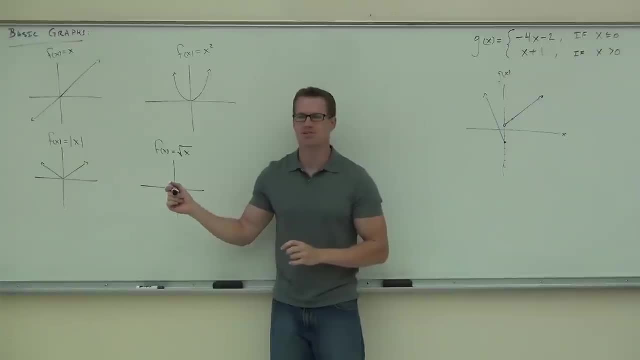 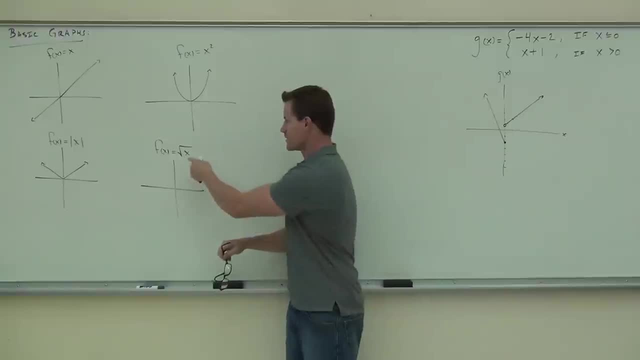 if you take my glasses off and you kind of look at it like that, this kind of looks like the shape of the graph a little bit, doesn't it? I mean, if you really I mean you have to imagine it, You have to really really imagine it. 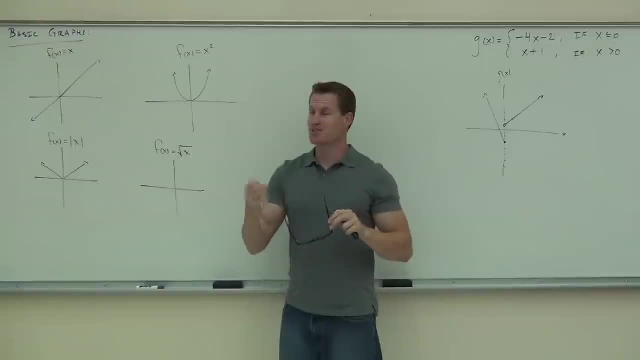 Or you have to have glasses like mine which are like, if I take it off, you're all just blurs, Just every one of you. I see grays and oh, I see orange. I see that one real clear. 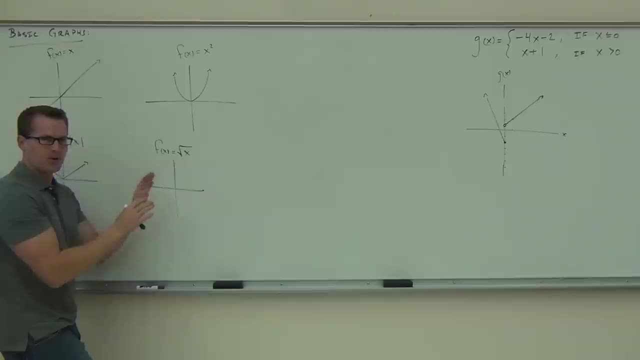 But what this does, it's half a parabola on its side. It's like if you took this one, You make it look like this and erase the bottom half, This kind of curves that way. Look at how the square root kind of goes that way. 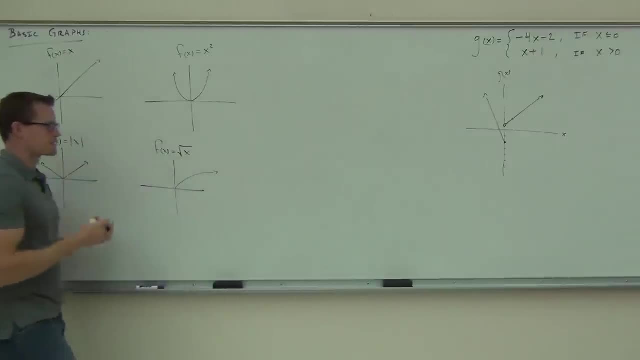 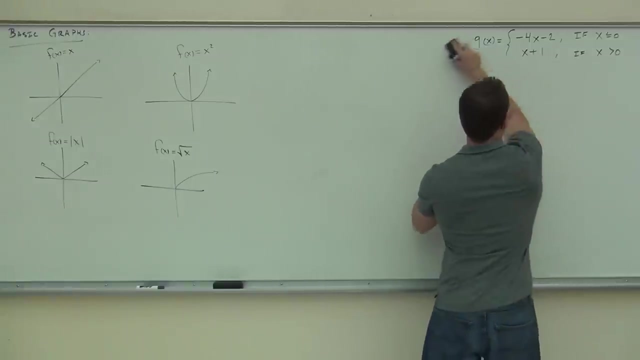 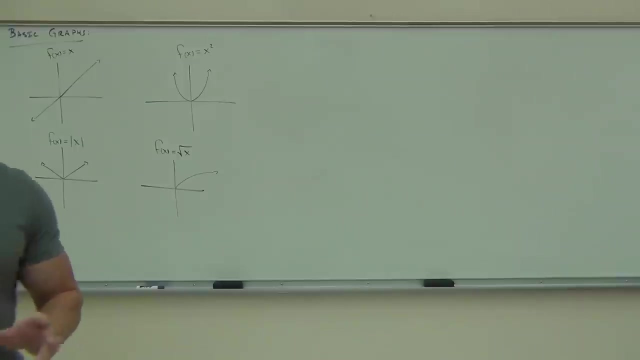 That's what that one looks like, Or something similar to that. I need you to memorize these four shapes. I need you to memorize that if you just have an X or an X plus something or X minus something, a line, you've got a diagonal line. 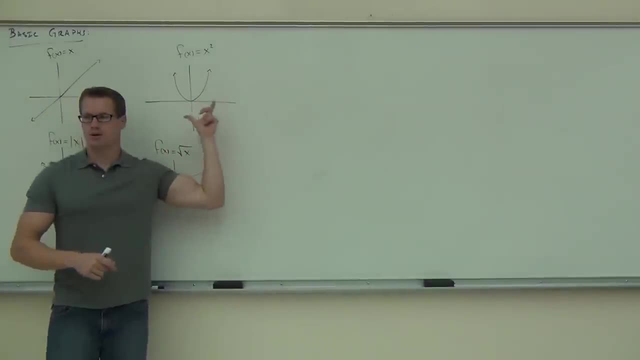 If you have an X squared, ladies and gentlemen, it is always going to look like that. It's going to be a parabola. If you have an absolute value, it is always going to be a V, And if you have a square root, 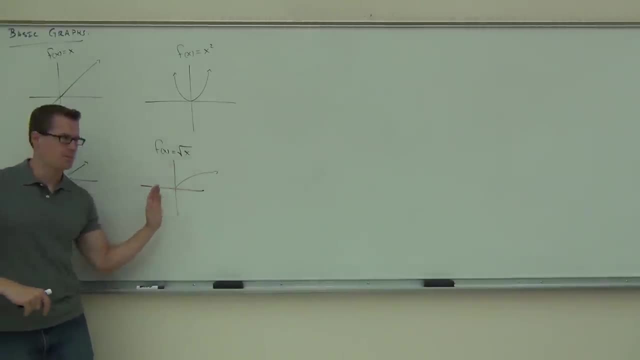 it's always going to be this: half a parabola on its side, that funny-looking shape that we have. that goes like that forever. You with me on this. Now, what we're going to do with this, the reason why I have to have you memorize it. 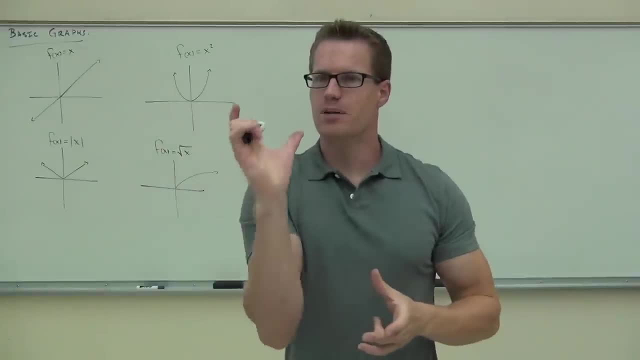 we're going to be able to shift this around, And so, by just understanding the basic shapes of these graphs, we're going to be able to draw a line. We're going to be able to draw a line. We're going to be able to draw a line. 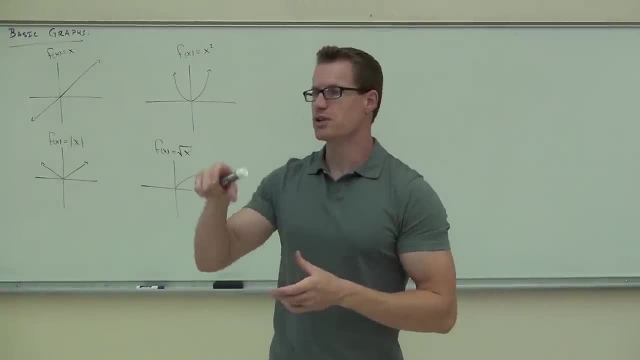 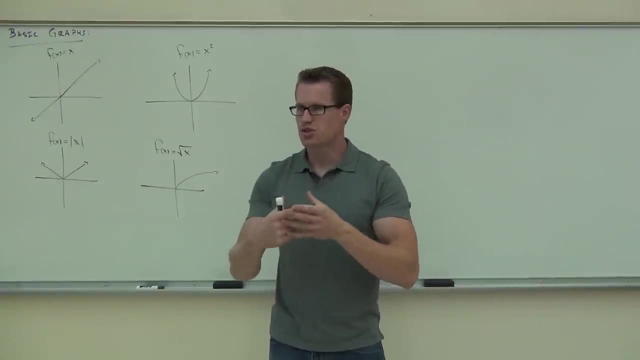 We're going to be able to draw lots of complex things just by doing a little shifting. We don't have to draw tables, We don't really have to do a whole lot of manipulation. We're just going to understand how to translate and shift. 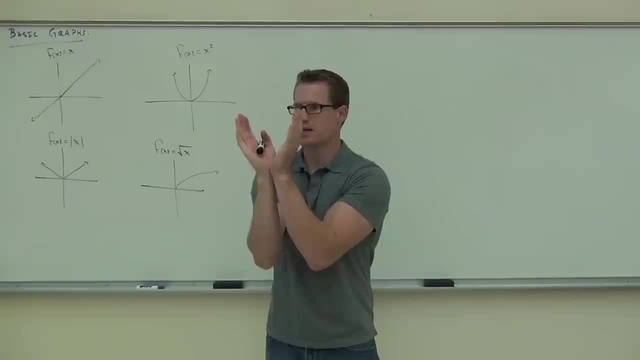 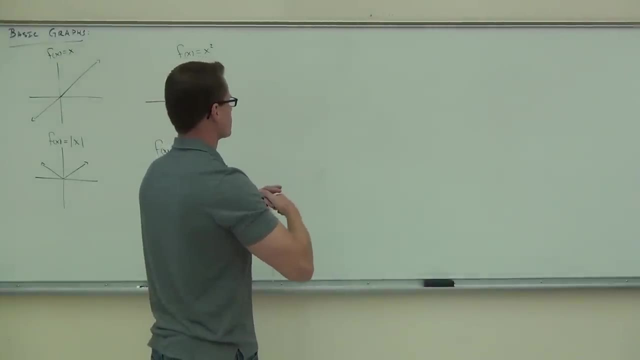 and eventually make smaller and compress and stretch our graphs. The first one we've got to talk about is what we did to this. When I did this on my graph yesterday, I was going to be able to do this. It was two days ago and I added one to the end of it. 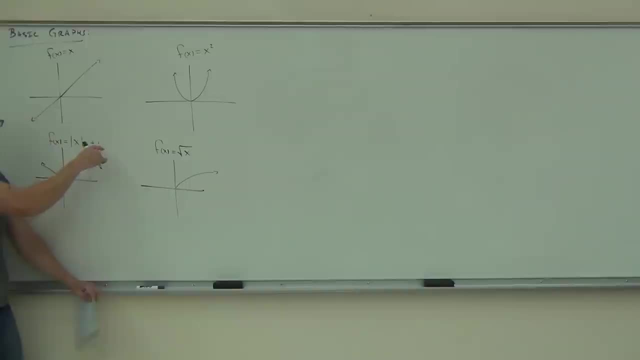 What this said is: okay, you're going to do your whole function right, and then you're going to add one. What did this plus one do to that? It did, yeah. it said: whatever you have, I'm going to add one to it. 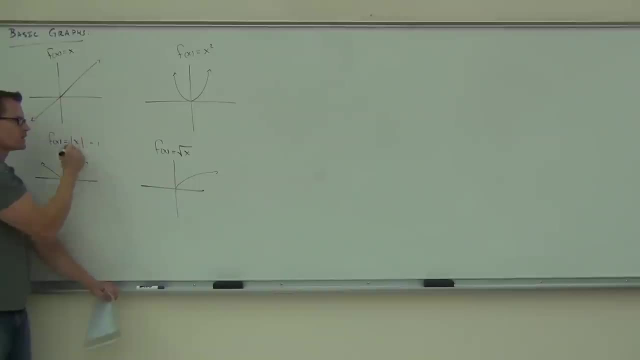 It's going to raise it up one. If I did minus one, what would that have done? Great, yeah, the whole graph just would drop down one unit With me. They have the same shape. This right here is our vertical shift. 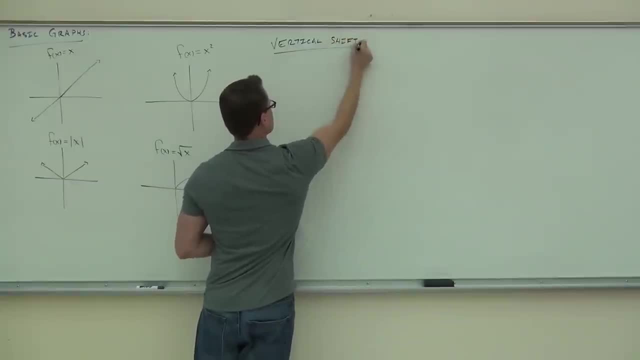 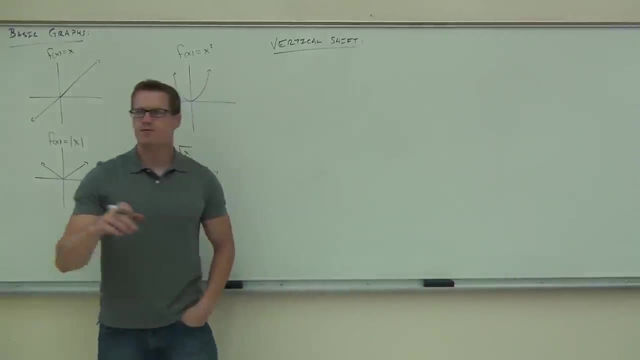 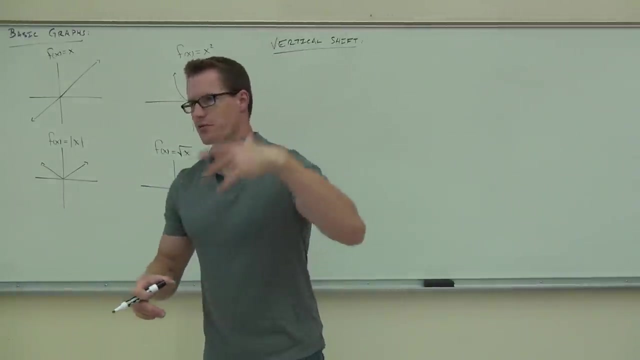 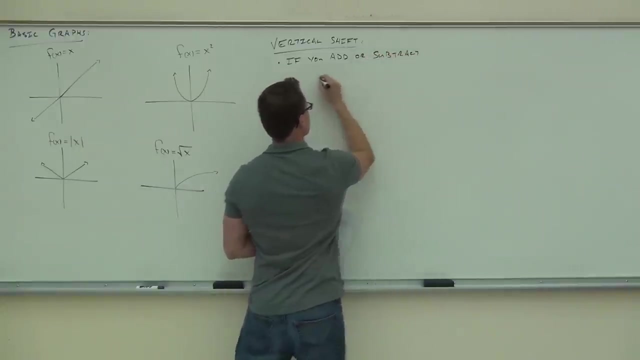 If you add or subtract a number at the end of your function, what that's going to do is shift our graph vertically, either up or down. Here. it will shift it up or down vertically. All right, now, it got to be submitted. My count is neither 1 nor 1.. It's going to be 10,000 or something, so it's coming down 7,000.. It wants to get rid of 16,000.. All right, I'm going to Haas math. 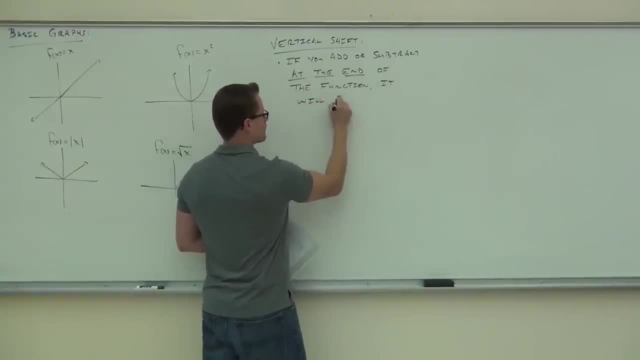 I'm going to place it right here: crazy saga or like 10 million dollars or whatever. I'm going to create a graph out of my room And I'm going to move it up, up and down into the pie chart. 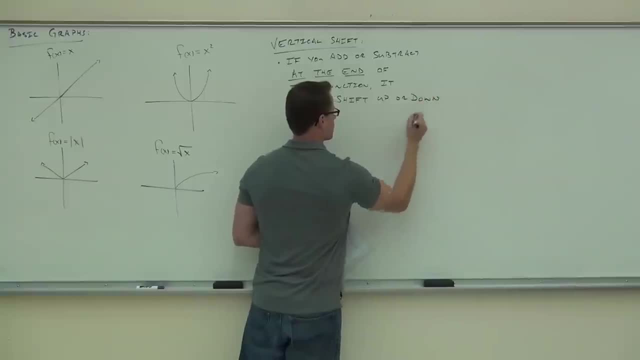 It's going to go hide where I wrote it, So I'm going to hitца Go ahead. I'm going to create a graph of five. All right, Here's the graph in here. By the way, you're going to notice that I've used f of x in every case up here. 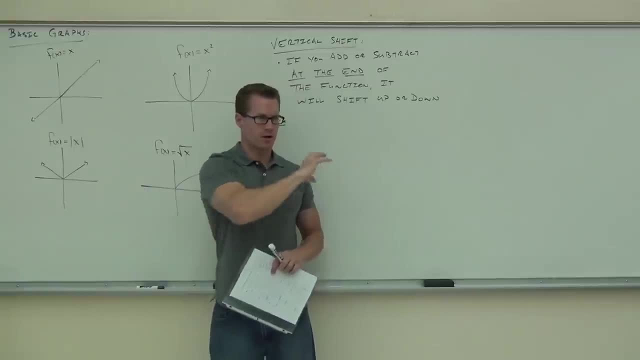 Do you guys see that f of x, What this stands for in our examples for this whole section? f of x stands for one of these basic graph shapes, because if I add one to the end of any of these, all it's going to do is shift it up one. 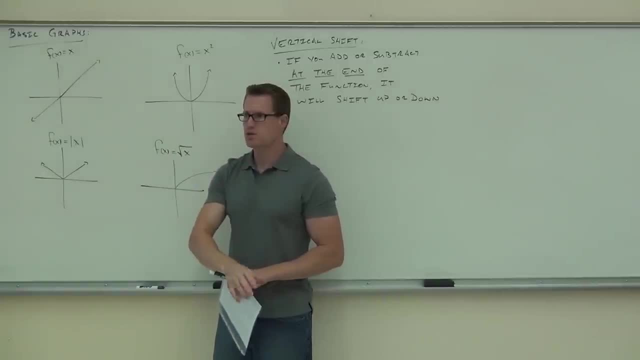 If I subtract three, it's going to shift it down three. Does that make sense? So when I refer to f of x, I mean a basic graph shape. Okie dokie, That's twice today, Okie dokie. So if g of x, our new function is made up of f of x. 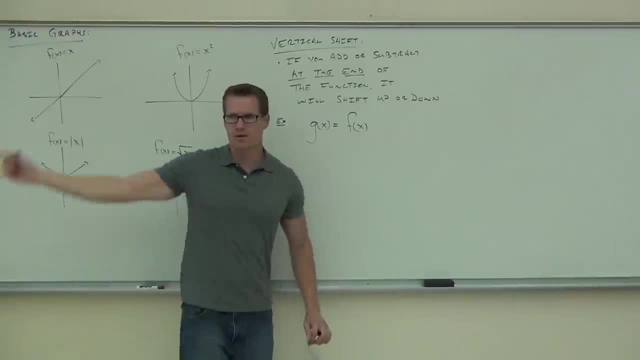 and by f of x. what do I mean by f of x Graph, One of these, One of those right there, If it's made up of a basic graph shape plus k, some number plus k, what's the plus k do here? 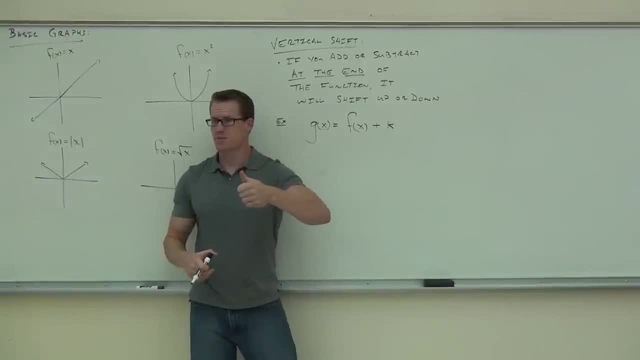 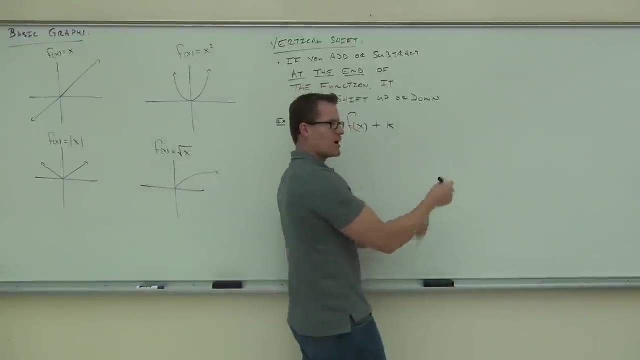 Well, it's going to shift up or down. Good, So in this case it's plus k. Is it going to be up or down? Up, Up, how much? One One, You don't even know. Ok, Yeah, This is shift up k units. 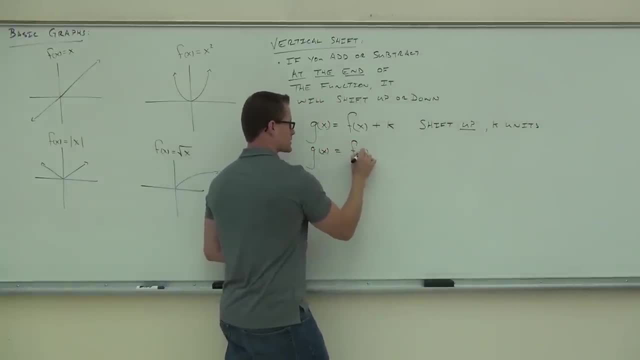 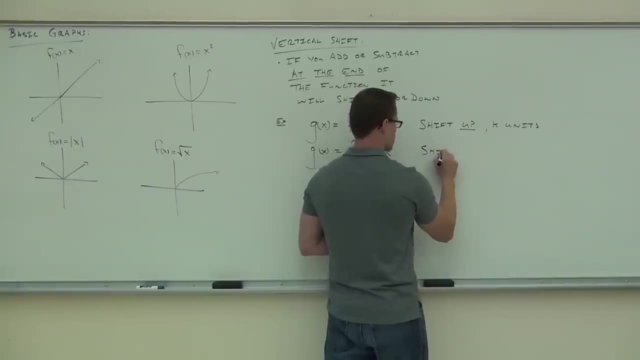 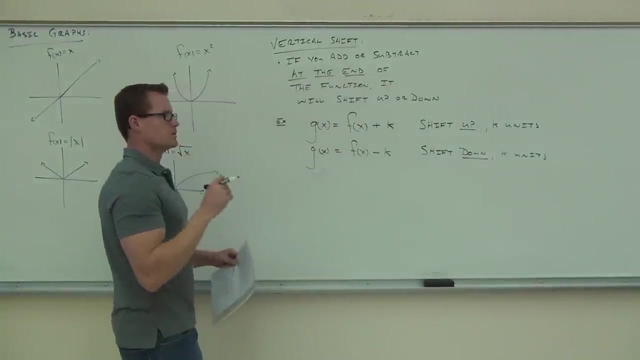 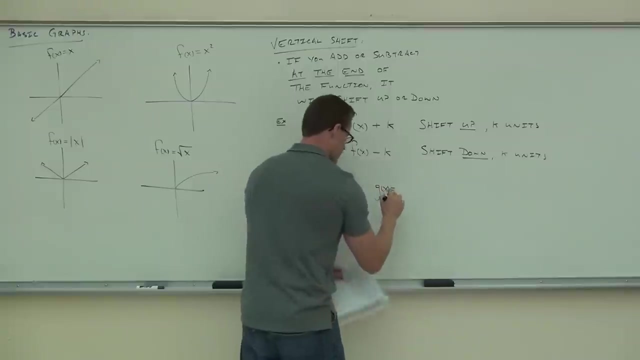 If I did the other way, f of x minus k, well, that's going to be the shift down k units. Let's do a couple examples to really illustrate what happens with this On each of these graphs, for right now I'm going to give you the original. 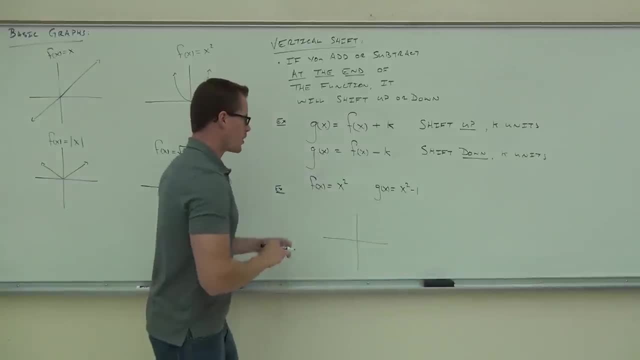 and I'm going to give you the manipulated, the shifted graph. So our first graph: we need to memorize this: f of x equals x squared. What shape is f of x equals x squared? It's on the board, if you don't remember. 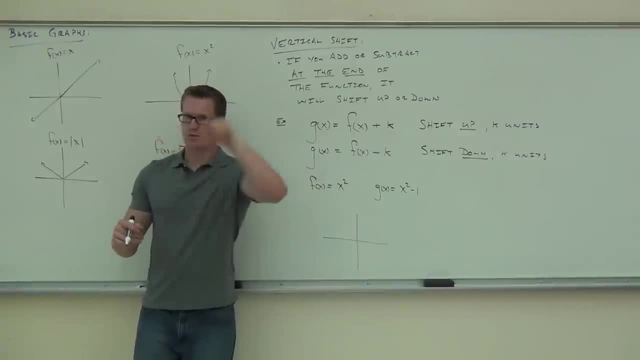 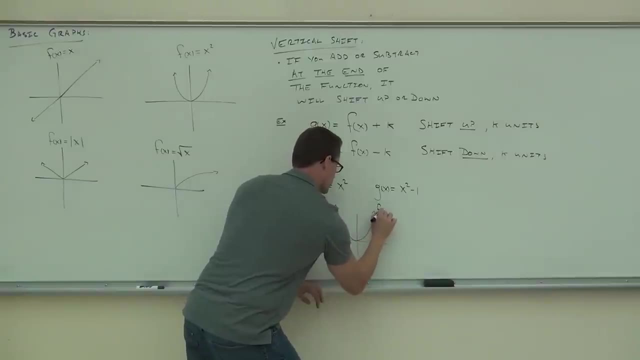 It's: yeah, it's the parabola, It's the u, It starts at 0, 0, and it just goes like this: It's that u, It's that u. So this right here is f of x. 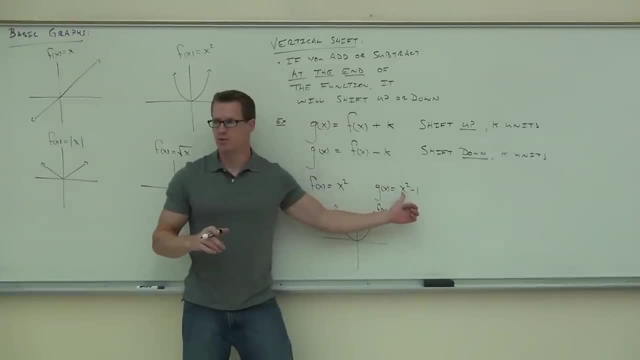 Now what I need you to do is be able to get to here without drawing another table. Notice, we didn't even draw a table for that one. We're memorizing how these graphs look. That makes it easier. We don't have to draw a table. 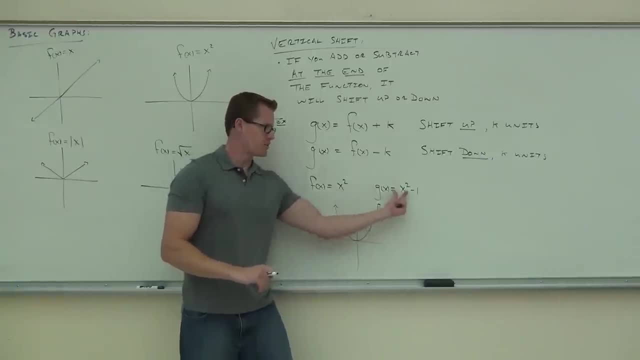 Notice how g of x is simply our basic graph shape, minus 1.. What is that minus 1 going to do for us? in this case, It's going to do 1.. Great, So all you have to do is this: Watch carefully, ok. 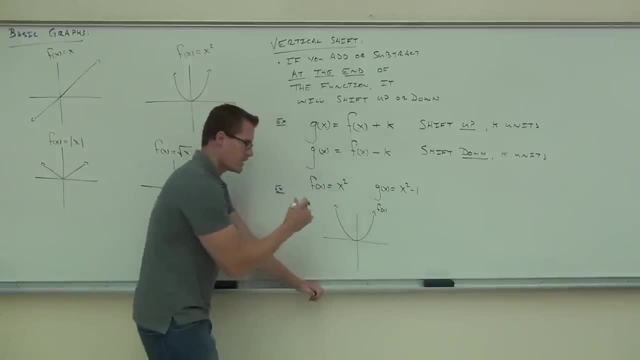 When you're doing your problem, you go: okay, I'm going to think about my graph and I'm going to shift it. what was it up or down again? Down, Down, one spot everywhere. Really, what you've got to think about is just the vertex of this thing. 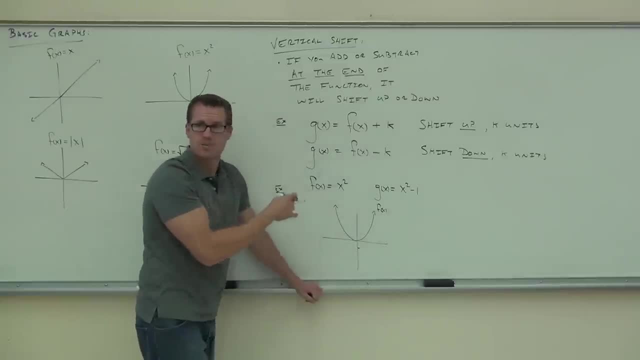 If I shift down the vertex and redraw that graph, it's going to be in the right spot. So what I'm thinking is- here's my original: I need to shift this down one spot. So, right here, I'm going to take this. 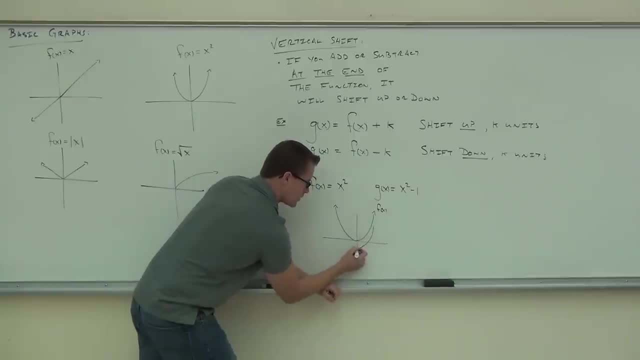 I'm going to shift it from the origin down one. I'm going to redraw my line Or my graph. That's how g of x will go. The original is right here, My basic graph shape that I have on the board. I've shifted everything down one spot. 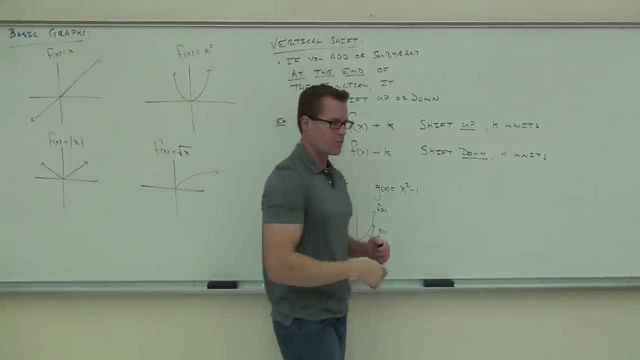 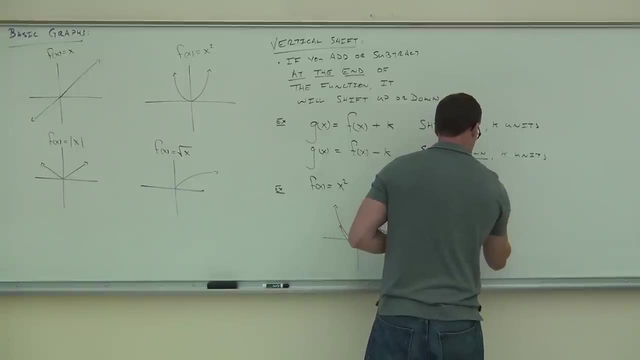 Do you guys have to be okay with that? Okay, Let's try one more. I'll have you do it. I want you to make sure that the square root does not go over the two. okay, Make sure it does not go over the two. 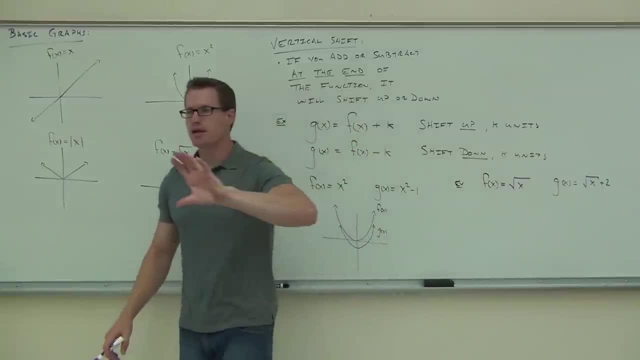 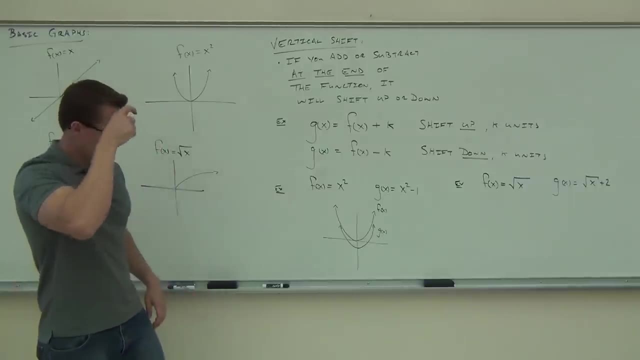 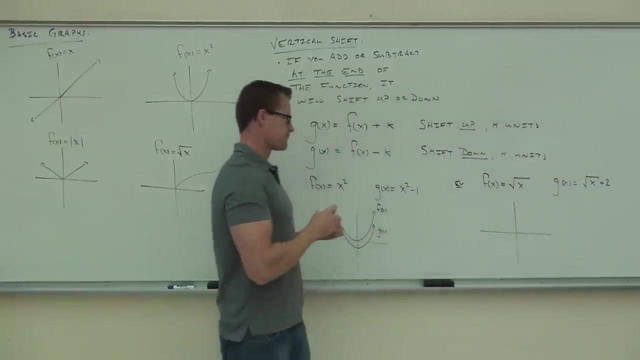 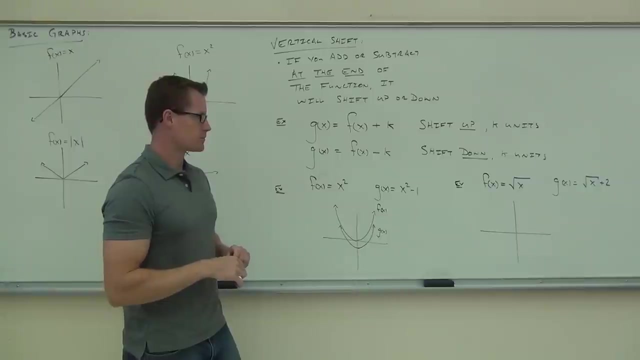 So draw your original, your basic graph shape, and then tell me and show me what happens when I add two to the end of it. okay, Do that on your paper, right? Hopefully you're starting to memorize these shapes. What shape is this? 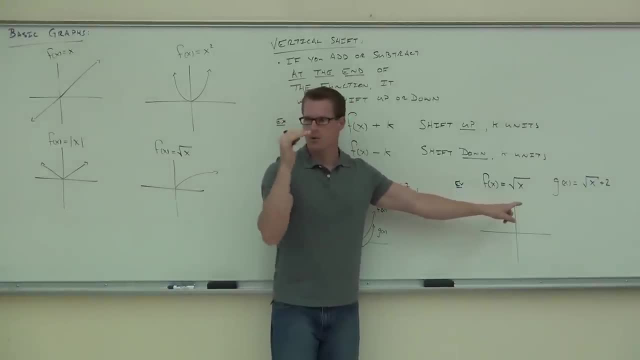 The square root Half-parameter. Yeah, that's that weird one-half parabola on the side. It kind of looks like that from the square root. Okay, So this starts at the origin. the original one just goes like that. 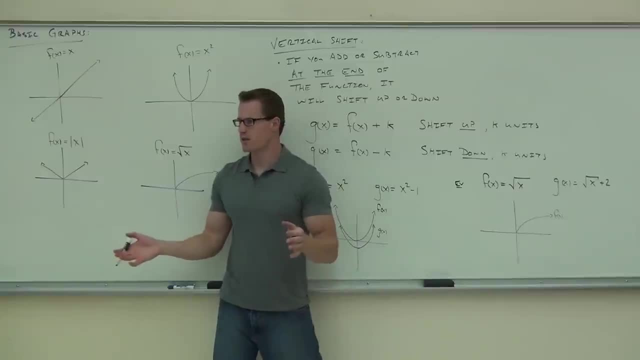 That's f of x. No surprises there, right? You all have that on your paper, right? The next one, g of x, says: I'm taking that and I'm shifting it somehow. Can you tell me what that plus two does to your function? 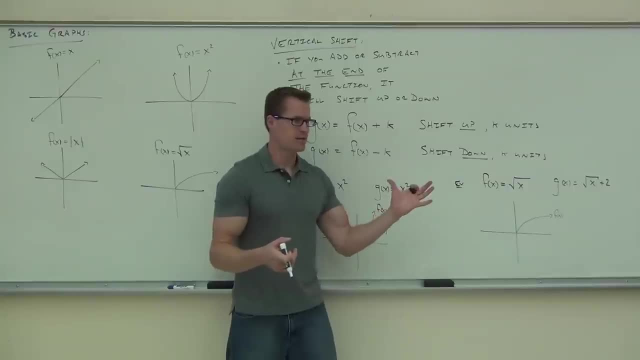 Does it go right or left at all? Right or left? Just taking that, it's moving it up two notches and we're going to redraw the whole thing, You with me, Okay, By the way, do I even need to give this to you at all? 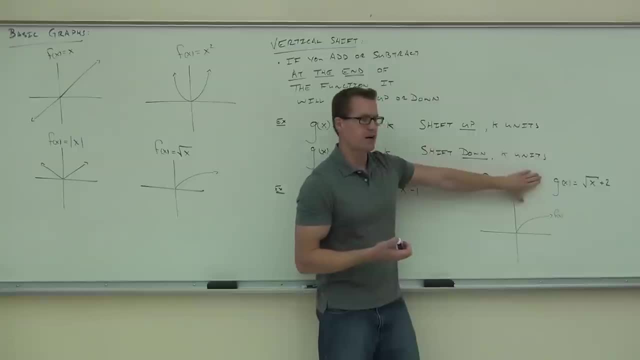 If I just gave you g of x, would you still be able to draw the same thing I'm about to draw? You just take away the original. You say, oh, this would be my original, right there. And then I'm just adding two to that. 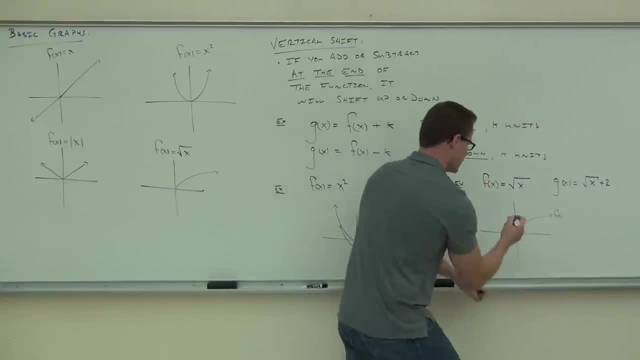 I'm going up In the future, that's what we're going to do. So it says I'm going to start. I have originally started here. That's my basic graph shape. This shifts it up twice. Up two times. Draw the same thing. 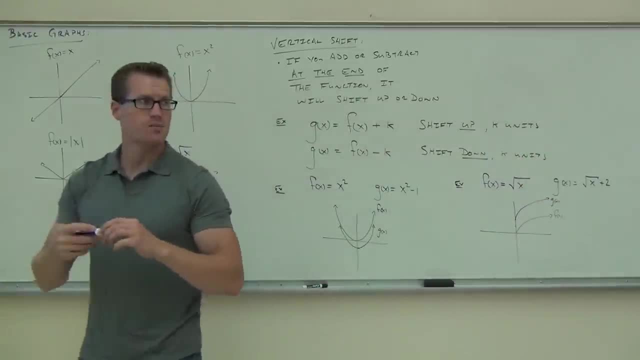 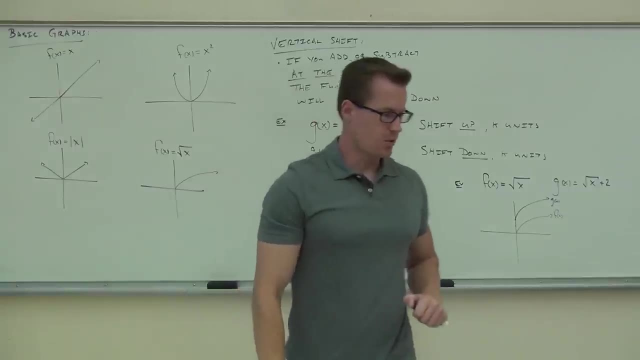 Make sure you label them, because we need to know which one's f of x and which one's g of x. How many of you feel okay with this right now? Good, We're going to stop there today. We're going to talk about a little bit of homework. 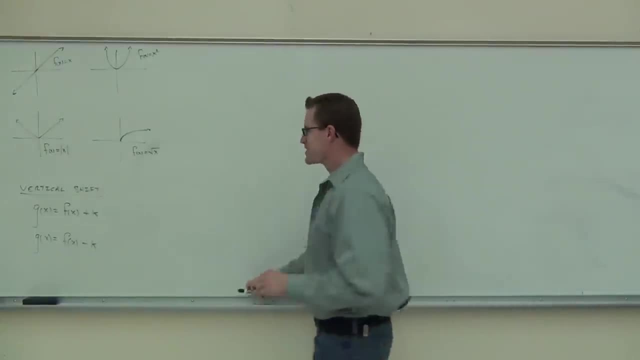 I need to make sure you see something, All right. So yesterday we talked about a couple things. We talked about basic graph shapes. What we have up here, we know our straight line is our x. We know our parabola is our x squared. 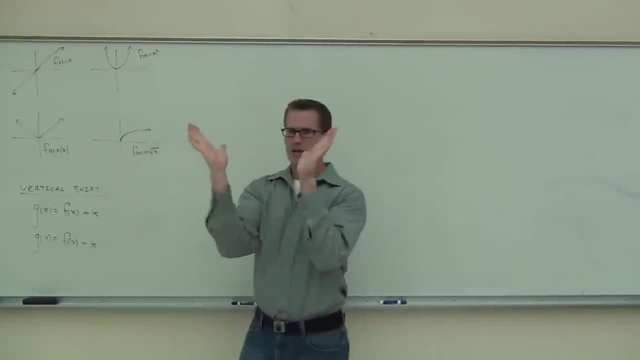 It's kind of like the u shape. We know our v is our absolute value. straight lines Make straight lines, And we have our square root of x, which kind of looks like the square root itself, just kind of curved over. And then we talked about two things. 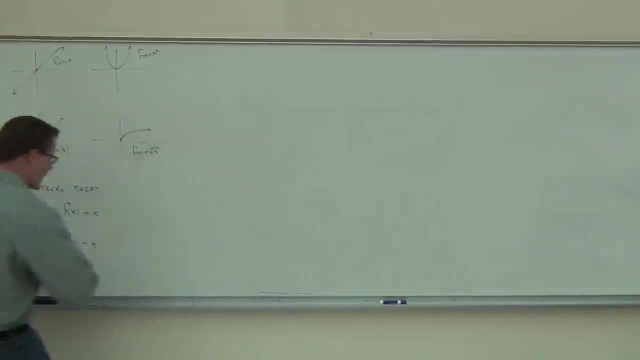 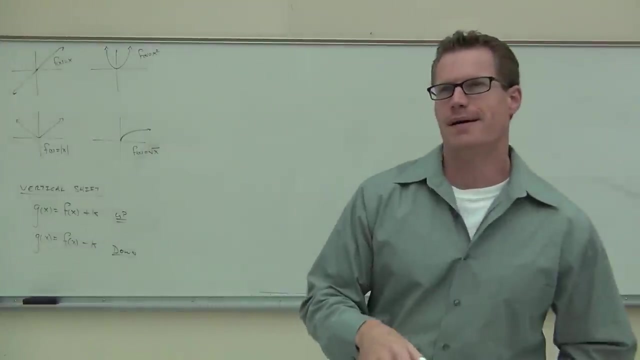 two vertical types of shifts. We have the up, where we're adding k, And we have the minus, where that means we're going down, We're shifting the graph down. Now we did figure out, like a couple days ago, on Monday, we could also do besides a vertical shift. 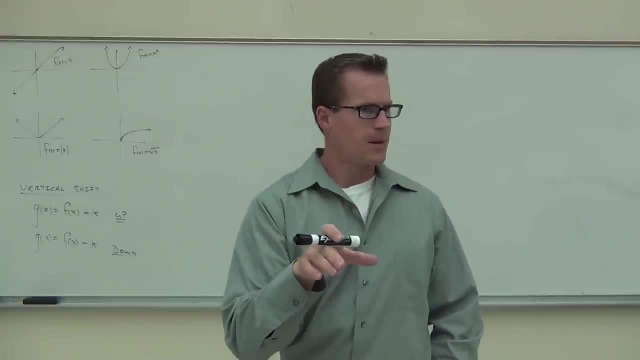 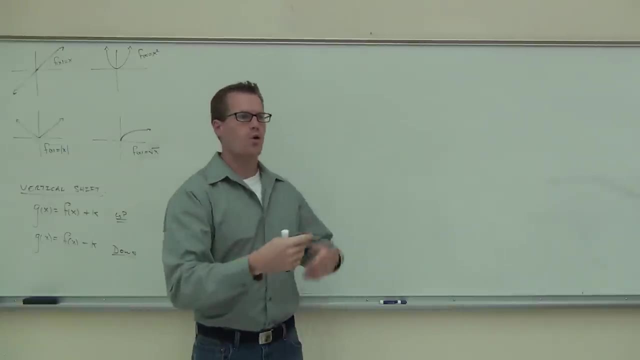 we could do a horizontal shift left and right. Do you remember doing that as well? But it wasn't after one of these functions, It was actually within the function. So when we talk about a horizontal shift, a left right, As a matter of fact, I think it was in this one. 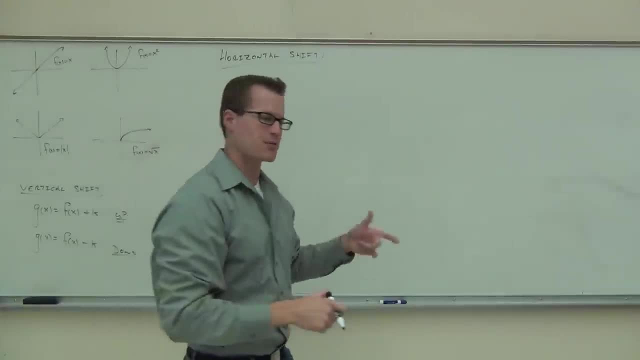 But we had that plus 2 on the inside of our square root. If you remember back from your notes on Monday, that's what we had. Well, here's the deal. if we add or subtract from the back end of a function like this or like this, sure, 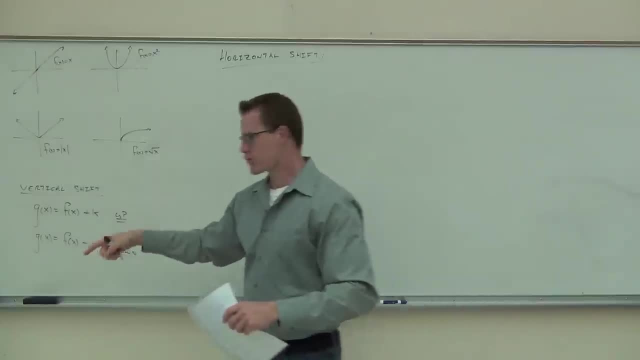 it's going to shift it up or down, Because what's happening is you're doing one of the original functions, like f of x, and then you're tacking numbers onto it And what that's doing is raising the value or lowering the value. 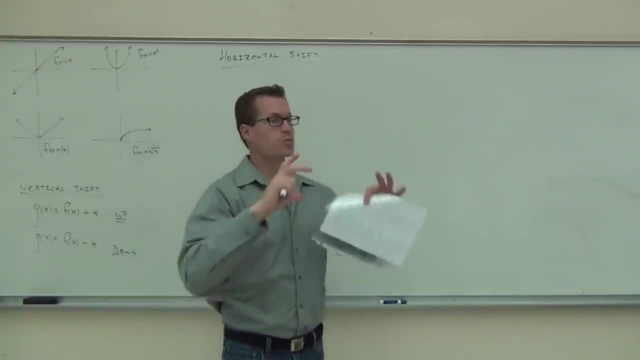 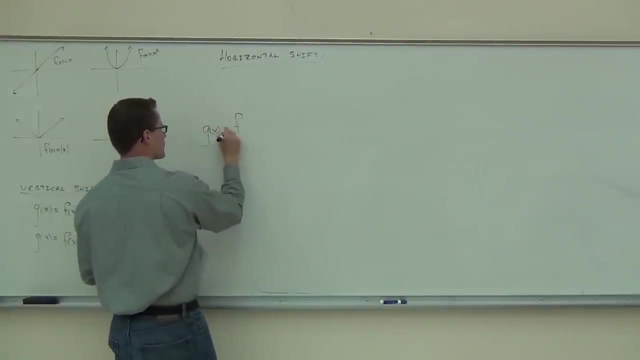 That's moving it up or down. However, if we add or subtract within the function- and here's how that looks, by the way, It wouldn't be. It wouldn't be like that, right? Because that again, that's a vertical shift. 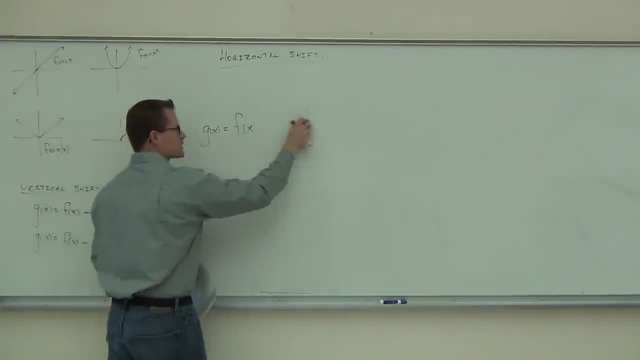 We already covered that. If it's within the function, it looks like this: Plus or minus k in there, And you know what I'll use h, so we get a different letter going on K. we'll leave that for the vertical. 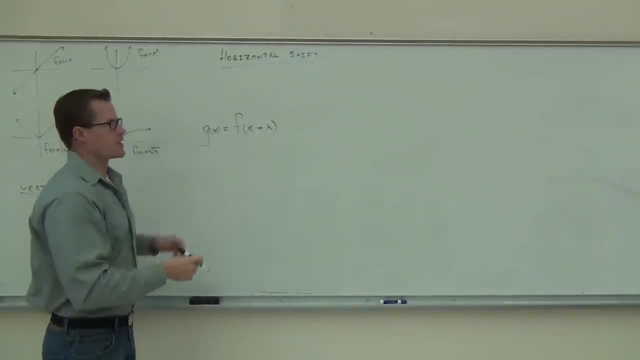 But that would be within the function. So when we looked at this the first time, we said, all right, what is this actually doing? If we looked at our square root of x from last time, we said the square root of x plus 2,. 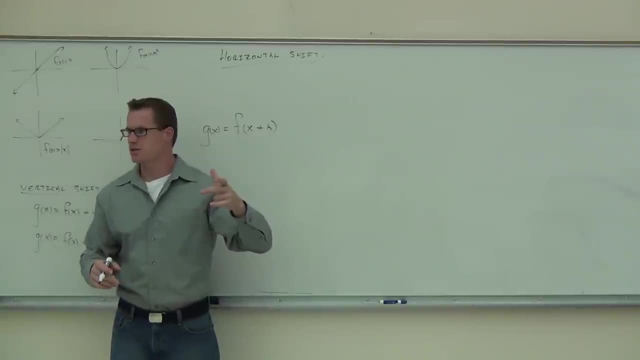 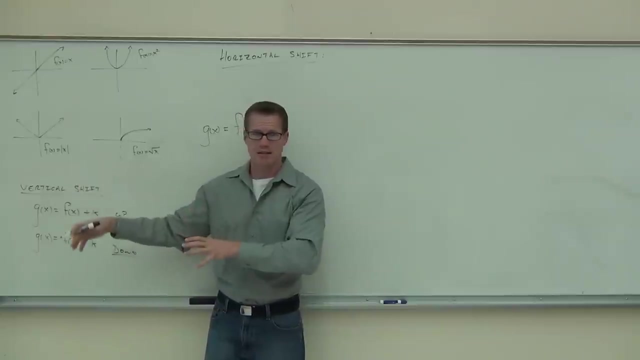 what this is doing. and this is going to seem kind of backwards to you a little bit, because when we did this, our vertical shift and if you add k, it makes sense that it goes up, right, If you subtract k, it makes sense that it goes down. 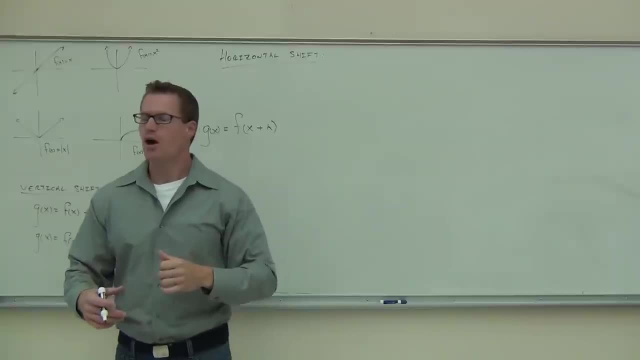 If you add h within the function, a lot of people are going to think: oh, you know what, If I add h, it goes to the right. That would actually kind of logically make sense, right, But it's kind of backwards to that. 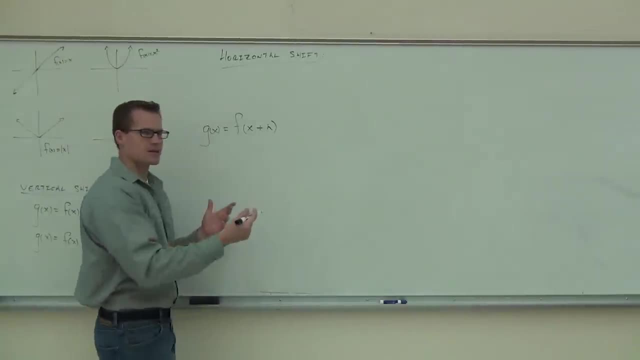 And here's why What this is doing. if you think about this like a timeline, you think of a timeline with like zero in the middle. Our timeline has zero in the middle, actually right, Because we have ad and bc, We have before and we have after. 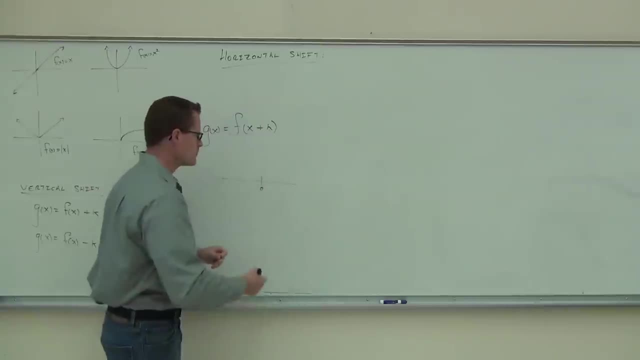 And this is kind of like a timeline for us. We have a zero right in the middle. If you think of this as a timeline, what this is doing is speeding up where your graph starts, So this would be slowing down where your graph starts. 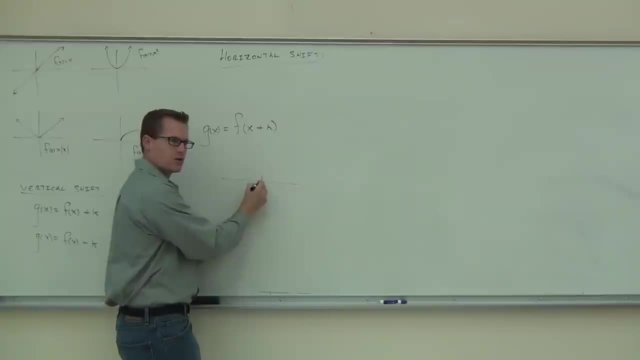 Does that make sense? So, like if you were originally starting at zero and were subtracting, you're starting later, and you're starting later If you're adding to it, you're actually starting earlier. You're making that graph start sooner. That means that this plus h, it isn't a shift to the right. 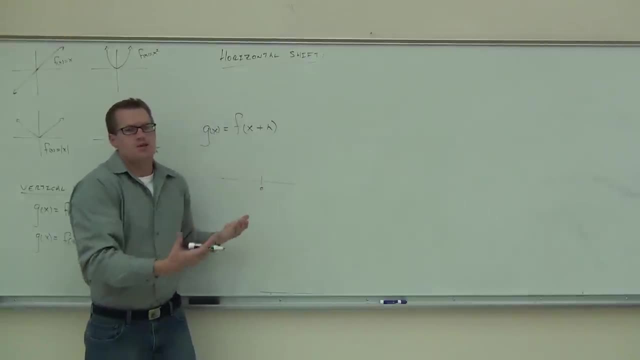 It's actually a shift to the left. If you think about it like a timeline, that should make sense to you, Does that? can you follow that? So it's starting our graph sooner. So a horizontal shift, that's a shift to the left or the right. 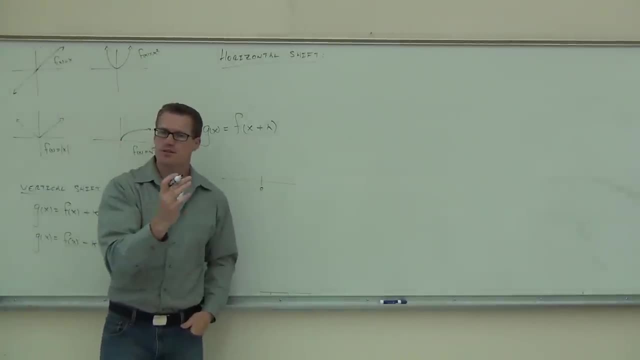 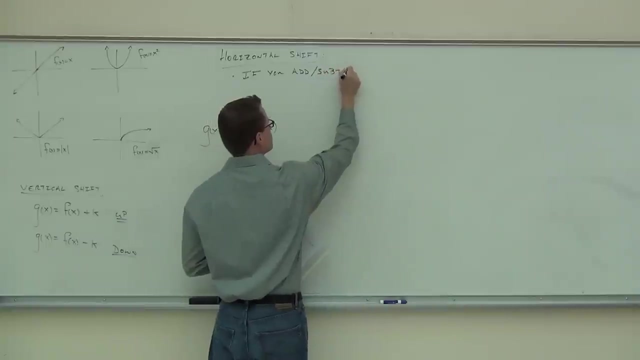 This happens when we add something within the function. Plus is going to go to the left and minus is going to go to the right, And that's the way this works. So horizontal shift if you add or subtract within the function. If you add or subtract within the function. 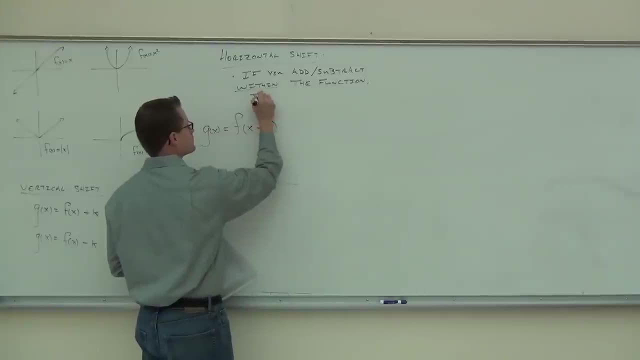 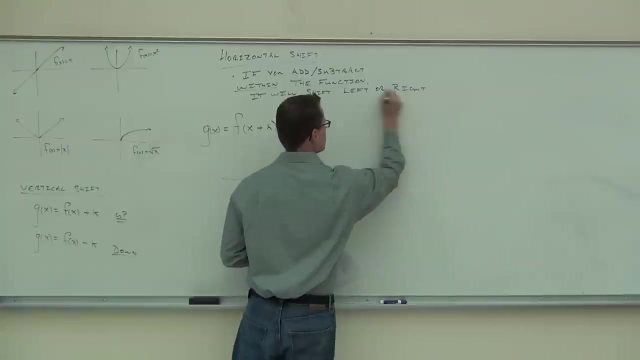 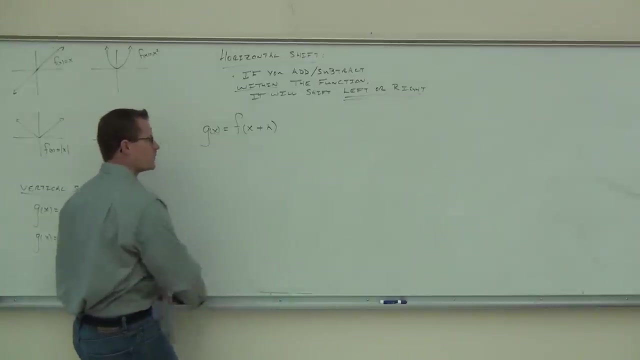 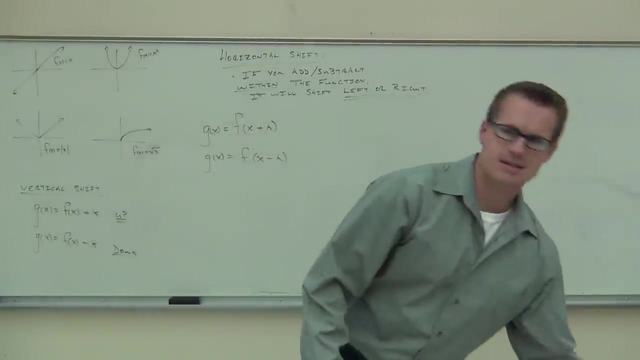 it will shift left or right. And again, how do you tell? Well, it's either going to be f of x plus h, So you say it's within that the parentheses, Or f of x minus h Last time, if you didn't catch this the first time. 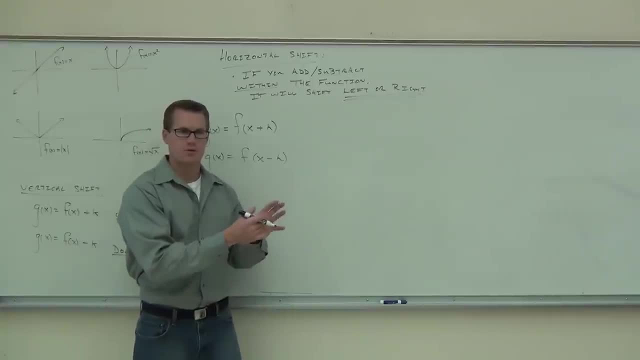 what this does is it speeds up or it slows down your function. So if you're adding h to it, what that's doing is saying: oh okay, I'm going to start this function a little bit sooner. This is moving it to the left. 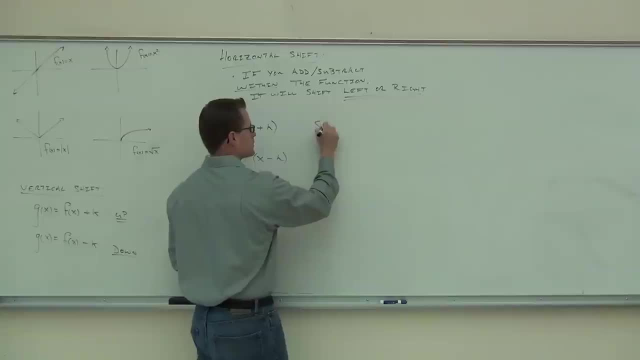 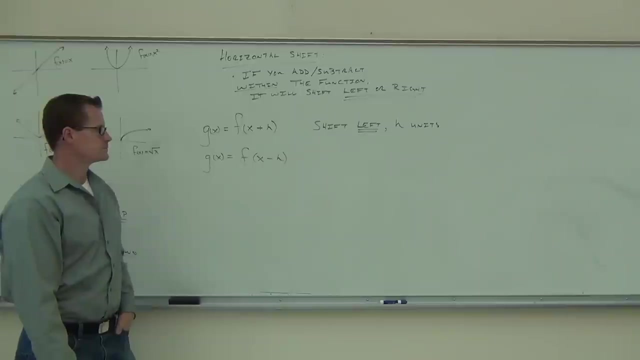 So this is a shift left of h. It's moving it to the right, So it's going to be a shift left of h units. Make sure you have that down, okay. The plus means left Minus h. This says I'm taking- I'm kind of like I'm taking time away. 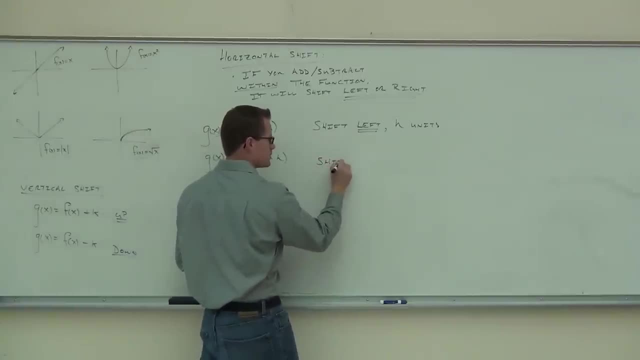 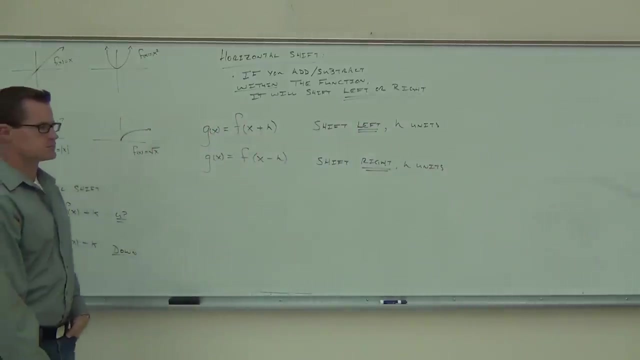 starting later. This is going to be a shift right: Eight units. If you really want to think about it a different way, if the whole timeline thing doesn't make sense to you, here's really what you're doing mathematically: You're taking an original number. 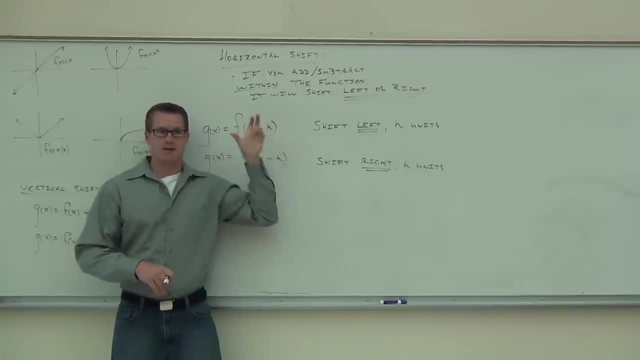 that you would normally plug in. you're adding something to it, making that value bigger, right? You're plugging that in. That means that this is going to start the same height only sooner, For instance, if you take out. let's do an example here. 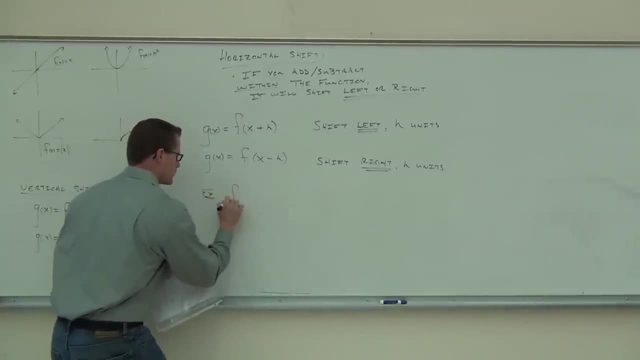 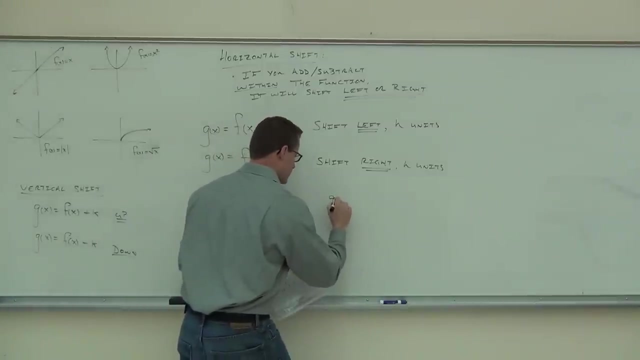 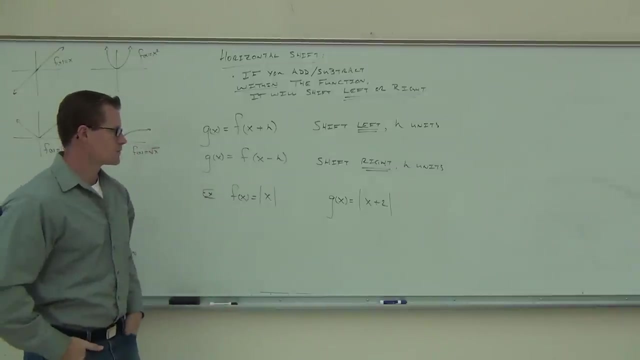 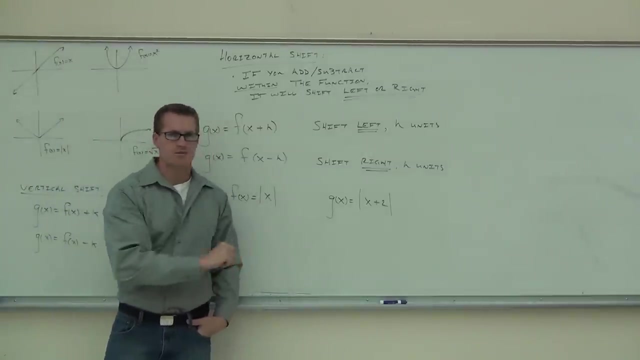 If you want to look at this one, What we're going to do. I'm going to show you this graph and we're going to graph this first, before the shift. I'll show you why this actually happens. I'll explain to you why that plays. 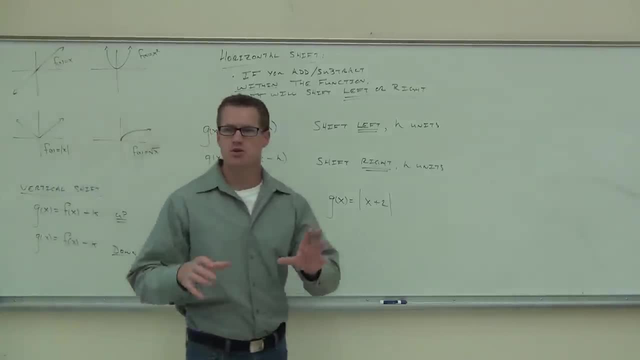 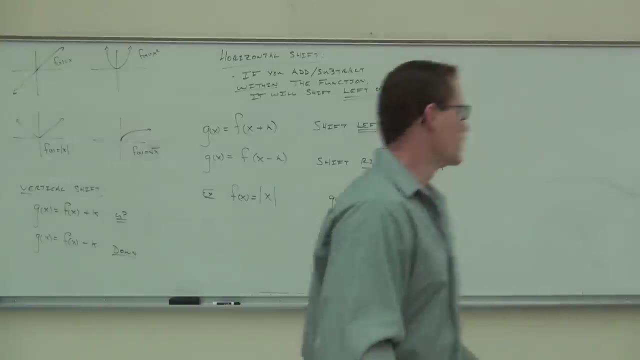 So you're going to have two plus two. Plus two means two to the left. So first thing I want you to identify: is the plus two within the function or after the function? What do you think If it's within the parentheses or within the absolute value? that's within the function? 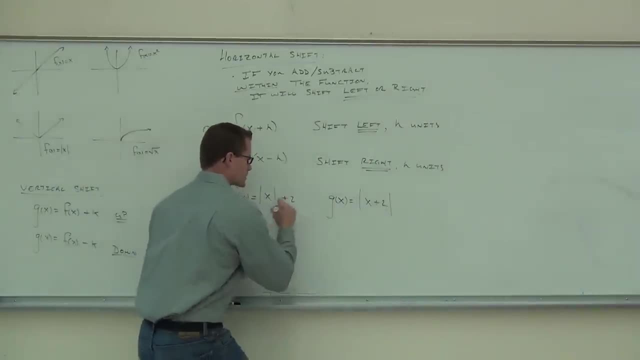 So here, this one is different than say: if I would have done this, Check this one out. Do you see the difference where the two is That two? what would this two be? That would be a sure. This two is actually within the function. 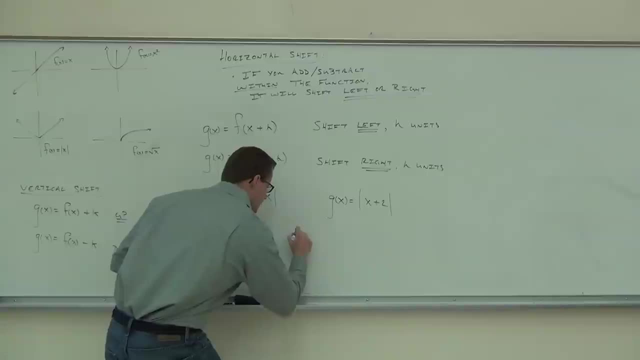 That's going to be a shift to either left or right. We're going to determine that these First thing we've got to know is our original, our basic graph shape. What is the basic graph shape up here? I think it's on the board as well. What is that one V So? 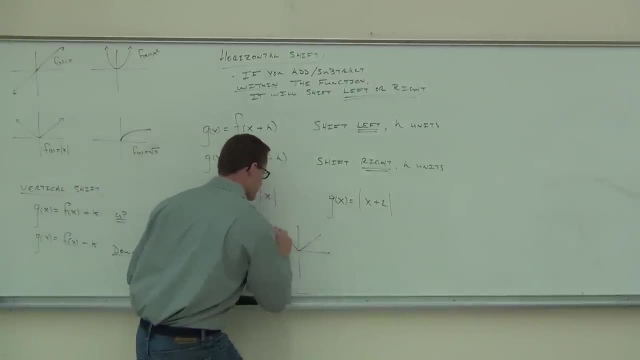 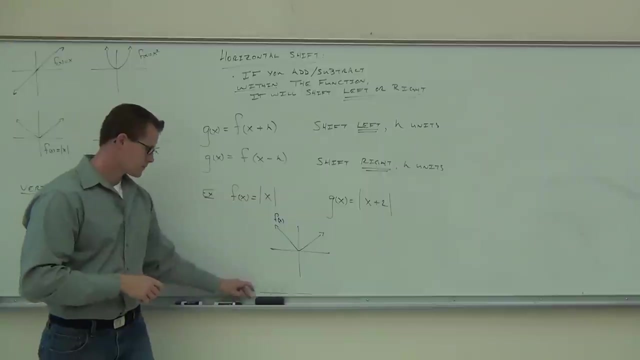 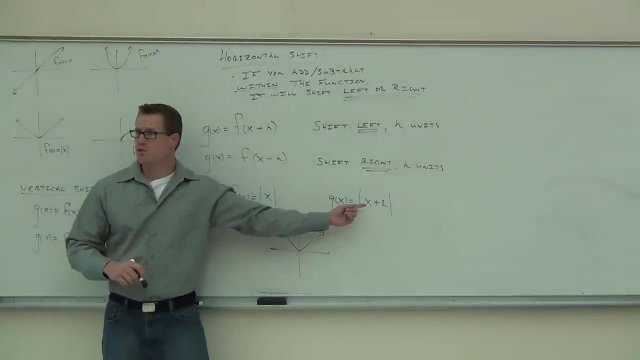 we're going to draw the V And I'll make sure I label that F of X. Let's see this one. Where should this one move? Should this move to the right? I know it's horizontal, so it's either left or right. Is it going to move to the right or to the left? What do you think? 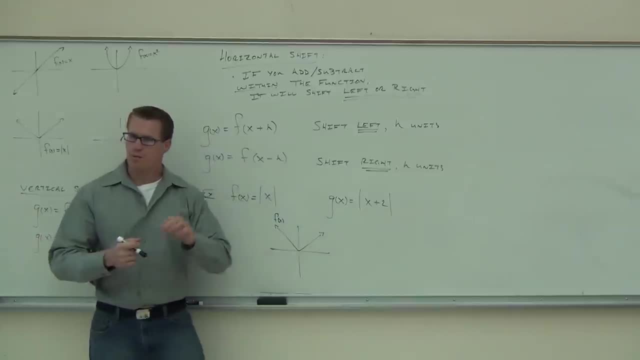 Left, Definitely to the left. How many spots? Two. So remember, we can think about the vertex here. If we're thinking about our origin as the vertex, we're going to move this left two spots and redraw it from that point. Here's how you can think about why this thing moves. 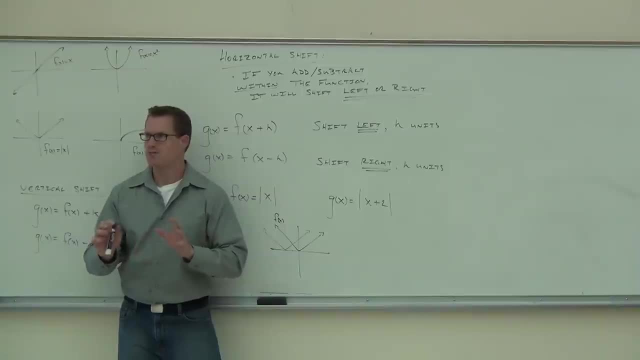 to the left and not the right. Are you ready for it? Yep, Or I could just put this home. Let's see if I can imagine my favorite picture. I think it's so pretty: Beep, beep. Okay, Now what do you think? 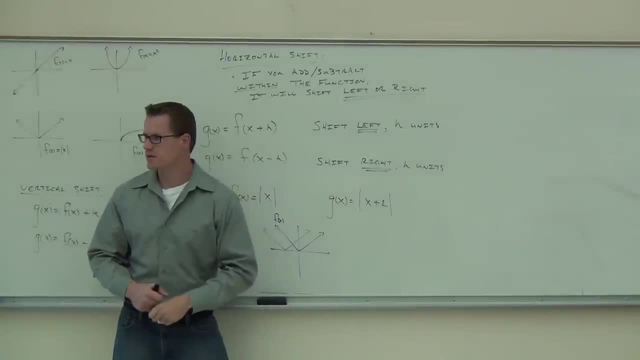 That's a good one. Yeah, that's a good one. Okay, so look, when you're looking at this function, you're looking at some of your information, right? Yeah? So if you want to take some of these things and detailed them and these things and these, 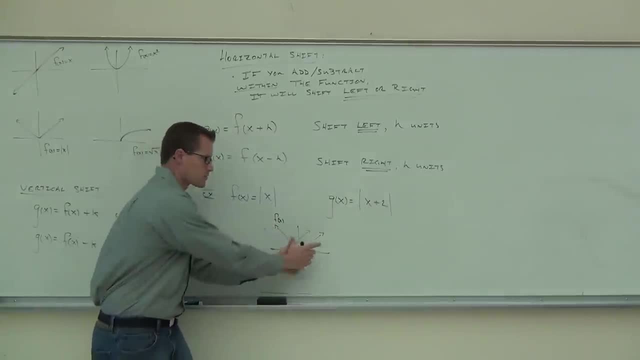 stuff. you have to see them. Okay, Yeah, yeah, at the same height. So what this says is: this graph is starting sooner. I would normally plug in zero to get out zero for this one, right, But in order to get out the same height. 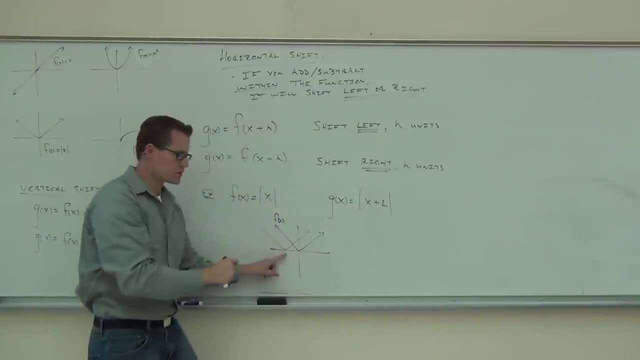 I'm plugging in negative two, That's two spaces to the left, So to get the same height that I would normally get for this function, I'm having to plug in two spaces less than that In order to get the same height out of this function. 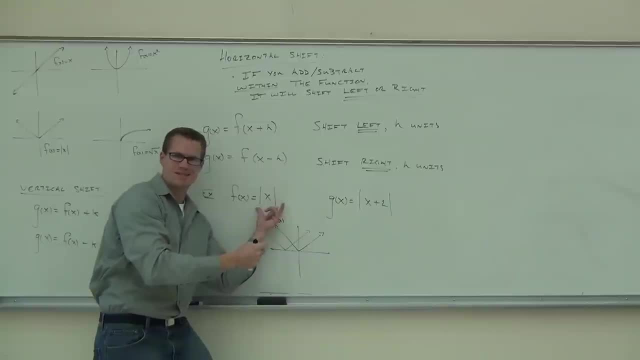 that I got from this function. I'm having to plug in two spaces to the left of that. Does that make sense to you? So to get out of zero I plug in zero, but to get out of zero here I need negative two. 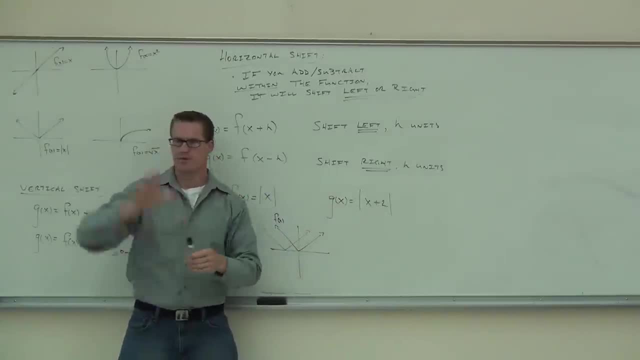 That means I moved my entire graph two spaces to the left. How many people understood that? Okay, good, So this is one of the reasons why plus means to the left if we're horizontally shifting, or minus means to the right, Even though it looks kind of backwards. 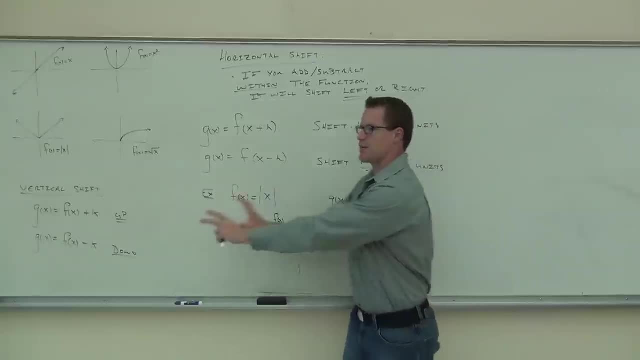 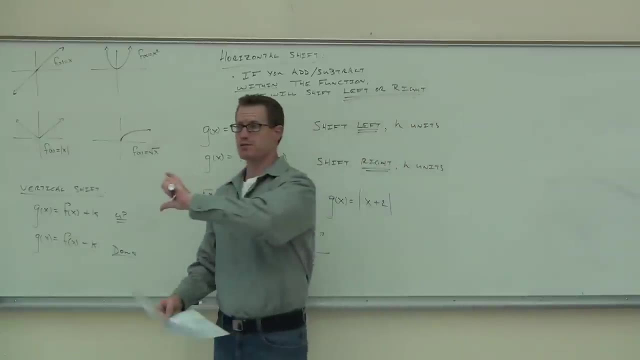 it does make sense mathematically, because it's saying: I'm starting my graph sooner rather than later. That's what this is doing. Now one question: we've done vertical shifts, we've done horizontal shifts, But we haven't done them at the same time. 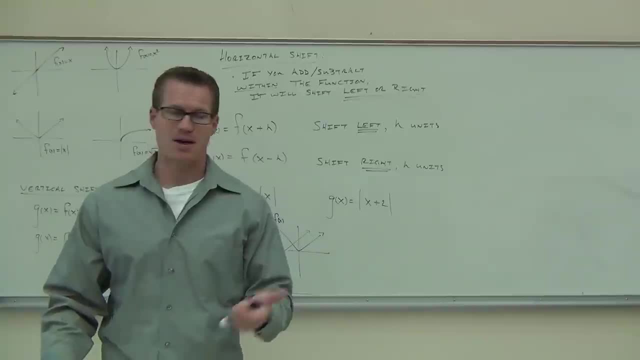 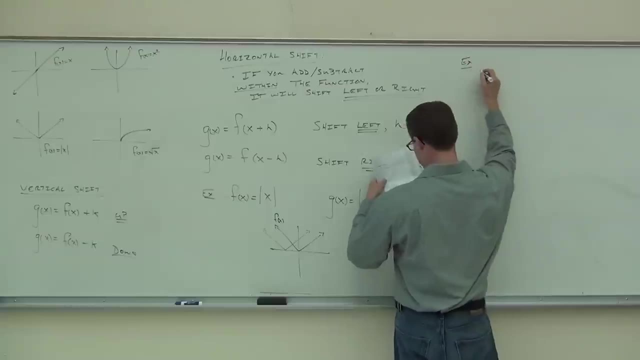 Do you suppose we can do these things at the same time? Yeah, we may as well, right, Let's see how that looks. If you need a title for this, let's call this combining shifts. Just be careful how you say it. 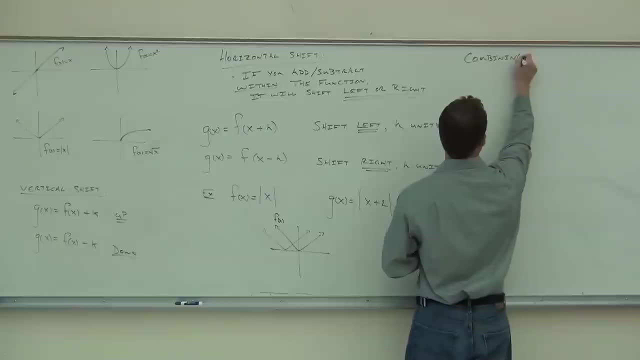 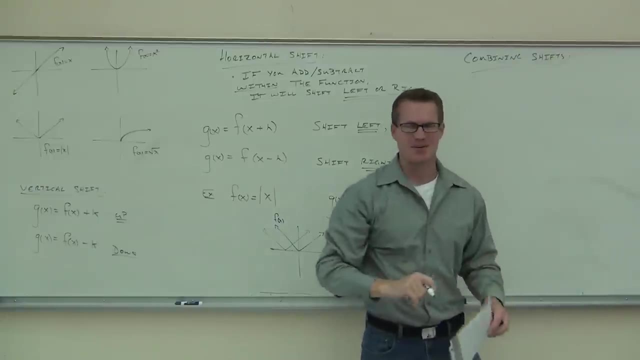 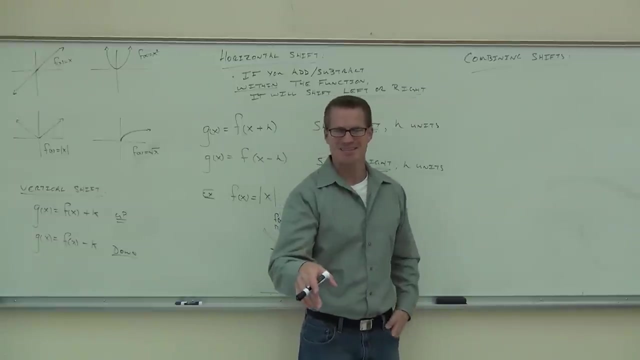 Okay, This is one of my favorite sections because of that word. It's just kind of fun. What a load of shift Square. Have I used that one in here before? No, that's a new one. I'd say I'm not taking any shift from you guys, right. 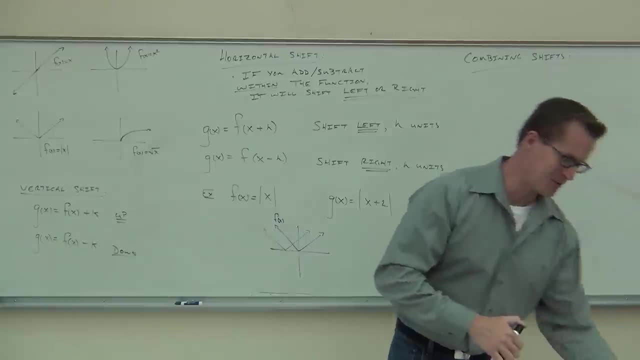 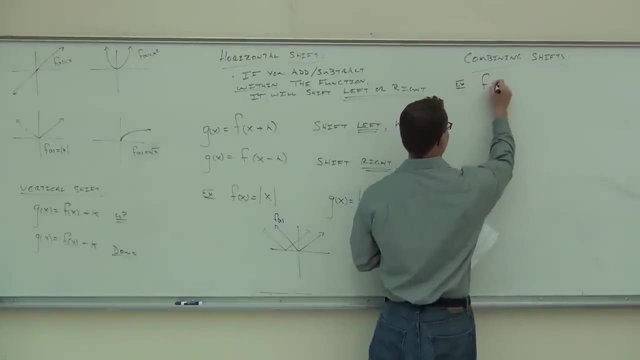 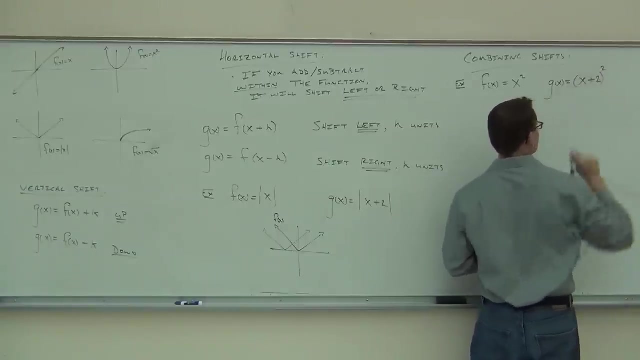 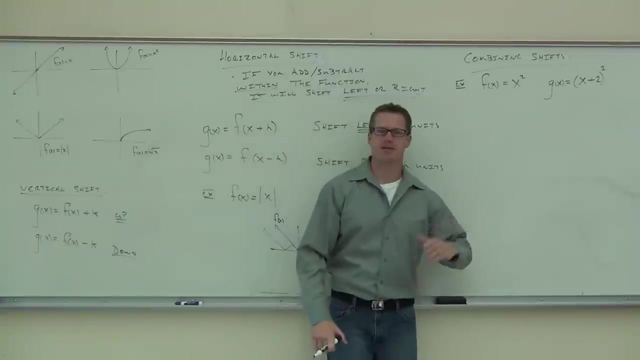 I said that one already Big load of shift. this class is Okay. Okay, All right. ladies and gentlemen, I need you to look at the board here real quick. Can you please tell me what my basic graph shape is? Parabolas. 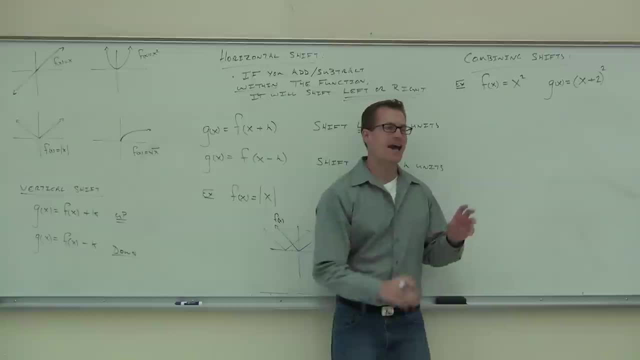 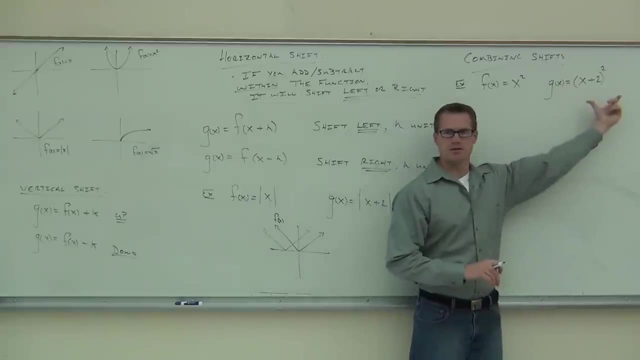 Parabolas, sure, Okay, A basic graph shape is a square. Now another question I have is: if I hadn't given you this- just pretend f of x isn't there- could you have said the basic graph shape just by looking at this? 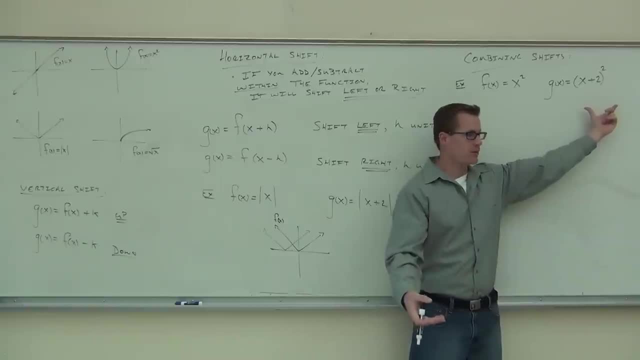 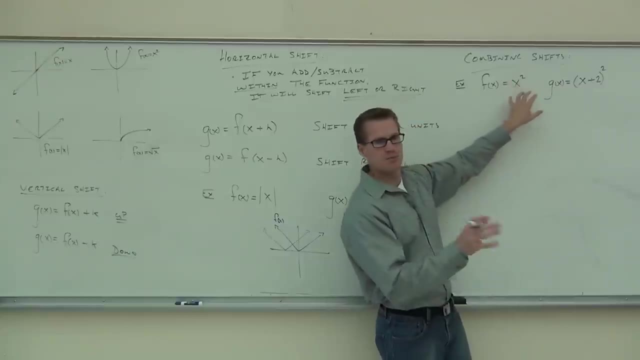 Yeah, Yeah. Any time you get that square, that's automatically a parabola. Are you with me on this? So for sure, that's going to be a parabola, no problem. So even if I don't give you the basic graph shape, 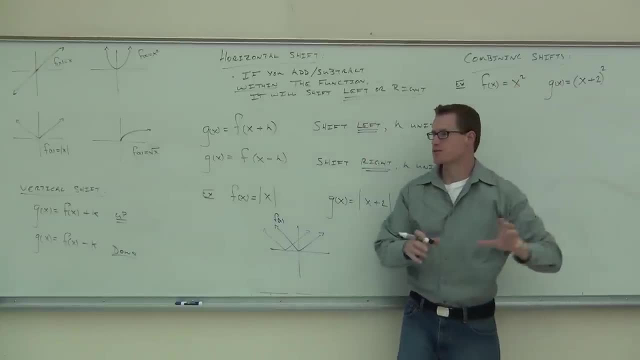 like a standalone item. you could really just look over there and tell that that's going to be a parabola. okay, Now if I left it just like this one, I'm going to set that to 10.. All right, 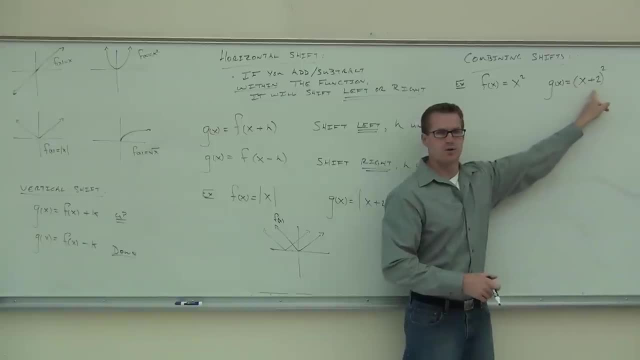 Just like this one. what would this do? Is this a vertical or a horizontal shift? Horizontal? Why horizontal? Tell me. It's in the parentheses. Very good, It's in the parentheses. So this is going to be to the left or to the right? 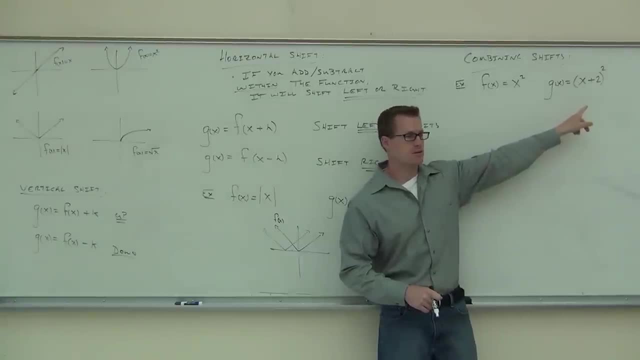 Which one Left? That's definitely to the left. How many spots? Two, Okay. What did I just put on there? I know it says minus one, but I mean, what is that according to the math that we're talking about? 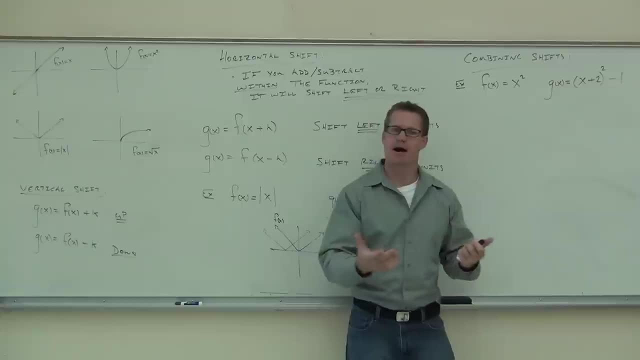 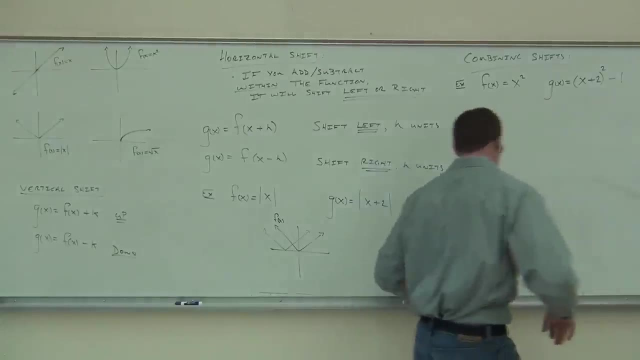 Vertical or vertical shift? Yeah, it's a vertical shift, So we can't actually combine our shifts. We just need to identify what these things are individually. Now, typically, the way that I show this is I like to circle the parts and identify each one before we go any further. 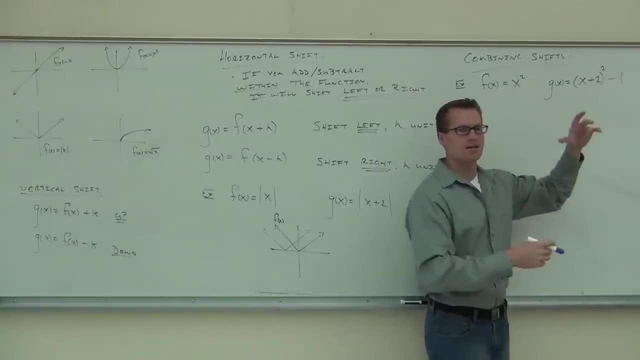 So when we look at this, we're going to be looking from the left to the right- identify each little piece. We know anything added or subtracted at the very end of our function is a vertical shift. That's why we start there. 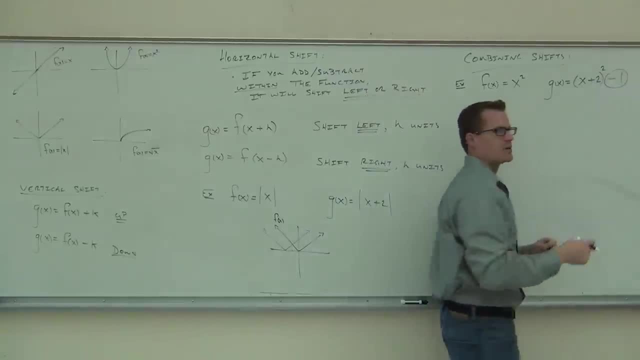 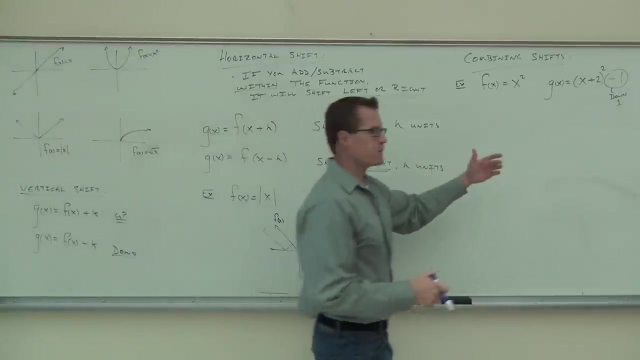 So we go over here, we circle this thing and you've all told me that this is going to be a vertical shift, This is going to be down one unit, Down one. Then we move ourselves to the right and we notice we have an X squared. 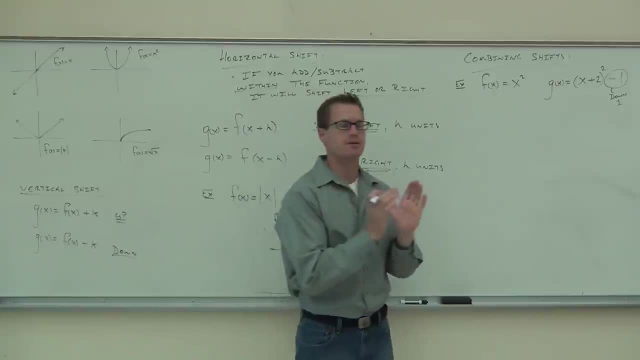 That X squared tells me. I'm for sure going to draw a parabola still, That's what that says. Then we look for anything inside the parentheses. So if we move from the right to the left, we move from the right to the left. 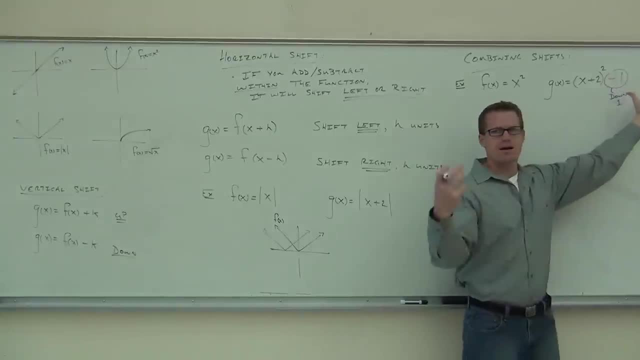 we identify our vertical shifts first. So we go: anything added or subtracted that's going to be up or down. Plus means up, Minus means down. So here we mean minus one or down one. We look at the type of graph that we have. 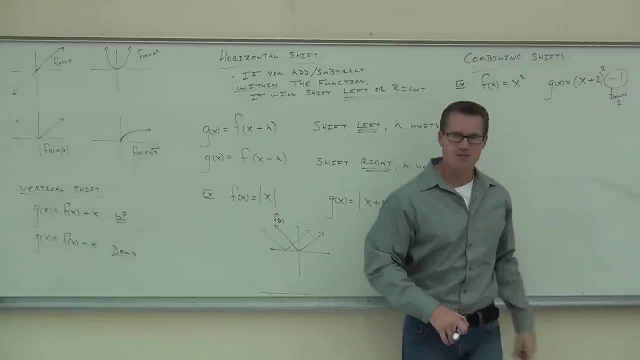 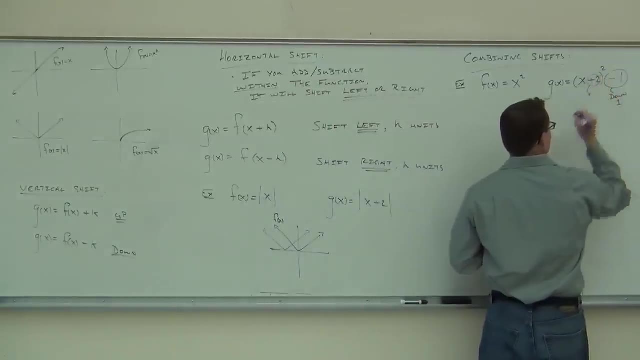 We have a basic graph shape. that's a parabola. We look inside our parentheses see if anything's added or subtracted in there. Of course we have that plus two, So we'll circle the plus two. And that plus two, you all said, was what was it again? 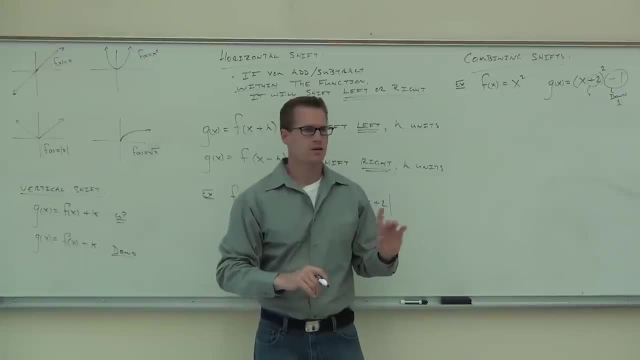 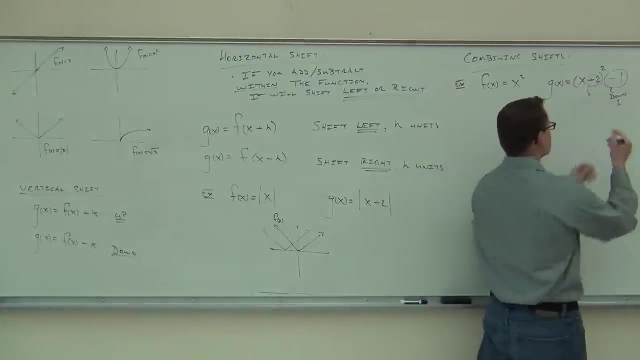 Horizontal, I know it's horizontal. Which way? Left or right, Left, Left, It's kind of backwards of what it looks like to you initially. So only this one, though. This one's the way it's supposed to be. One two: 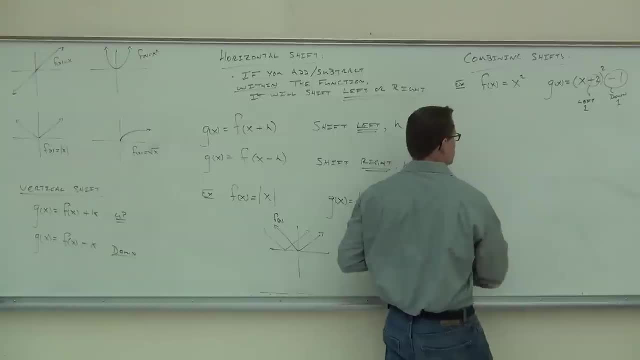 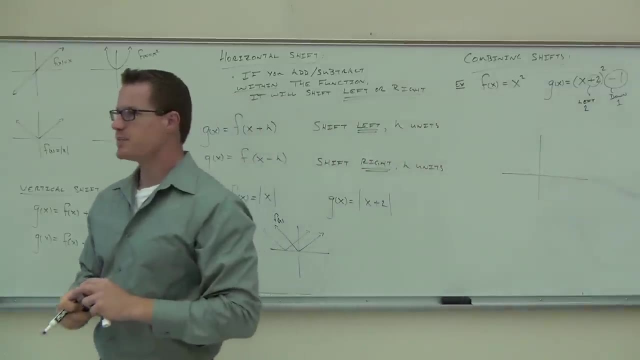 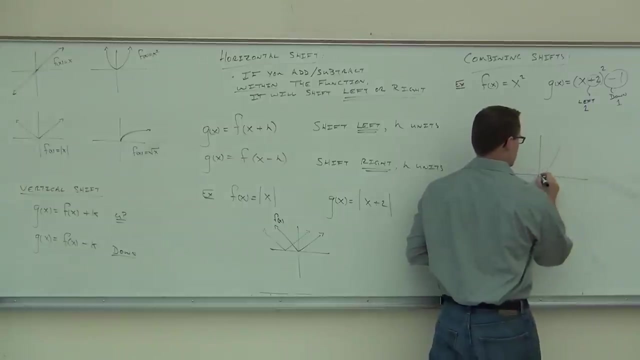 Let's see if we can do all this. The first thing you might want to do is get the picture of the basic graph shape in your head first. So, since this thing is a parabola, our basic graph starts at the origin and makes a nice parabolic or U-shape. 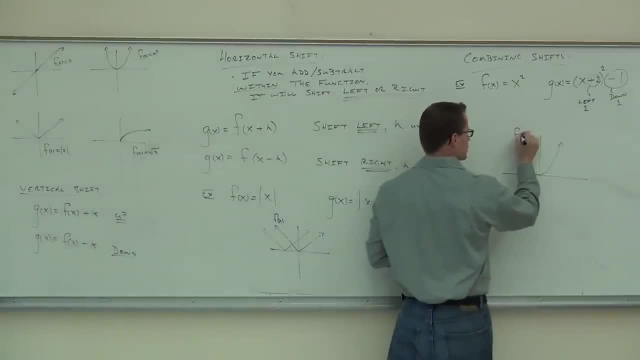 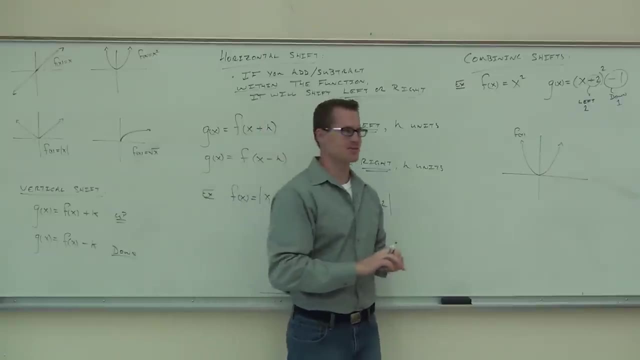 And we'll let that do it. Okay, And then we'll label it F of X. Are you getting good at drawing parabolas, yet Starting to look prettier? I hope they will. You'll draw a lot of them. Then we're going to use what we did over here to shift this graph around. 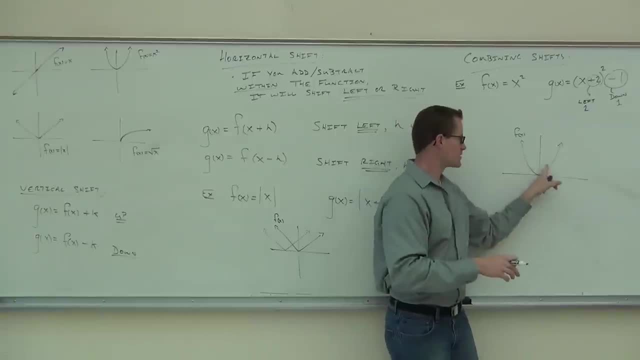 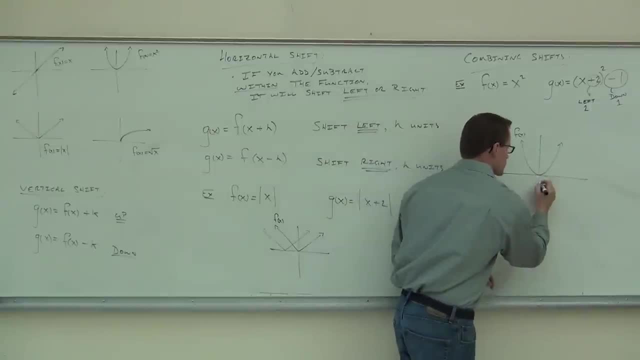 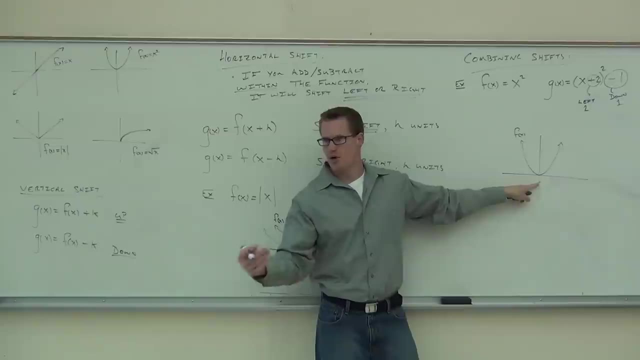 Downward, Downward. So we're going to start with that: down one. Okay, Down one means right there, Do I make a graph? right there? No, No, No, No, Because I still need to shift this over, so no, 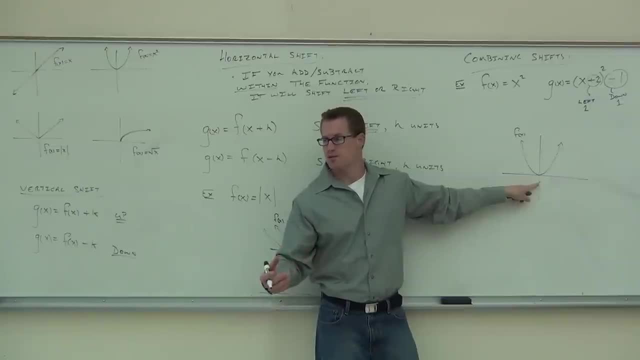 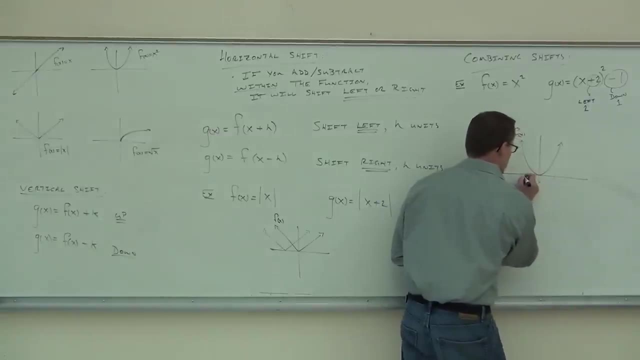 So we could do a combination of these shifts. We do the down one, but then we also have to go where Left two, Left two, Okay, So left two. That's one two. you know what? It sounds silly, but I often have people do this. 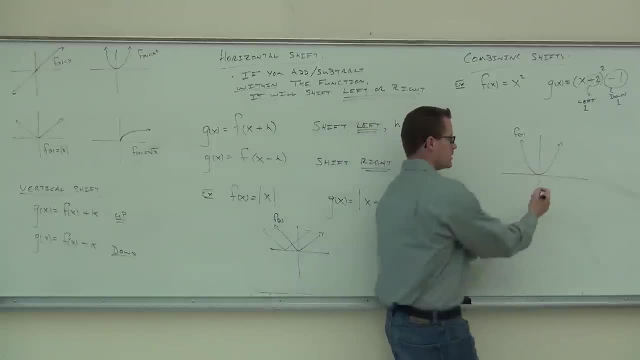 I often have people do this basic graph, basic graph, which is correct. Put a graph here and put a graph here. That's not really what we're doing here, folks. Or they'll put a dot here and a dot here and draw a line. 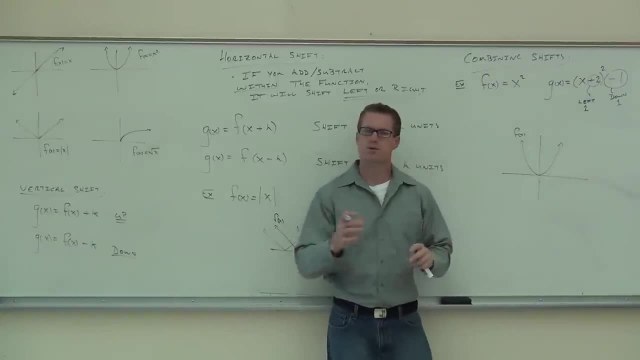 We are not drawing lines here. What we're doing is drawing parabolas. All you're doing is moving this parabola from the origin to somewhere where your directions tell you to go- In this case, down one and left two. So we do a combination of that: We move our graph. 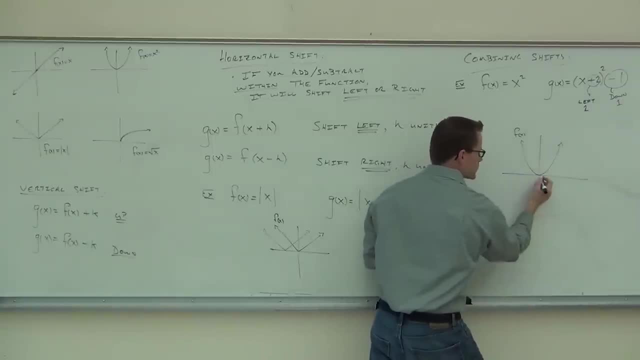 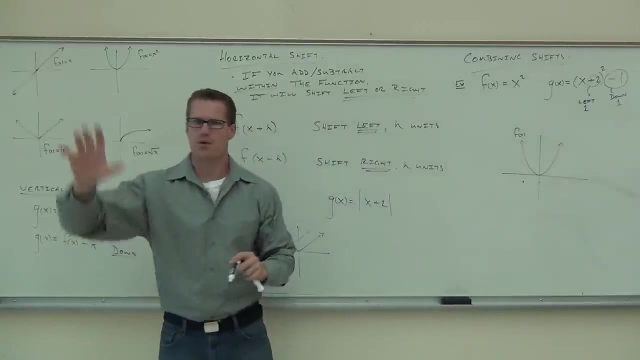 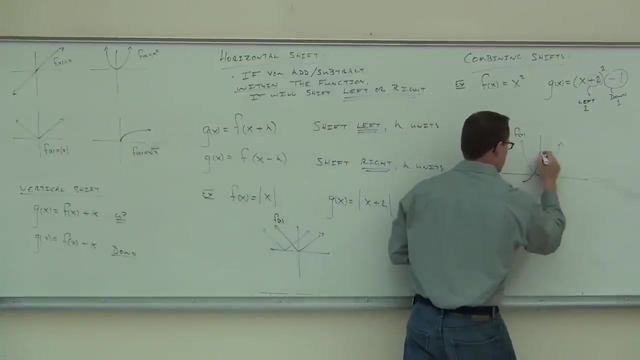 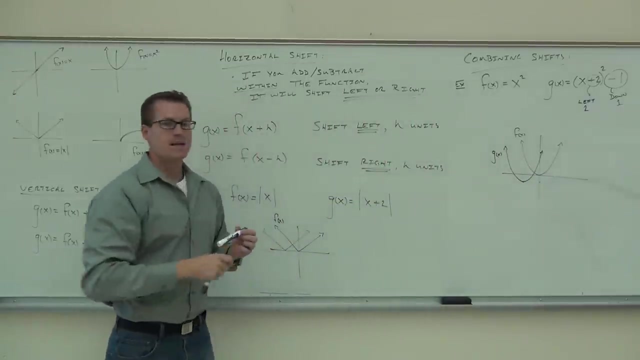 down one from here and left two. So we move our vertex down one, left two, We put a point and then we simply have to redraw our parabola from that point. How many of you feel okay with that? Good, So let's redraw that. Just make it kind of nice and pretty. G of x Now. 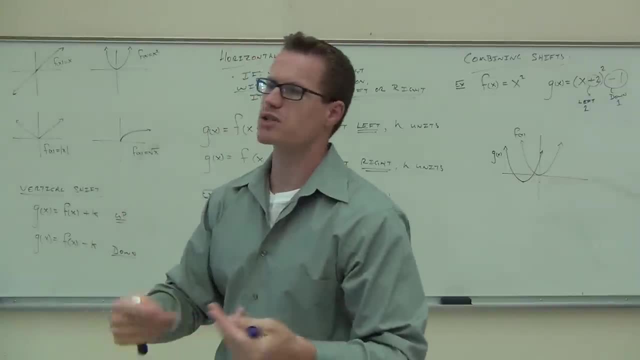 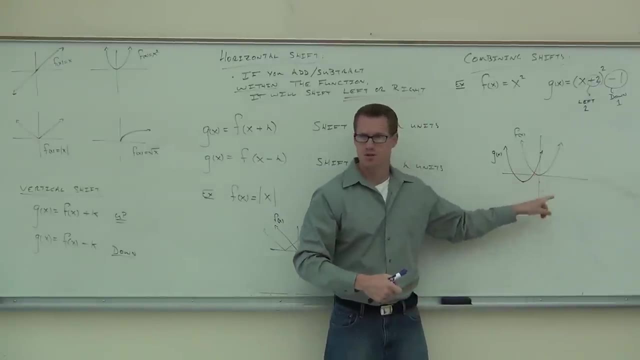 the graph shape doesn't have to be exactly precisely perfect. I mean, we are sketching here. However, the vertex does need to be precise. I need to know that. you understand. this is down one and left two, not down two and left one. 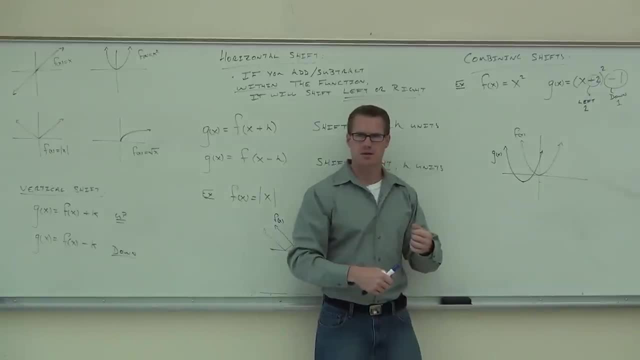 So I do need to label your graphs like that. Are you with me on this? So, while your graph shapes might be skinnier or wider than mine, that's okay for right now, But I do need that vertex to be precise. Let's try one on your own and then we'll move on. 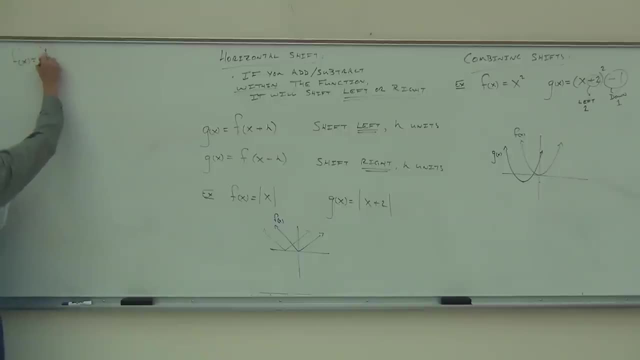 You've got one on trifecta. Give that one a try for me. So look from the right to the left. Identify those shifts. The first shift you should see from the right to the left would be a vertical shift, That's anything that's added or subtracted after the function ends the original function. 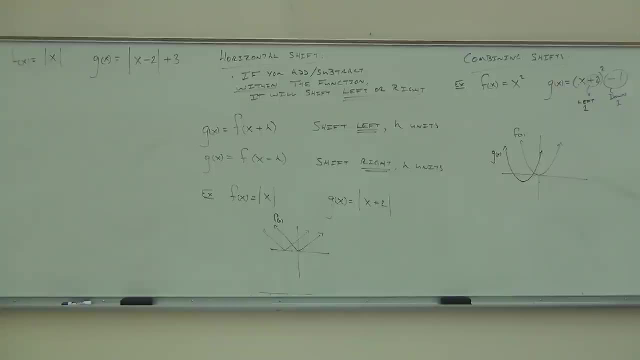 ends. So anything basically outside of parentheses or outside of absolute value or outside of the square root would be a vertical shift. Then we look at if there's anything inside the function, such as inside the parentheses or inside the absolute value or inside the square root, that would be a horizontal shift. 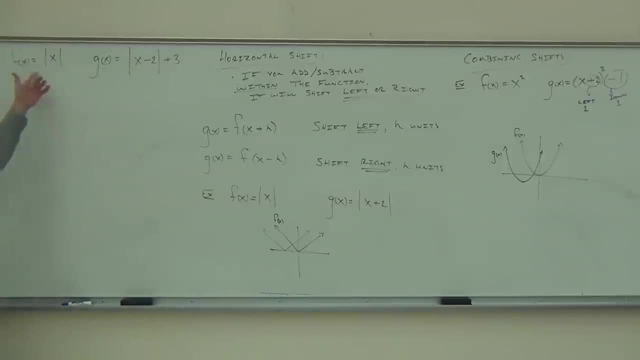 So when we look at our problem over here, our basic graph shape, what's our basic graph shape, folks? V- Yeah, it's the absolute value graph. It's like the V. Okay, So we'll draw that first, just to make sure we have that in our head. 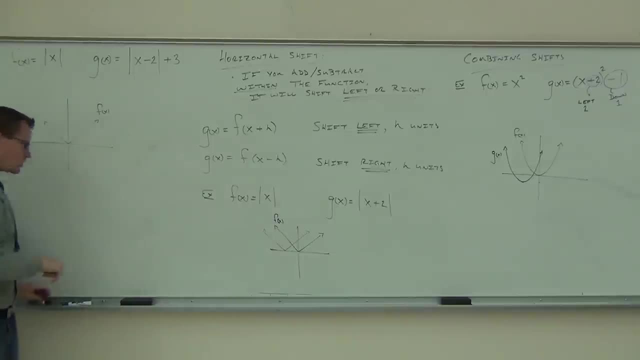 So that's f of x. Next thing we do is what I told you over here: We're going to look at each individual piece of this, circle it and tell me what it is. I am going to have you do that in your test. 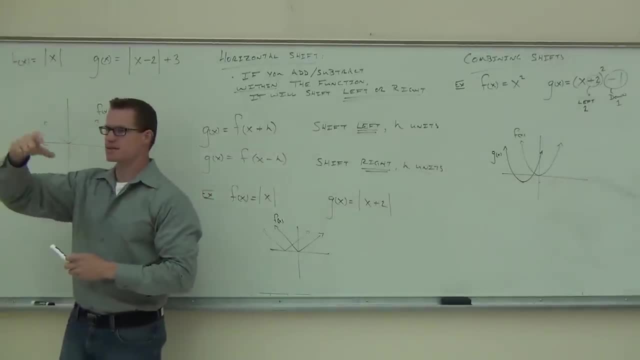 Make sure you circle those parts and say, okay, this means up or down, This means left or right. I check for that, So I'll circle this piece. That's the first one I see. What does that plus 3 mean? 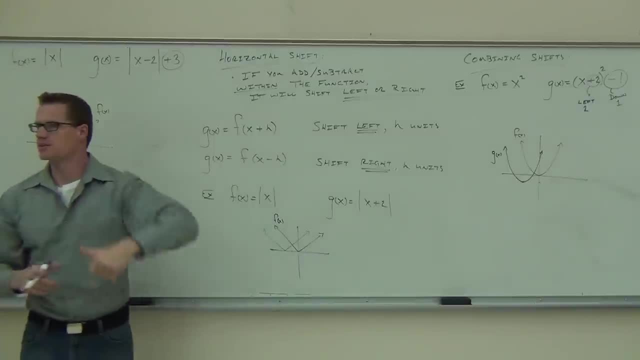 Up 30.. Great, It's after the function. It means up, Minus means down, So this is going to be up 3.. You are right. Next thing we do is look at anything inside the function. I see a minus 2 inside the function. 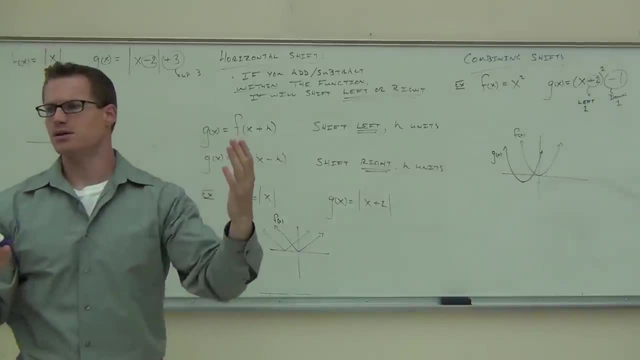 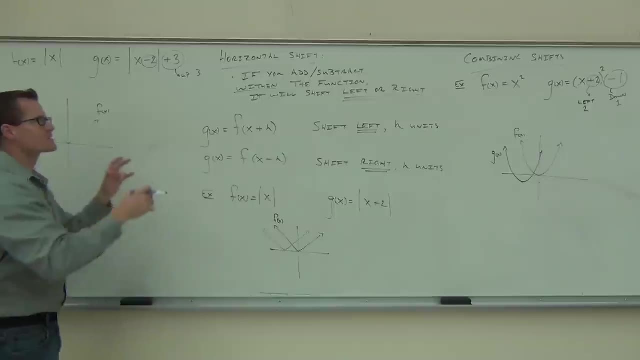 That means inside the absolute values, in this case That minus 2, what does that mean to you? Right, Right, Good, Okay, So I'm incorrect. You're all right, We're going to the right. So that minus 2 means we're actually slowing down the function. 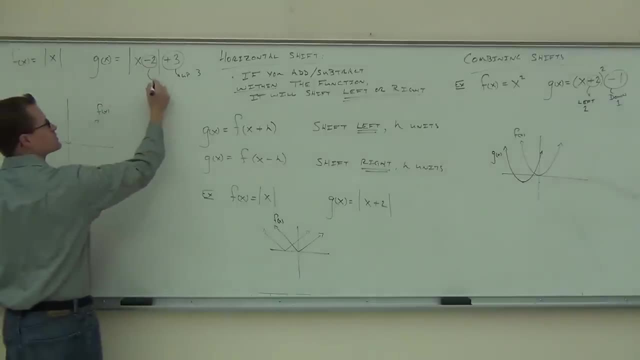 If it would normally start here, now it's starting later. So this minus 2 means to the right. Okay, So that minus 2 is going to be 1, 2. And we do a combination of those things. So from our original function we're going to move this up 3.. 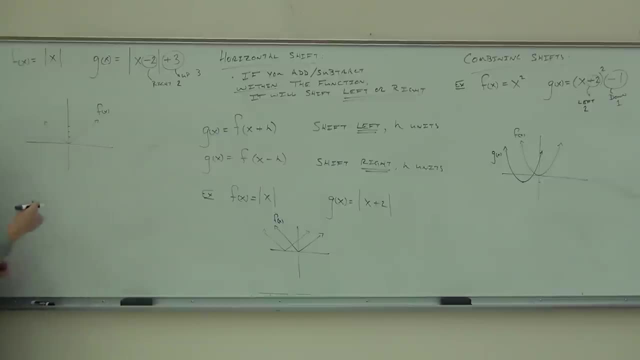 So we're going to do 1,, 2, 3.. And we're going to move it to the right 2.. So we're moving this point up: 3, 1, 2, 3.. And right: 2, 1, 2.. 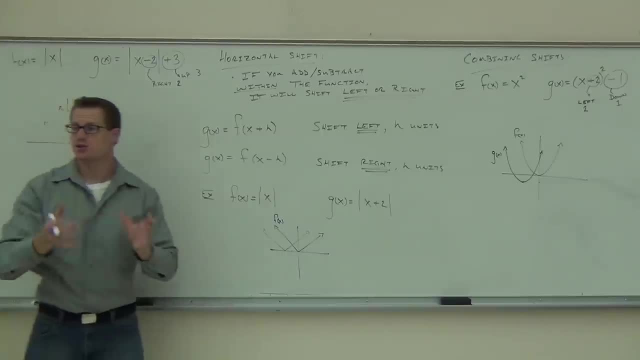 We redraw that v. The shape of the graph does not change. You should have two Bs or two parabolas or two lines, whatever you have, according to your original. So here we'll label this G of X, This one's F of X. 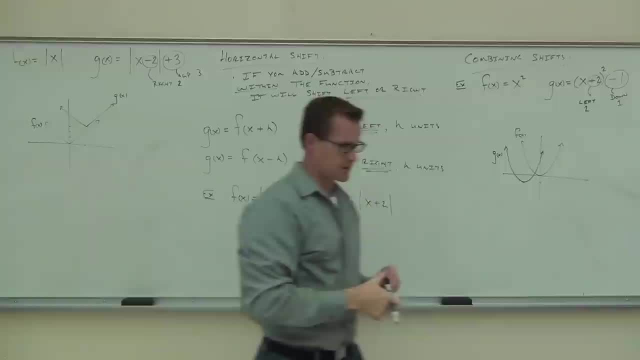 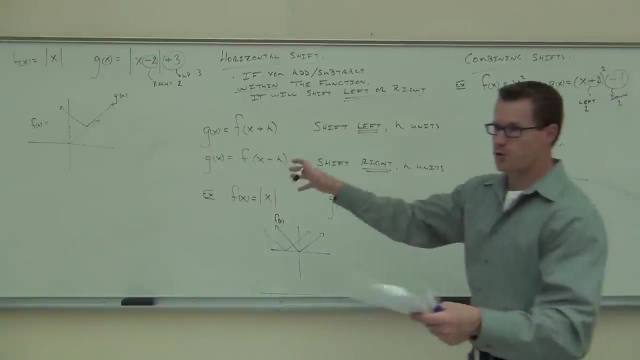 How many of you got that correct shifting? Good for you. That's fantastic. Now there's one more that we've got to talk about. In fact, we've already talked about all of these. I'm just kind of giving them the formal names and, formally, how you do it. 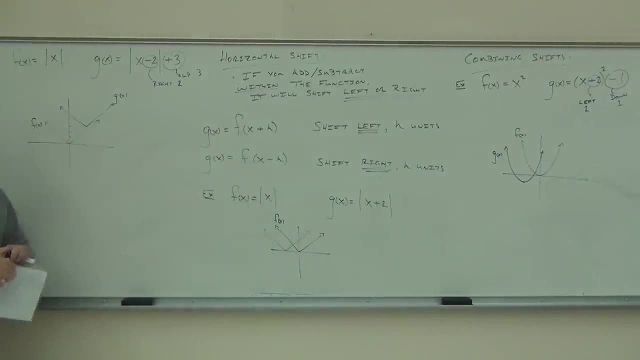 We've already done all this stuff in section 8.1 or 8.2, by graphing them, But there was one more that we haven't covered yet. We've done the vertical, We've done the horizontal. However, do you remember there was one more, when we put a negative in front of our function? 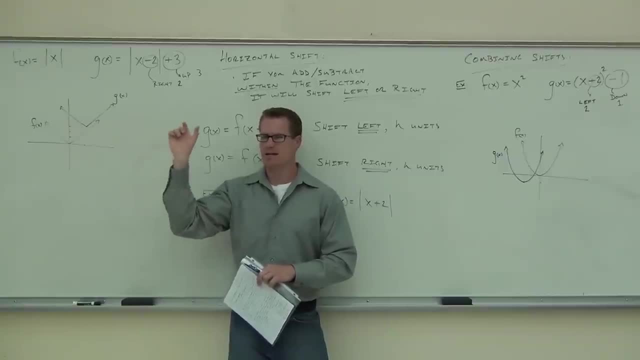 What did that do? Remember we had X squared and we had negative X squared. Remember that X squared was upward, facing What was negative X squared? Yeah, all it did was go. it just flipped it over. What that's called is a reflection. 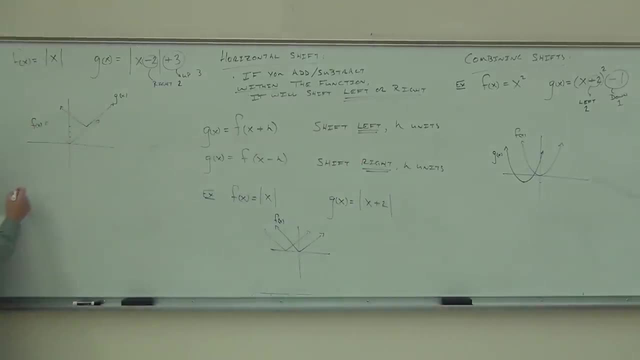 So we can also reflect our graphs. Specifically, we're reflecting across the X axis. We're treating the X axis like a mirror and flipping it over that. Here's all you need to do to reflect a function. You take your basic graph shape and what we found out from earlier. 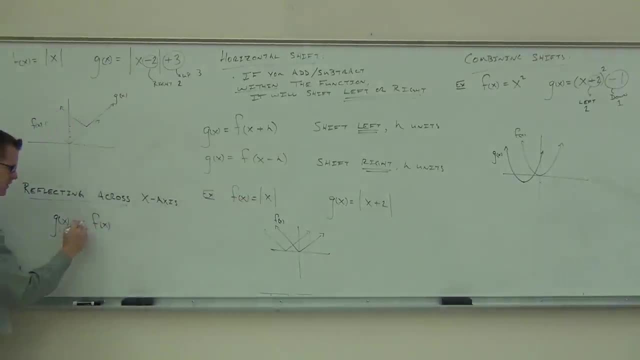 X squared and negative X squared are reflections of each other. If you put a negative in front of your function, what that's going to do is reflect it across the X axis. That's all it does. It just takes your original shape and flips it upside down. 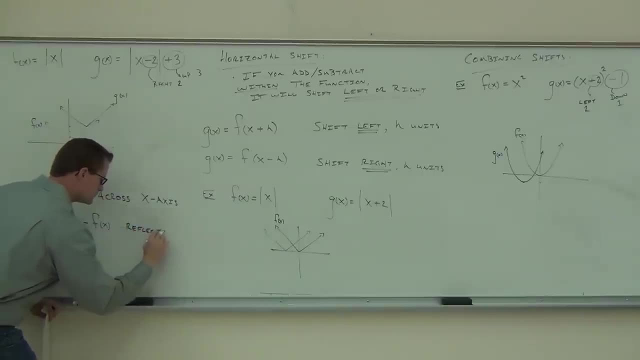 So if you put a negative in front of your function, that's a reflection across the X axis, And that's a reflection across the X axis. Now, the exact same thing. if we had a positive, we'd be reflecting our graph shape over and over again. 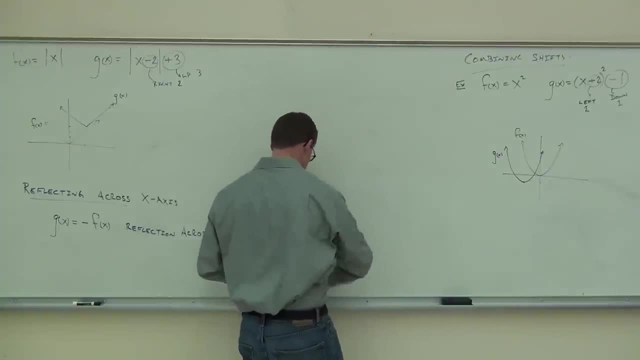 But the negative times a we'd be reflecting across the X axis And you'd be reflecting your graph shape over and over again. Let's have a look at the graph shape and let's see what we find. This is okay, we're going to say if we want to see a reflection across this axis. 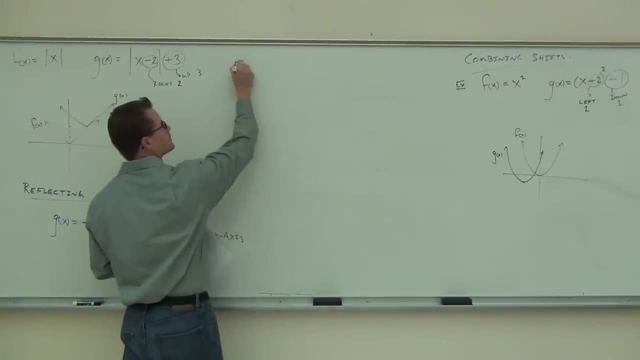 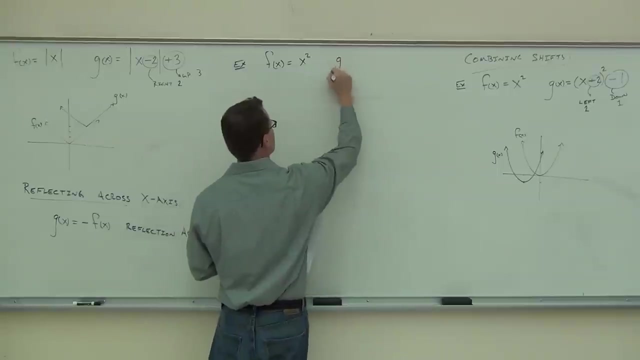 The first time we see the reflection, we're going to be reflecting the x-axis, So we're going to be reflecting the x-axis. If you don't remember, I'm going to draw this one again. Here's what this says: If f of x is our basic graph shape, which you all know, that's a parabola at this point. 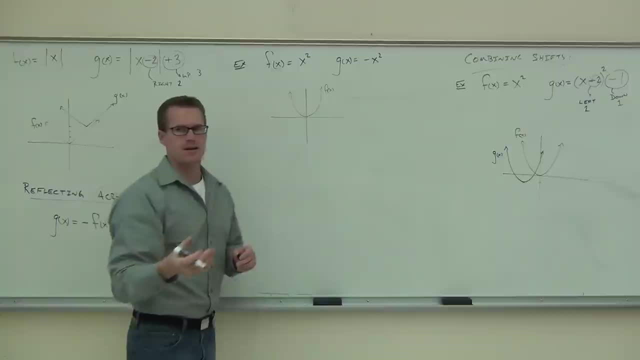 negative. f of x takes every value and makes it negative, So does the zero change. Am I shifting this anywhere? No, there's no plus, there's no minus. there's nothing at the very end. There's nothing within the parentheses. 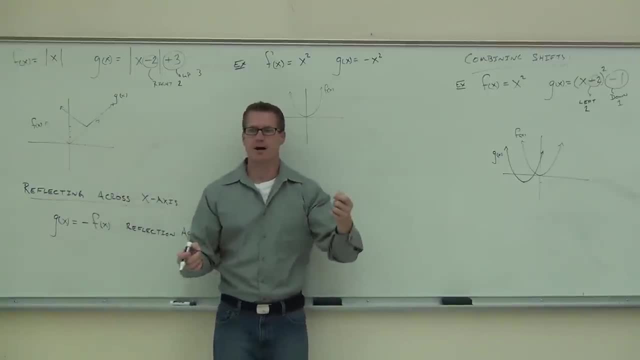 So the vertex isn't moving anywhere. All it's saying is that every other value is going to become negative. So where we had positive 1, here we have negative 1.. Where Positive 4, we're going to have negative 4.. 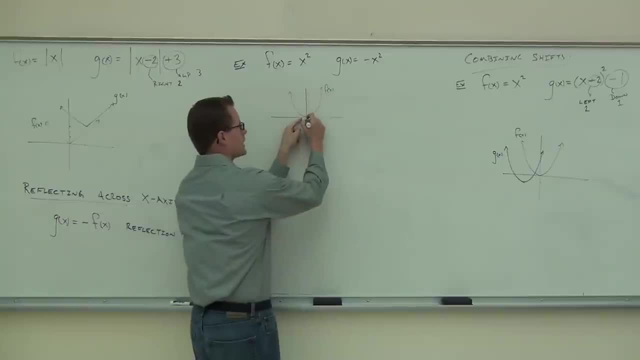 We have positive 9,, we're going to have negative 9.. So it takes this whole side and it flips upside down, And this side where we had positive 1, again negative 1, and so forth. So this is going to take our graph and just reflect it. 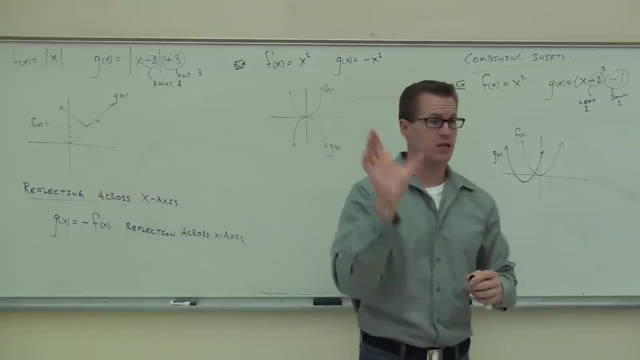 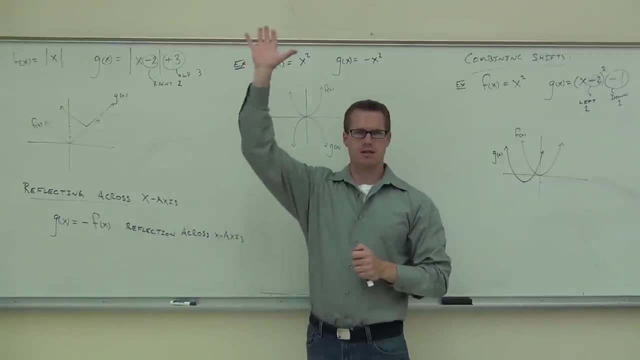 That's why that negative does that And that will work with any of your basic graph shapes. It will take whatever function you originally had. it will flip it upside down. That's basically what we're doing. How many of you feel okay with the vertical, horizontal and the reflecting? 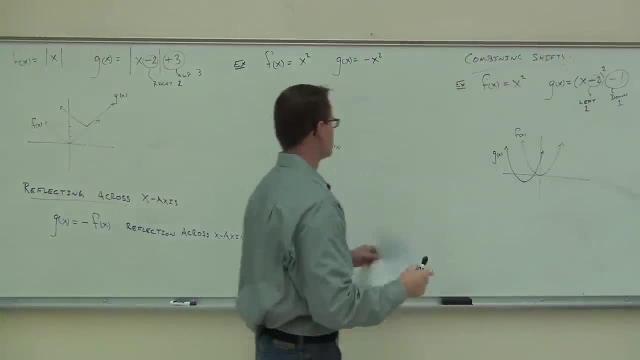 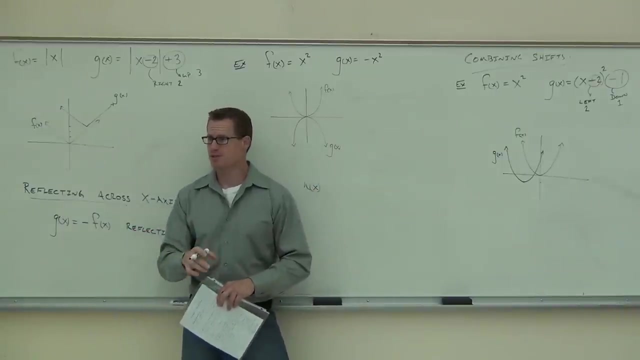 Sweet. Let's put all of them together. Let's put all of these together and see what we can get out of these. So I want you to graph this one now. I've got to tell you, if you start your homework and you're making tables up for this thing, it's going to take you forever. 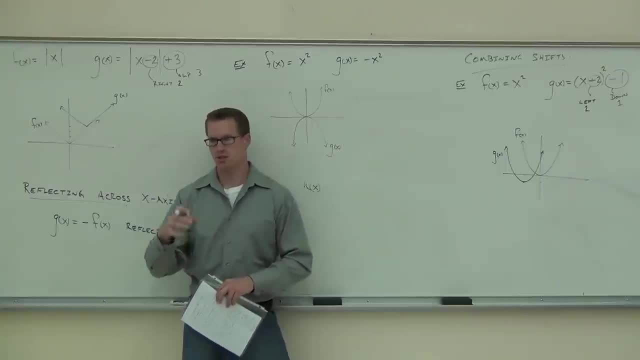 You're going to. I don't want to say you're going to make mistakes, but if you don't make mistakes it's going to take you forever anyway And typically when people use tables on this type of graphing, they make mistakes with the signs. 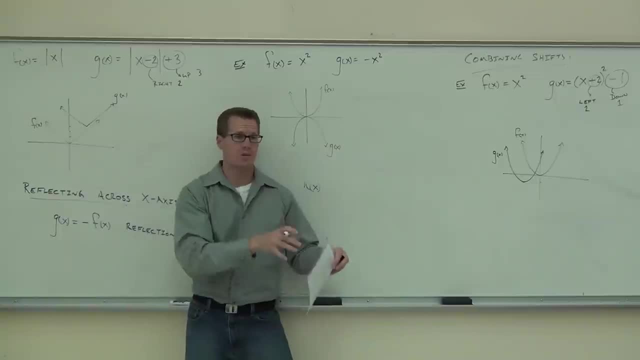 That's usually what happens. So really, I want you to get away from making tables on every graph. you see, What I'd like you to do is use the shifting that we're talking about in class. I swear on the test. this could be like the easiest problem on the test. 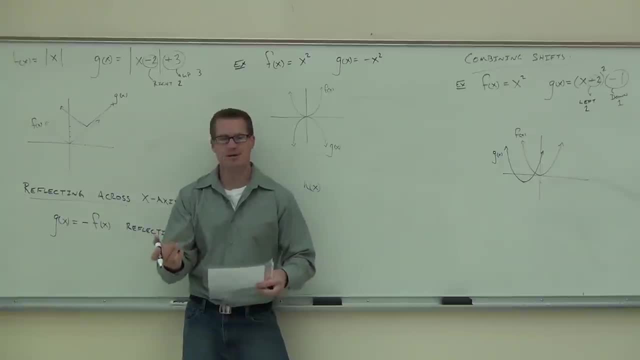 It seriously takes five seconds if you know what you're doing. If you have to make a table, then it's not going to come out right And you're going to take a long time to do that. So really practice the shifting on this homework that I'm going to give you tonight. 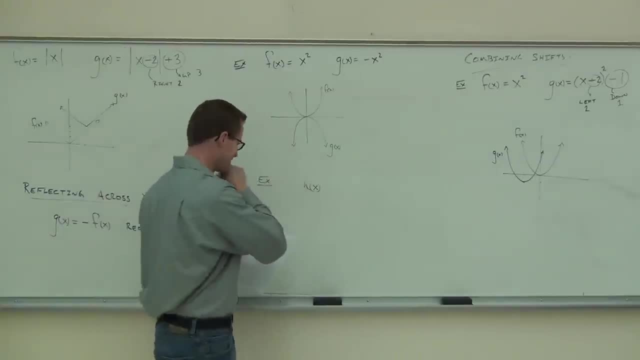 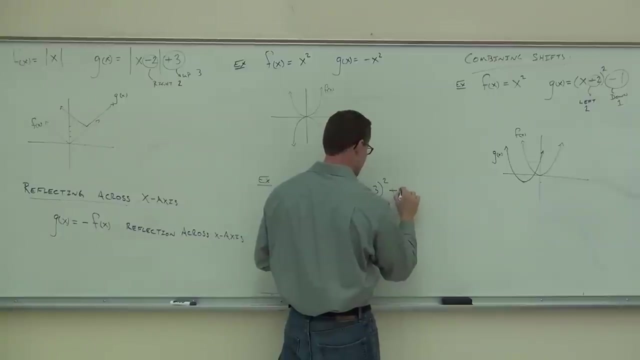 By the way, you're going to have homework tonight. Had a couple days off, right One, That's a couple, That's a couple. Okay, you're going to notice I didn't give you the basic graph shape explicitly, but you should still be able to figure it out from just looking at this thing. 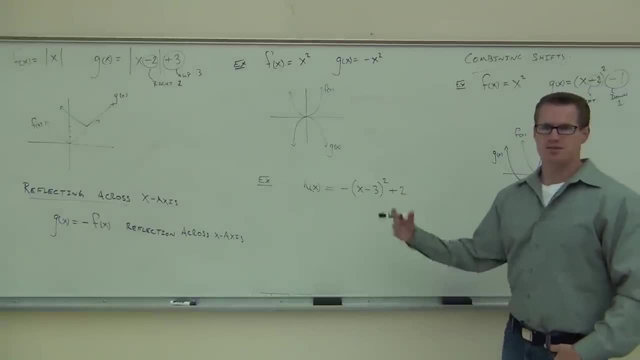 So from just looking at this thing, would you say: this is a straight line. Is this the V, Is this the parabola, Or is this the funny half parabola on the side thing, Parabola. Why is it a parabola? 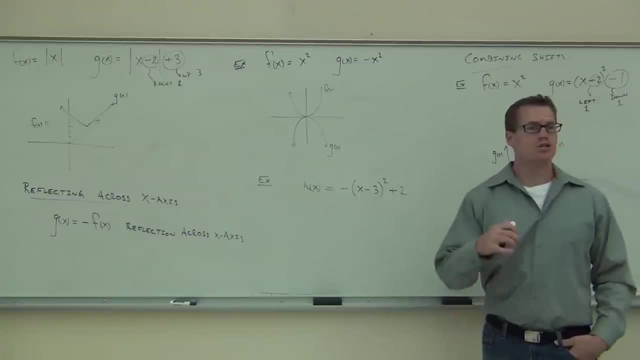 Because that's a square, Definitely, That's for sure, a parabola. Now we're still going to go about and do the same thing we did on these examples, which is we're going to go from the right to the left. 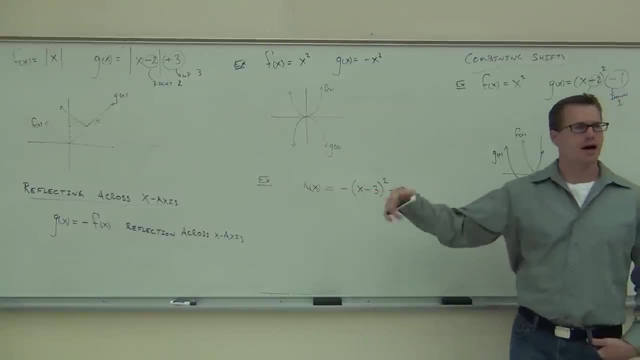 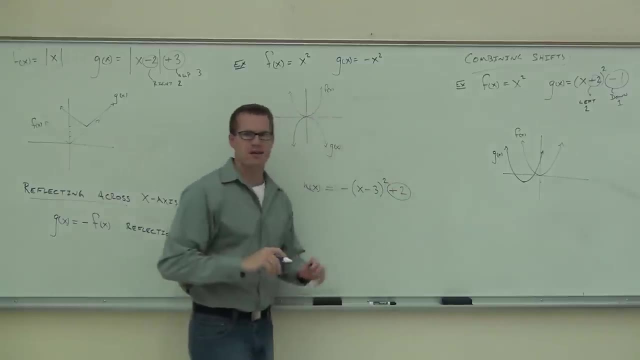 I may have misspoke earlier and said left to right. We're going from the right to the left identifying these things, So we're going to go right to left. The first thing I see is a plus 2.. Now, we should know that. that plus 2, that's at the end of our function. 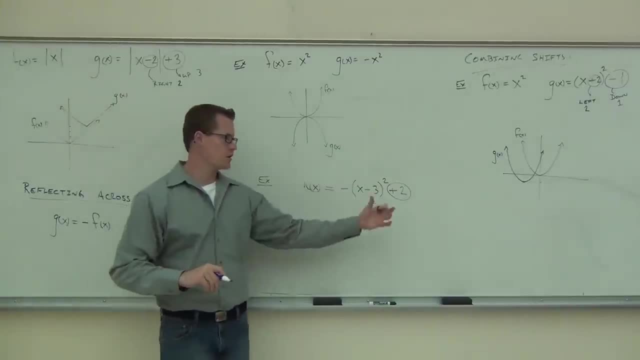 That's after everything's happened already. That's adding 2 to whatever number you get out of this. What's that going to do to our graph? It's going to change, That's right. This is a vertical shift Up 2.. 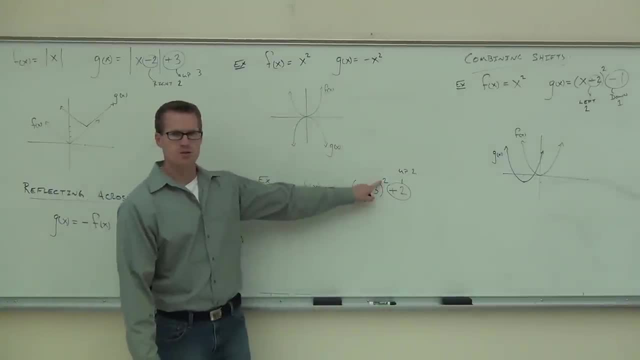 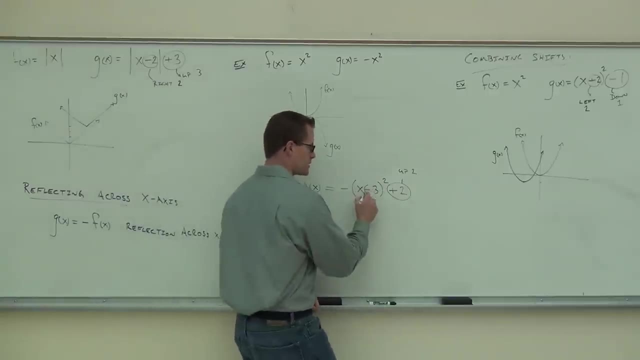 No problem, This thing told us it was a parabola, So that 2 really doesn't do a whole lot for us. It just said: oh, you're dealing with a parabola there, But inside of our function this thing does something. 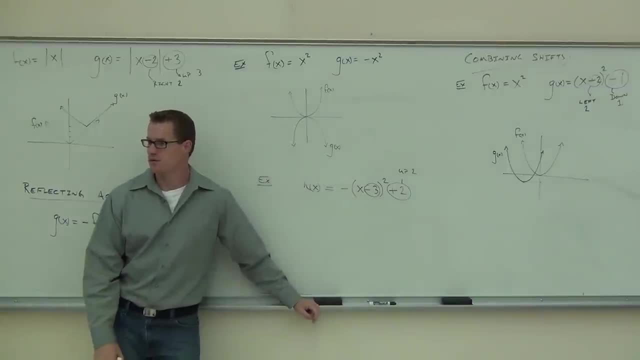 That minus 3 should shift it somehow. How does it shift it Right? Good, So so far we have up 2.. It was at the end. We moved a little bit to the left. We have right 3.. 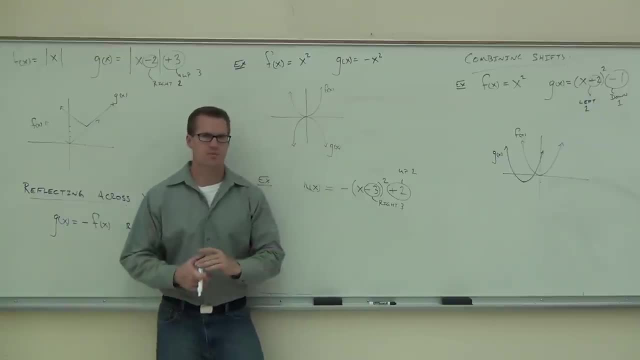 We're going to move to the right. And lastly, there's one more piece of this puzzle we have. What is it? Yeah, this negative here, That negative when you see that that's going to be a reflection Or you're going to flip it over. 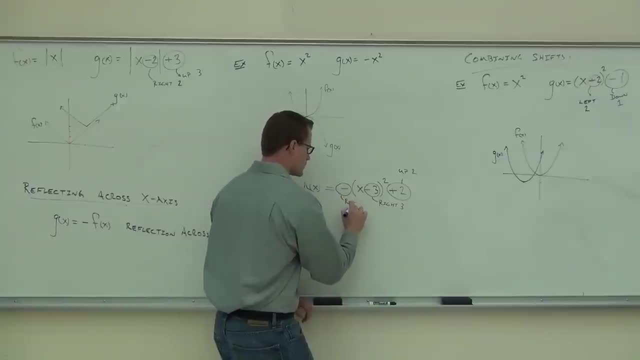 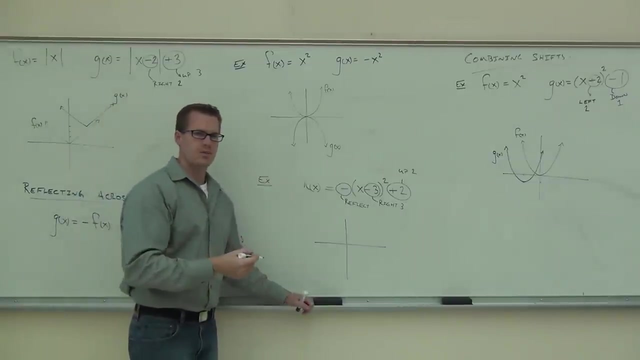 So we'll put reflect. So let's see how this turns out. Our original shape. you can choose to put this or not, I really don't care. If you do put it, you have to label your functions, OK. If you don't put it, well, then it's going to be implied. 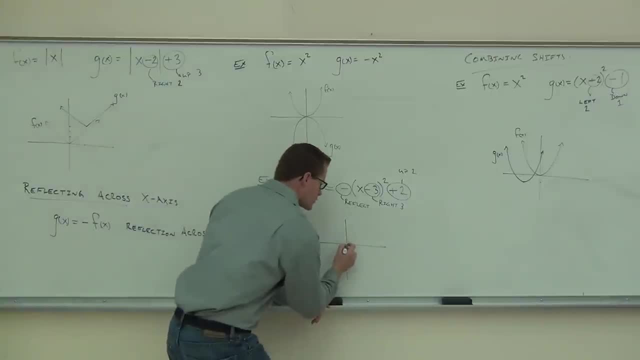 that the function you draw is h of x. So if I draw my original, like we've been practicing, if I draw that you have to label this like f of x, OK, And you have to label the next one h of x, because I need to be able. 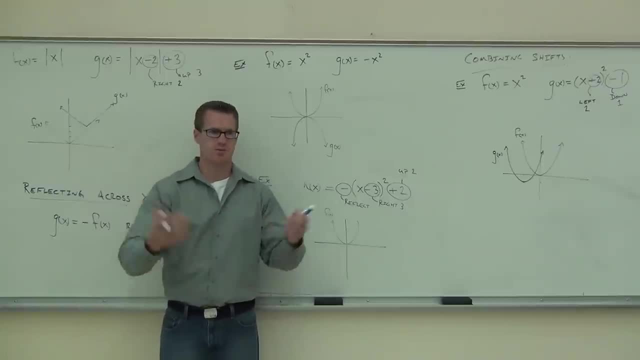 to tell the difference between them. You're with me on that, right. I can't have you just draw two random graphs and go pick one. That's not going to work. So this is f of x. Now we're going to make h of x by doing: 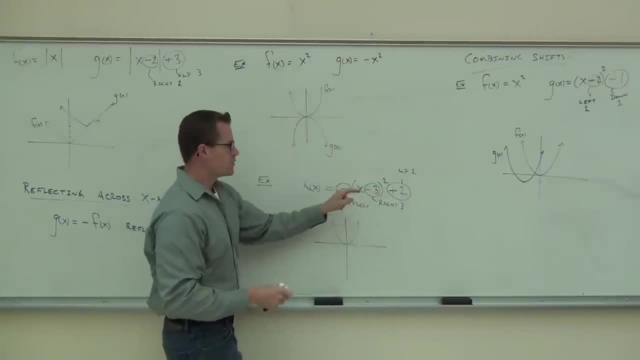 by the way, this is optional. You don't have to do this. You can go directly to this one if you'd like. We're going to shift this around and make our h of x. It says we're going to go up two. 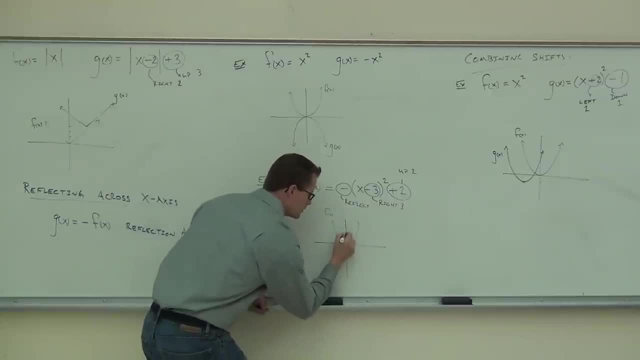 So on our graph we're going to make two steps up. It said we're going to go to the right three. That's one, two, three to the right. We do a combination of those moves. So we're going to go up two and right three. 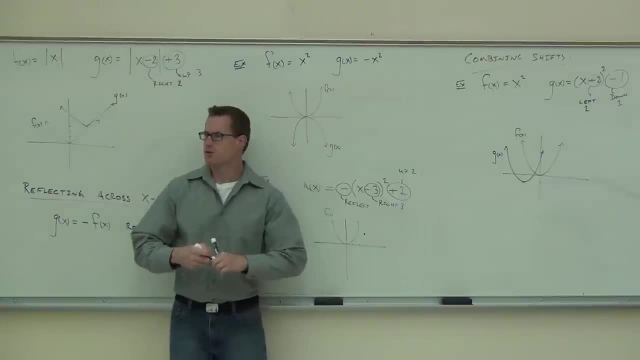 and we're going to put a point right there. That's the first thing you look at. You look at up or down first, then you look at left or right, then you put your point and then you determine whether you're going to be upward facing like your original. 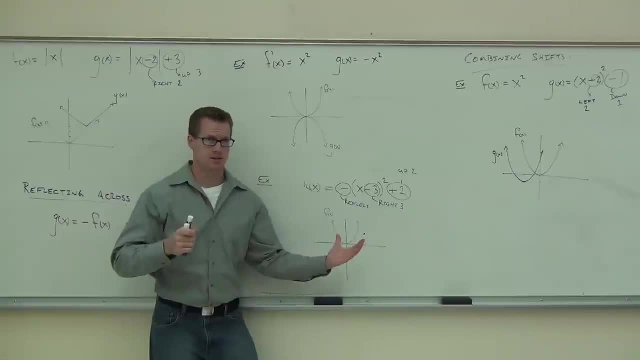 or downward facing. if it's a reflection, Which one are we going to be? in this case, That one, Yeah, Yeah, We're not going to be like this. That would be you'd draw the same parabola if you did not have the negative there. 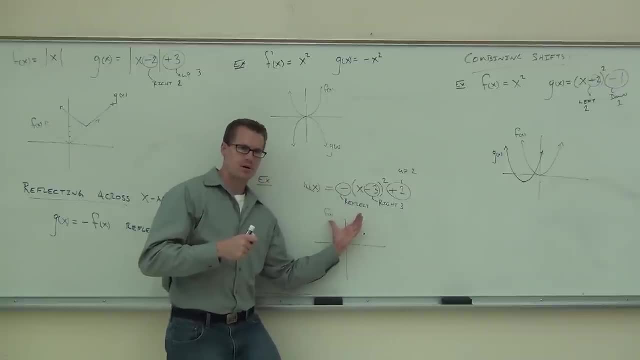 But that negative says you're original. You're not only going to shift it up, not only are you going to shift it right, but you're also going to reflect it. So we shift up, We shift right, and then we draw this thing upside down. 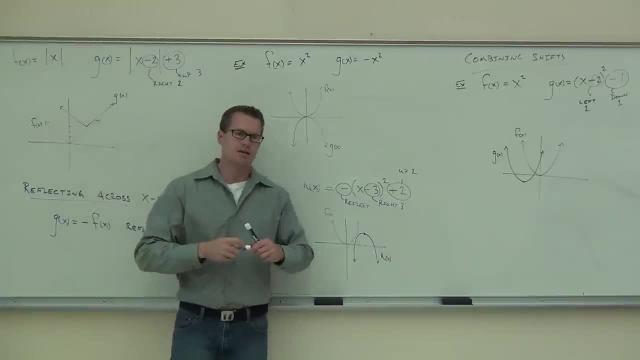 And since I have two graphs, I have to label that h of x. It's probably a good idea to label it anyway, but you ask and you must. if you have two graphs on that thing, Would you raise your hand if you feel okay with this? 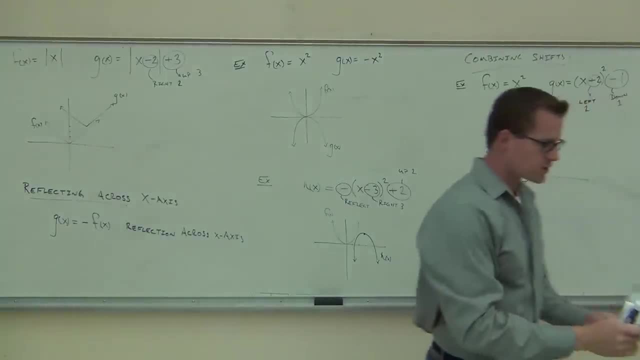 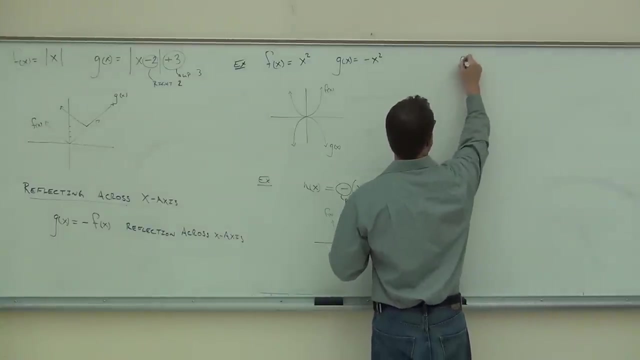 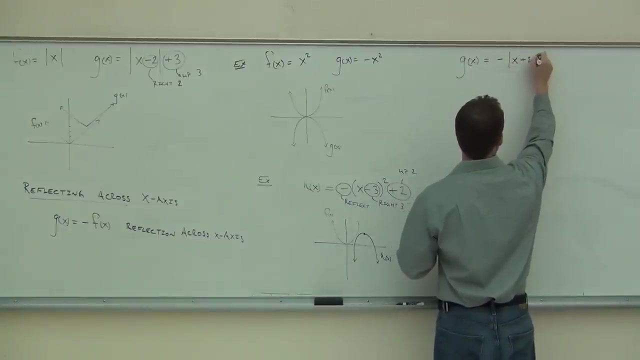 Good for you. I'm going to give you two to try on your own. Let's work through these and then we'll be done with our section. All right, All right. So I want to point out that when I do the square roots, 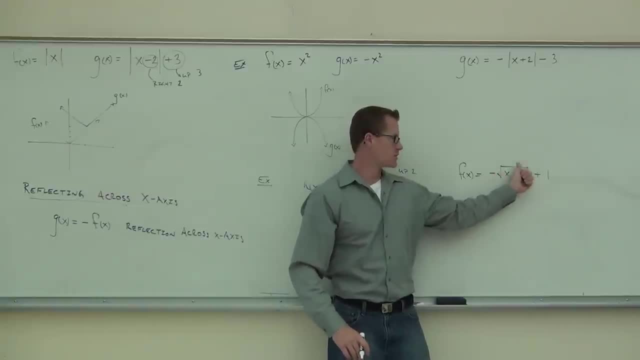 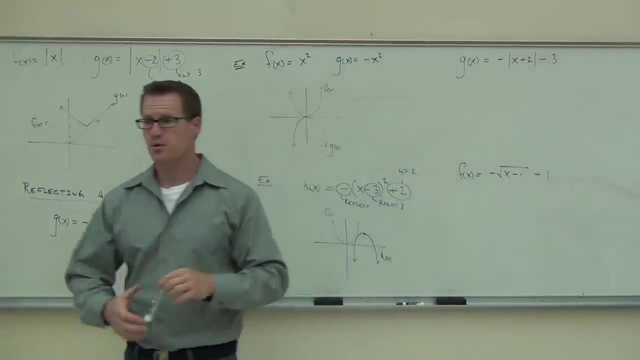 I'll put a little tail at the end of that thing. That way, if you have to rewrite it, you know exactly where that stops. So that's not going over this plus 1, that's just this minus 1 right here. So go ahead and graph those. 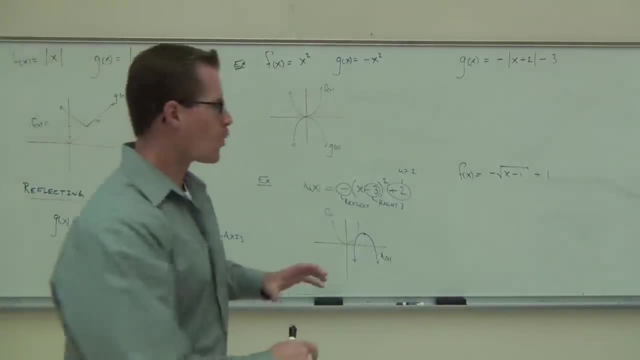 You can choose to draw your basic graph shape first, if you'd like, and then shift that around or go directly to the shift, But I do want you to circle those items and tell me what they're doing. So practice, So, practice that. 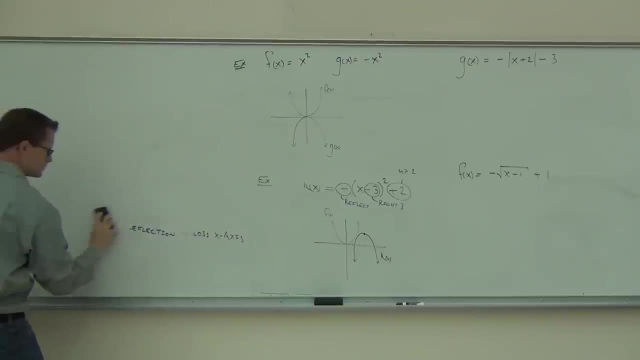 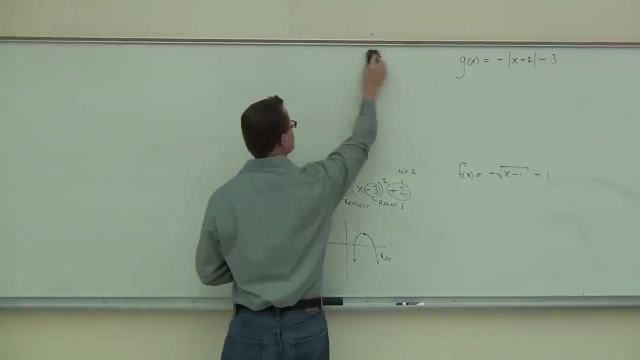 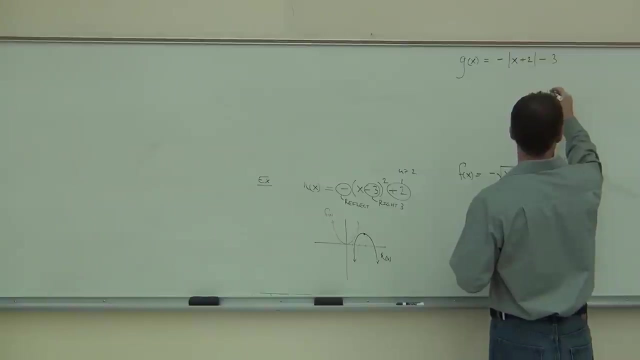 Okay, Have you noticed that when you really get the hang of these problems, you can go very, very fast? You can just kind of look at the angle. Oh yeah, I know exactly what that's doing, if you really get the ideas. 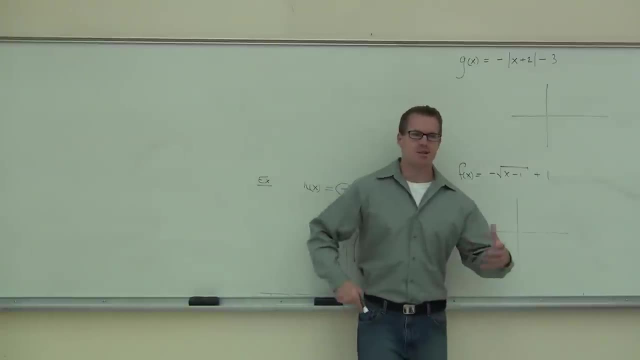 Let's talk about g of x. all right, Firstly, you've got to be- it's really imperative that you understand the basic graph shape of these things. What is the basic graph shape here? Yeah, that's the v. You've got to be able to identify between the parabola. 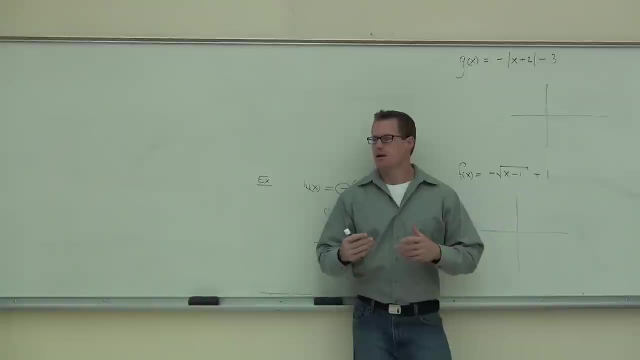 and the v and the half of the parabola on the side and the straight line. You've got to be able to do that. So in our case, for sure we get the v because we have the absolute value. So this is going to be an absolute value graph. 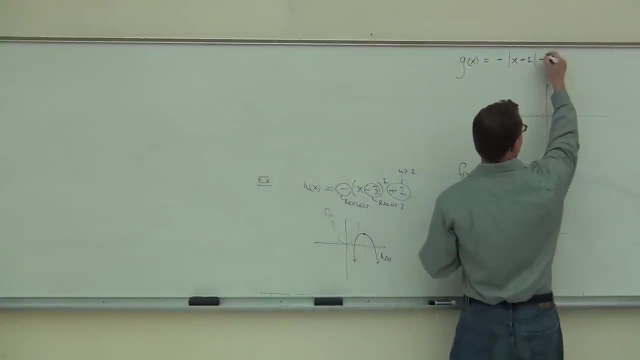 We're going to go identify these things, So off to the right, we're going to start over here. What's that minus 3? tell us Down 3.. Good, And this in here. that's within the function. so that's going to be what. 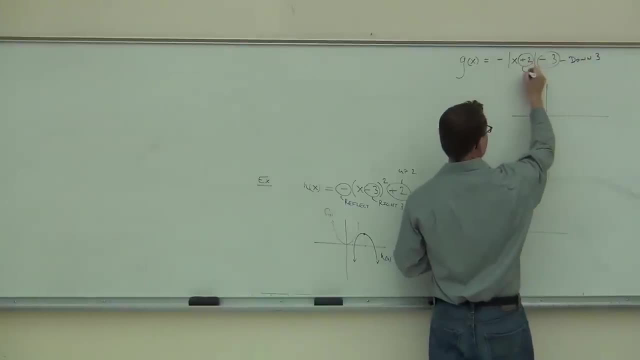 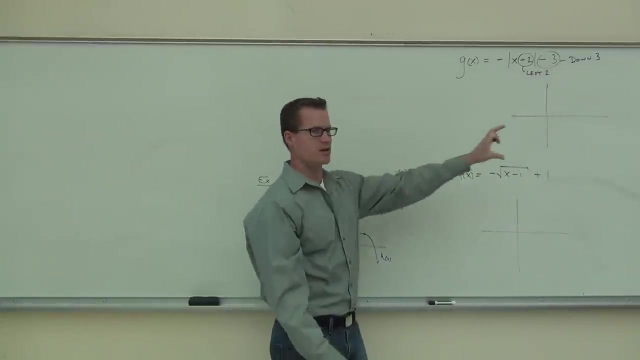 Left 2.. That's right, I mean correct, Left 2.. Okay, so we have down 3, we have left 2, we have a general idea about where this graph is going. And then, lastly, this minus means something. 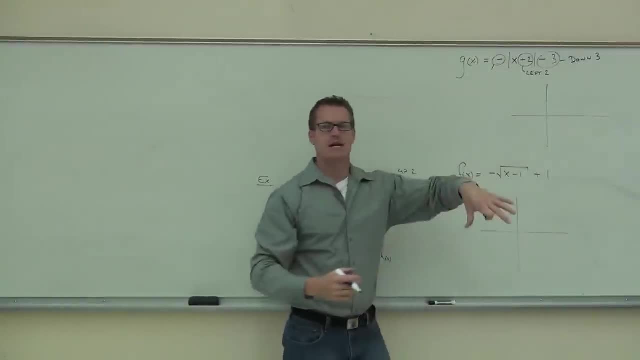 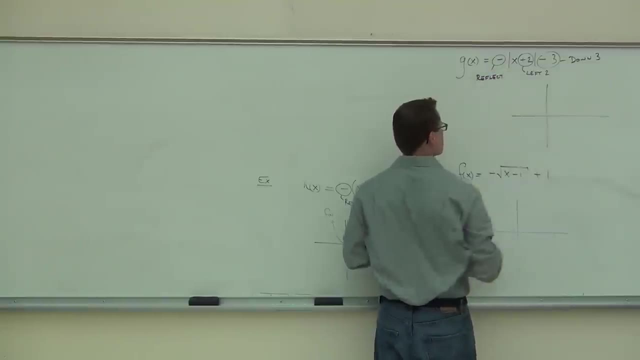 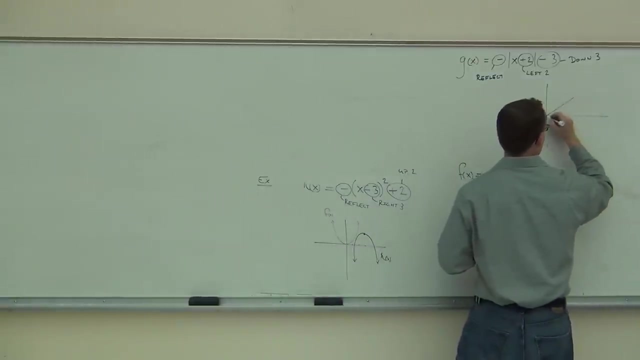 What's that tell you to do? That's that reflect? that's right. So it's going to be upside down v. If you chose to draw your original graph, that's fine. So the basic graph shape here would be a v, starting at the origin. 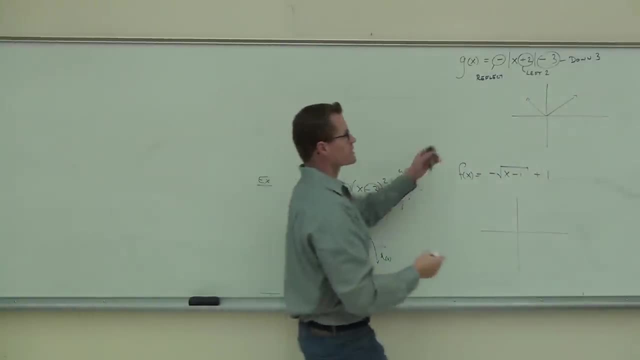 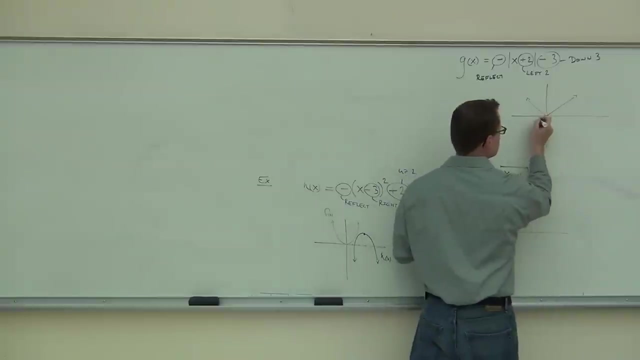 That would be the basic graph there. Now, in order to shift this thing around, it said: we're going to move it down 3.. Okay, we can do that. We're going to move it to the left. 2, and that's where we put our point right there. 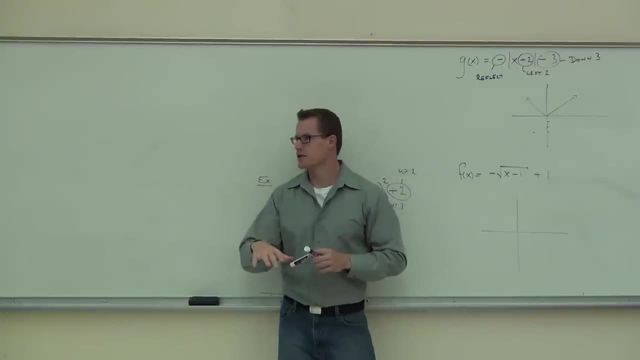 Lastly, we determine whether we're upward facing or downward facing. That's the idea In this case, since we said: reflect, we're not going to be upward facing anymore. It flipped it over, So we should be not a v, but kind of like a mountain top. 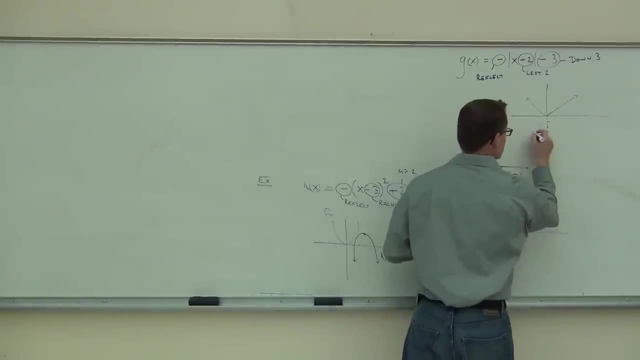 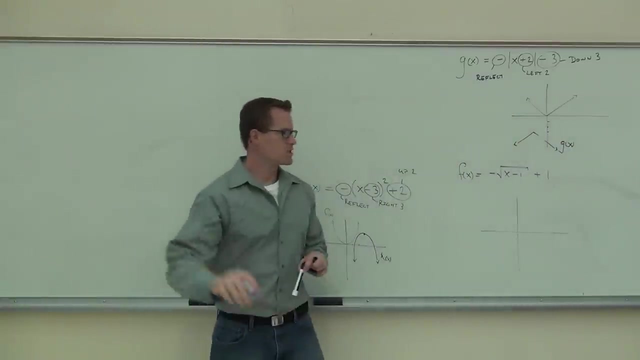 That's really what we should be looking like here, So we'll draw our v. Make sure we label this g of x. Okay, What's your agent? Have you got that Good for you? That's fantastic. What's the graph shape of this one? 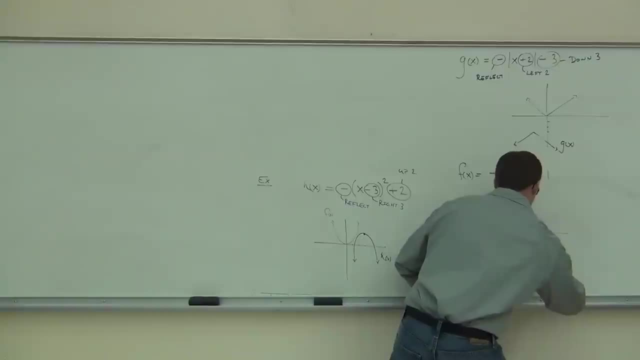 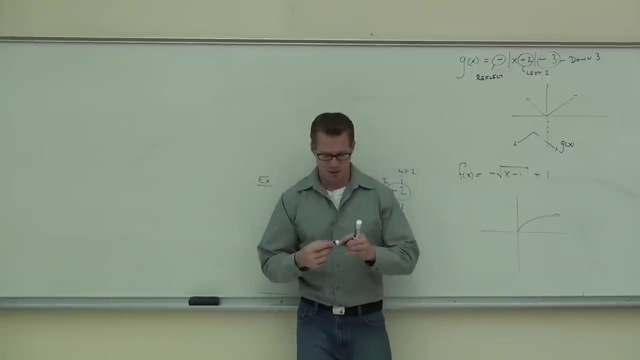 I don't have a graph. We're in line. Good Yeah, that's the half parabola. Make sure that when you're drawing these. I saw some of this on your last graphing homework. Some people are continuing this downward. 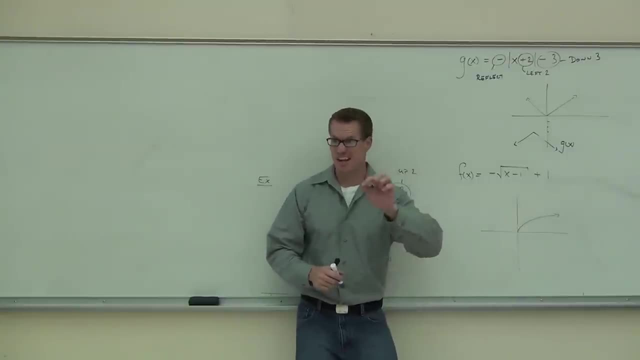 It doesn't continue, Okay, it stops. This graph actually is there. You can't even plug in these numbers. This is square root, right. So if you plug in negatives, you've got this thing wrong. You cannot have that. 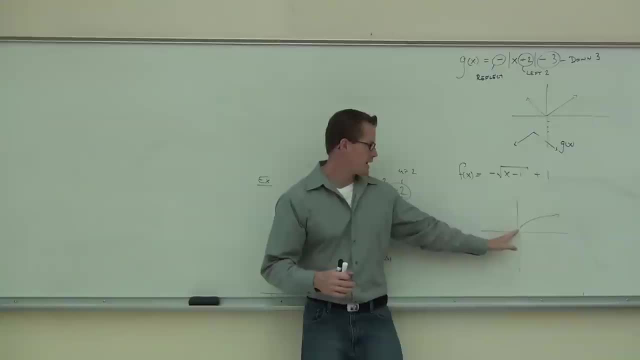 Unless you shift it around, unless you shift it around, you can't have anything on this side of the graph. Are you with me on this Shifting it to all? bets are off the table because I can plug in different things depending on where my shifting is. 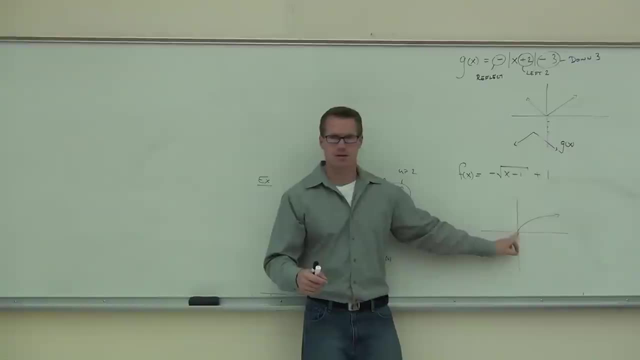 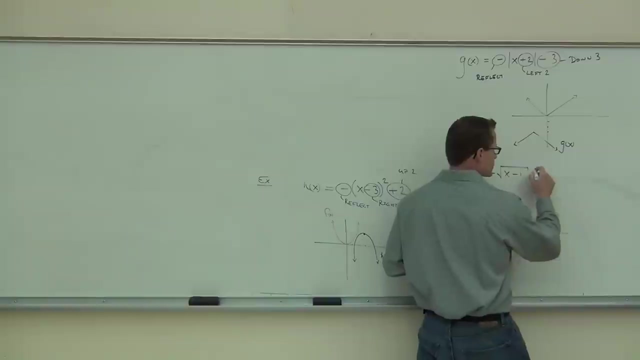 But if you're just drawing the square root of x, it has to stop right here. It has an ending point or a starting point, if you want to consider it that. So we'll identify what these things are doing. This is a plus 1.. 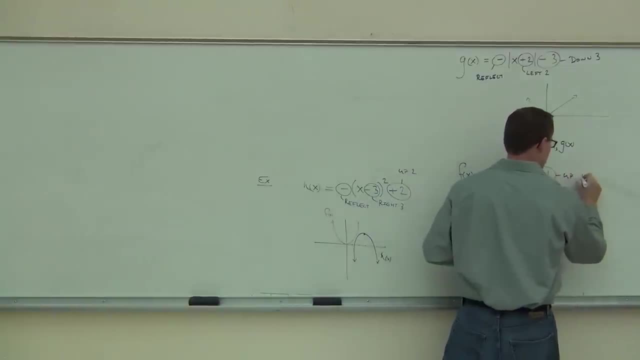 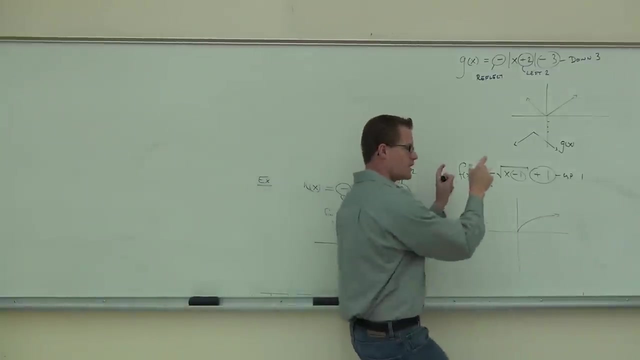 That means we're going to go up 1.. Minus 1, that happens to be within the square root, That counts as within the function. So if it's within that square root, we know we're going to be moving to the, in this case, right 1.. 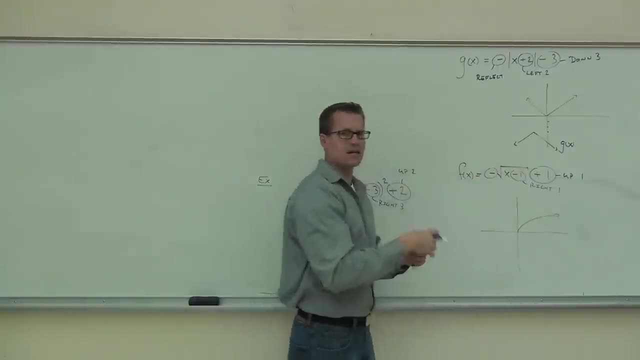 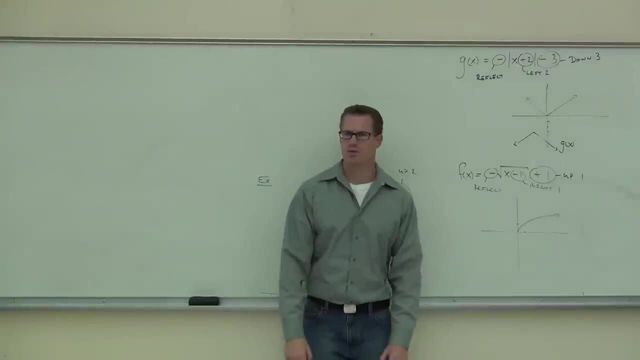 We're going to go up 1.. We're going to go up 1. And wait a second. We're also supposed to reflect it, So am I going to get the same graph like this: What am I going to get? The other half of the parabola. 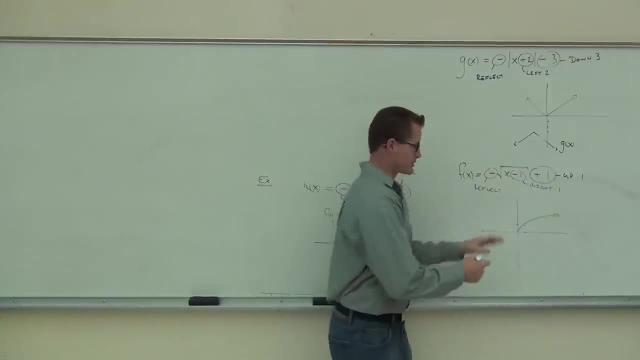 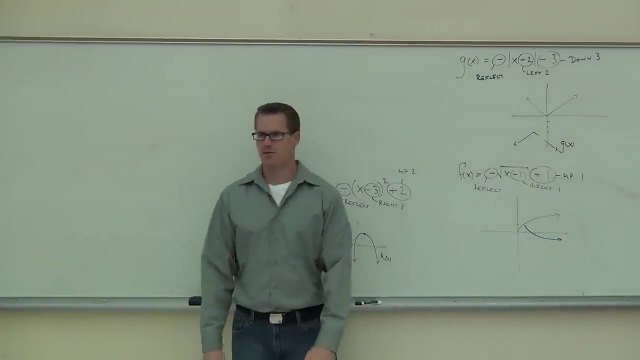 Yeah, it's like the other half. That's right. It's like this half. It's shifted a little bit, so it's not going to match up exactly, But you should do something about like that on your graph Instead of being curvy this way. it's curvy this way. 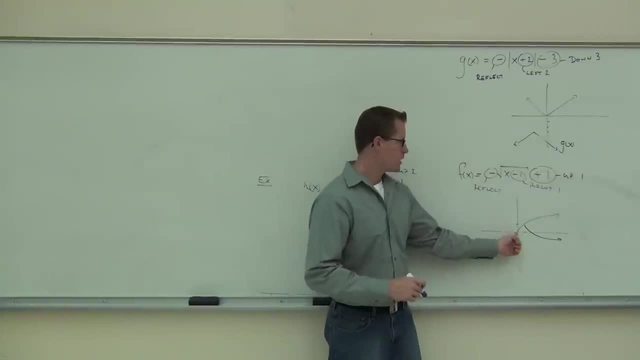 It's the other half of that parabola. So we move this up: 1.. We move it right: 1. And then we reflect it. Make sure you label that appropriately. That's our f of x in this particular case, And we're done. 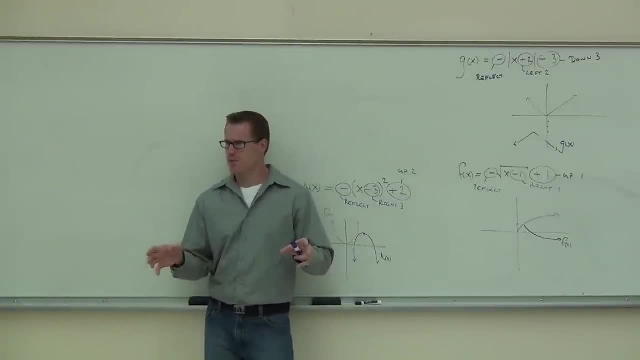 Guys, do you feel okay about this graphing stuff? Yeah, Are you able to identify the basic graph shapes without me giving it to you? Yes, you are Okay. Are you able to identify an upward shift and a downward shift? How about left and right? 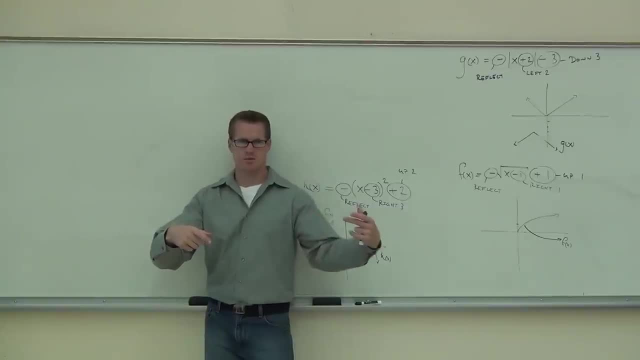 Which one's right again, The minus or the plus Minus. Minus means right, Plus means left. Okay, And what tells you how to reflect Or what to do? The day and the moment. The day and the moment. The day and the moment Real. That's very good. 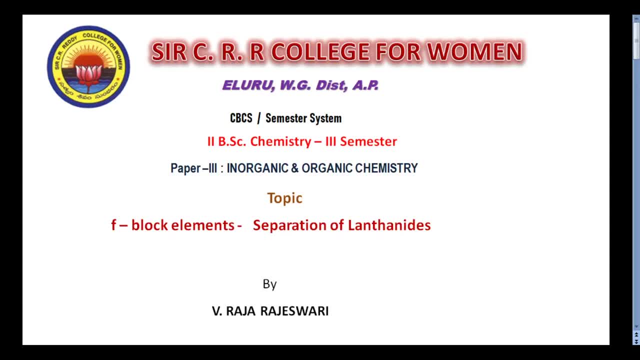 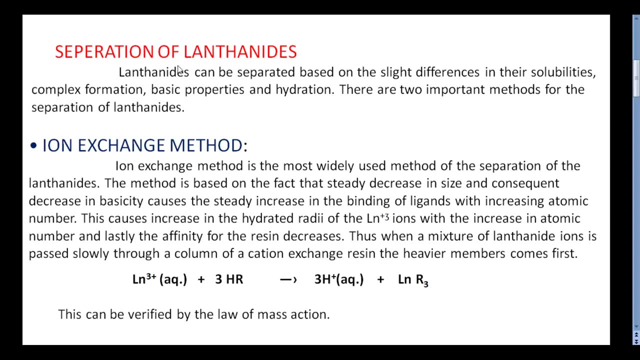 I am Rajaswari, working as a lecturer in chemistry in Sir CRR College for Women, Eluru. In this video we discuss about the separation of lanthanides. Separation of lanthanides. Lanthanides can be separated based on the slight differences in their